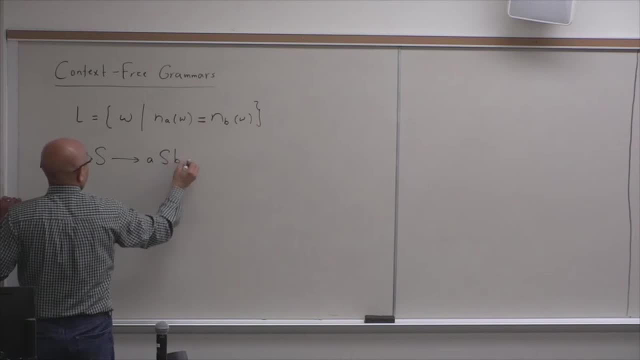 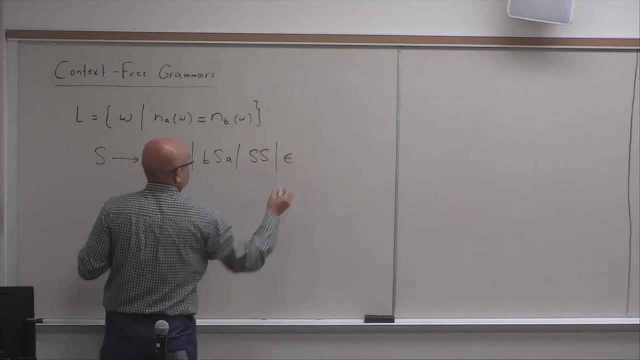 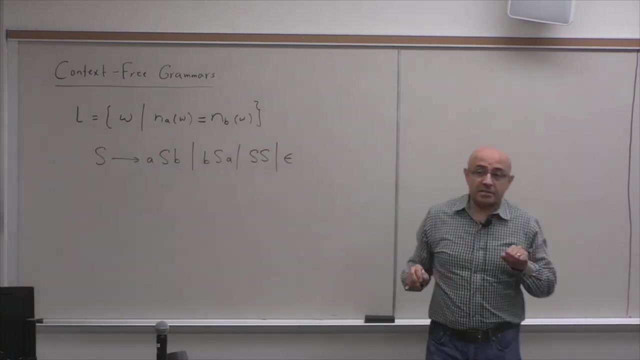 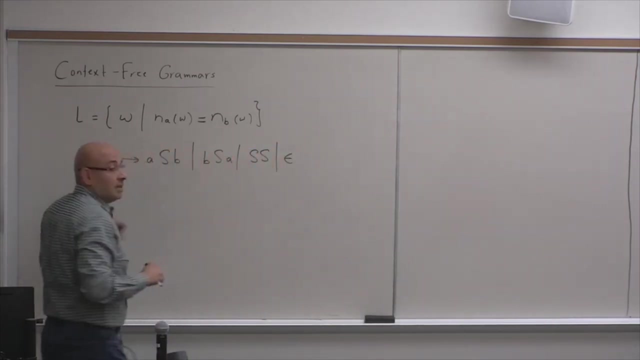 for this language, Or epsilon. Now, in order to show that a grammar indeed generates a language, or that you know the language of this grammar is indeed this language, you need to show that every string generated by G- let's call it grammar G. So this is- let's call this grammar. 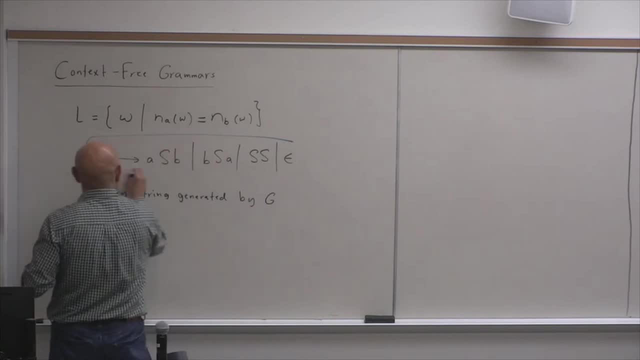 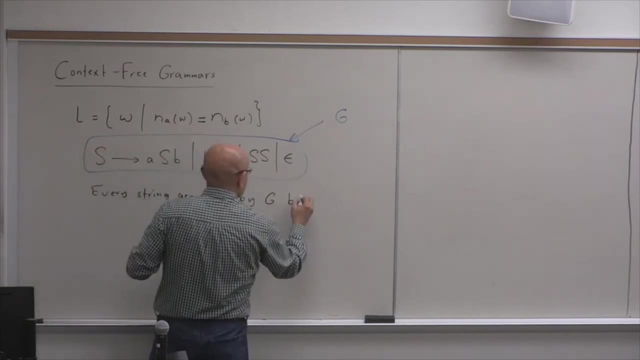 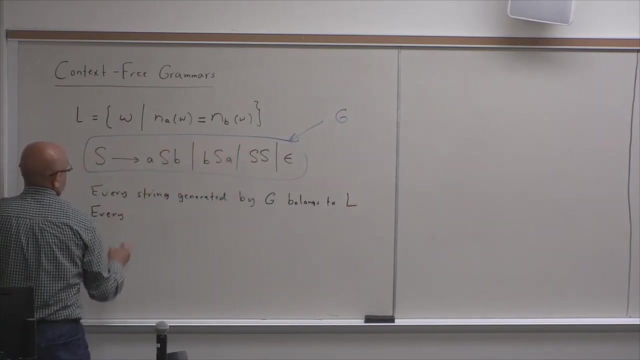 G, grammar G: Every string generated by G belongs to L, and that every what? So, in order to show that this grammar generates the language, we need to show that every string that is generated by G belongs to L. Okay, Okay. 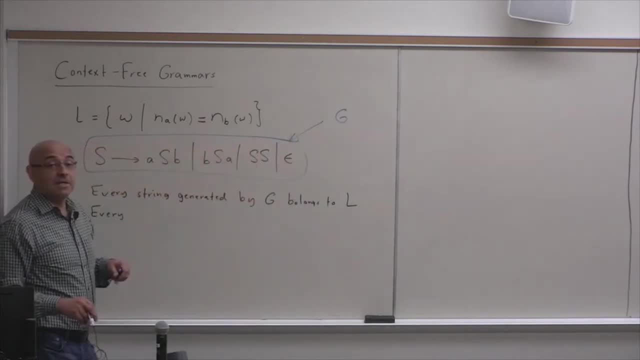 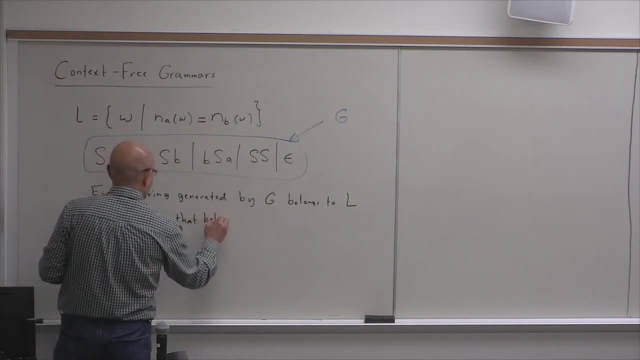 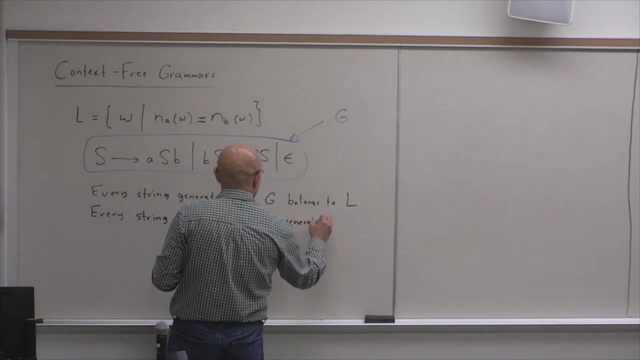 So, in order to show that this grammar generates the language, we need to show that every string that is generated by G belongs to L and that every string that belongs to L is generated by G. Are these the same thing? Two state totally different. 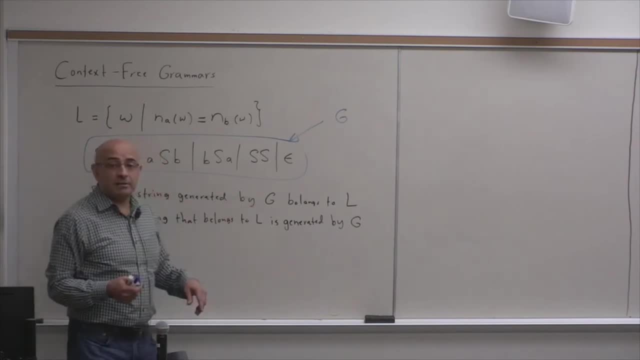 So showing that every string generated by G belongs to L. is it easy or hard? This is very easy. There is no way that you can generate a string here that doesn't have an equal number of A's and B's. There is no way to put more A's than B's or more B's than A's. 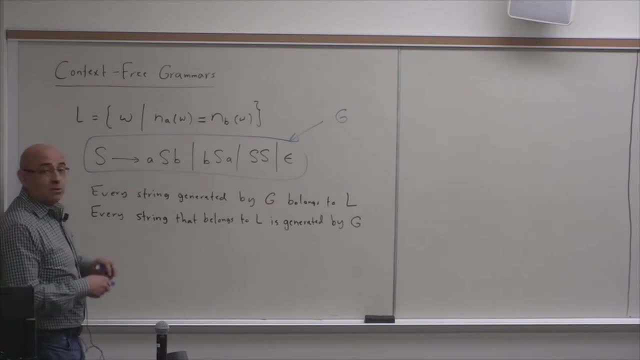 because you will have to use one of these rules. So you have rule one, rule two, rule three, rule four, And none of these rules, you know, can put more A's than B's. So these are the tools that will add A's and B's to the string. 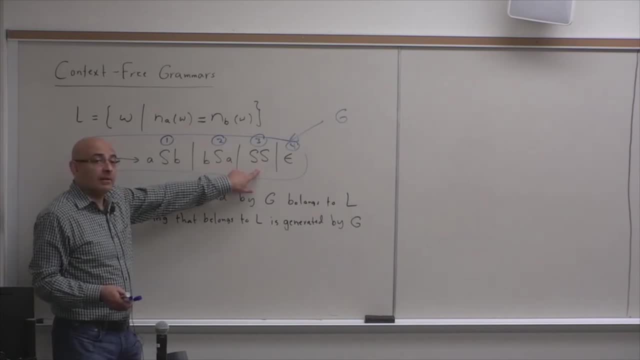 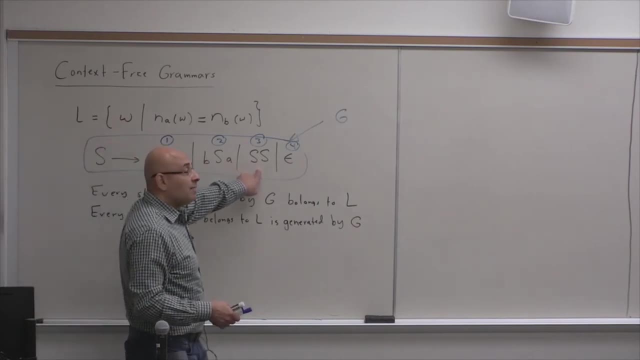 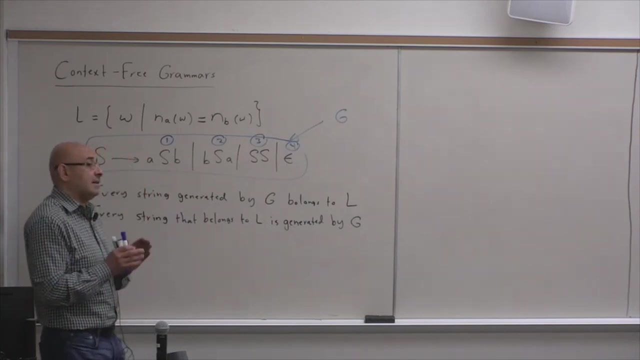 What does this rule do? It makes a branch. What does it do? It splits the path into two branches. Well, in fact, think of it in terms of generation, not in terms of analysis. So you are thinking of it in terms of analyzing a string. 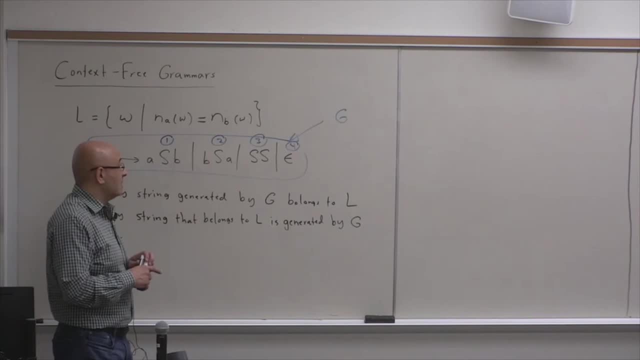 So not analyzing a string. we are generating a string in terms of construction, not analysis In terms of construction. what does this do? Or generation What that It's. so yeah, so what's the relation here between S and S? 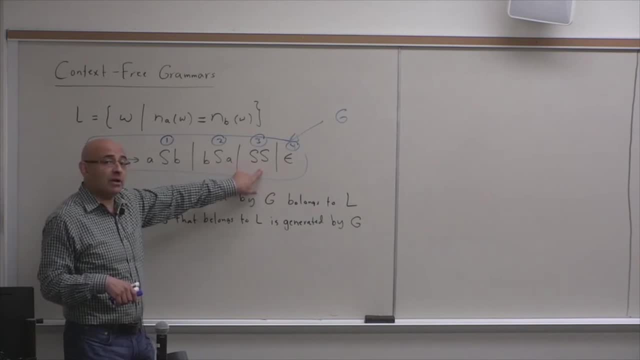 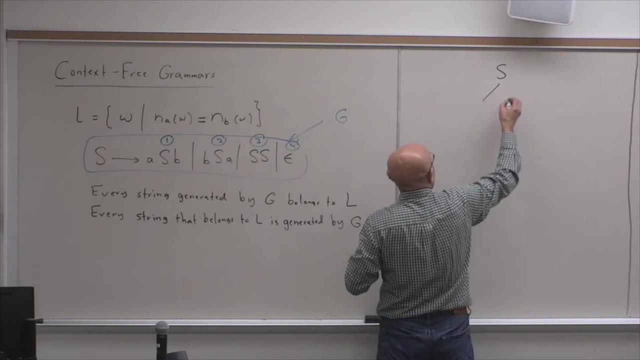 So we're concatenating two strings that belong to the language. So we're concatenating two strings that belong to the. so we're saying that you know this S can be the concatenation of two S's that belong to the language. 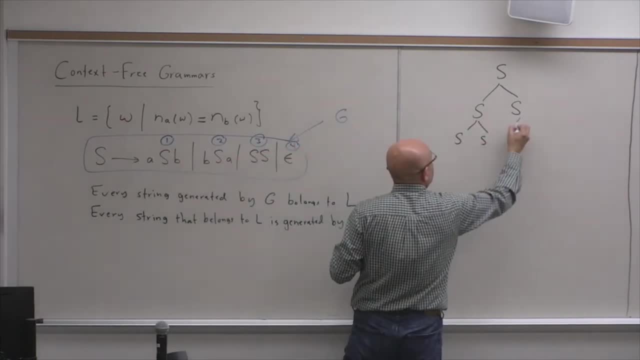 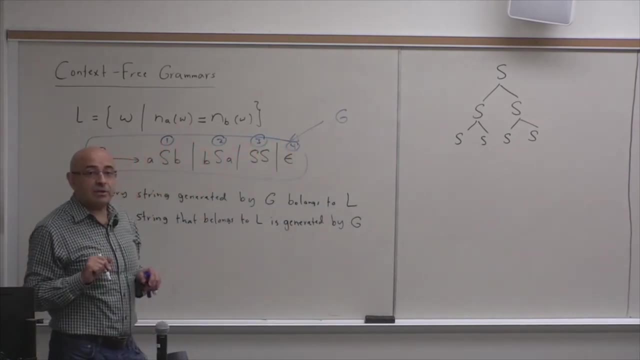 And you know we can keep doing this forever, but obviously this will not generate an actual string. In order to generate an actual string, we will have to use these rules, you know, or if we want to generate the empty string, so we can substitute epsilon for all of them. 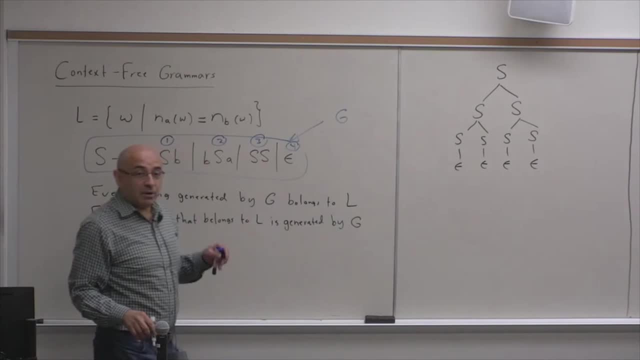 and then we'll get the empty string. But in order to get a string that has A's and B's in it, we'll have to use one of these rules. Okay, So we'll have to use one of these two. So this concatenates two strings that got generated by the 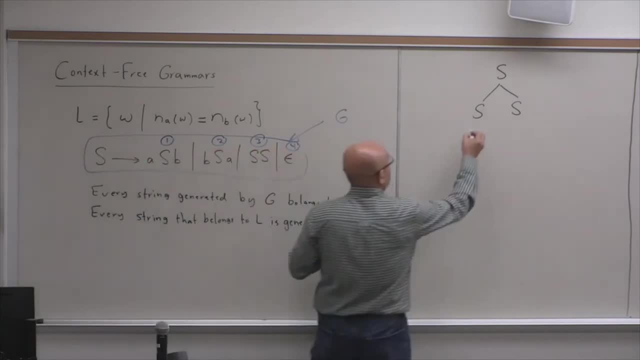 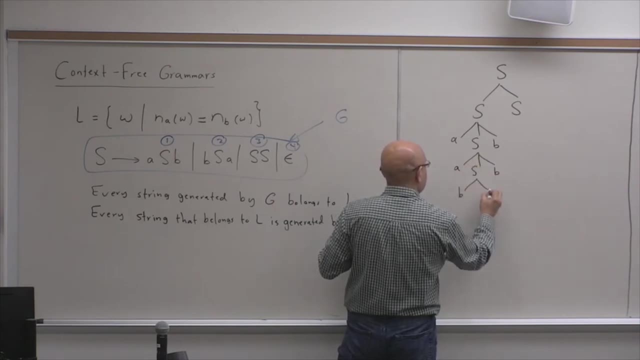 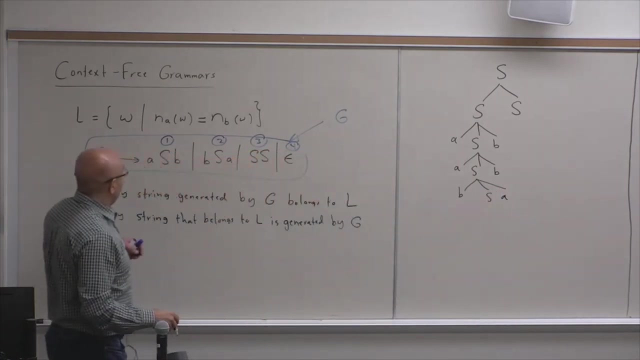 you know, by other rules. So here you know, we can do ASB, we can do ASB again, we can do BSA, and so forth. Now, so it's very obvious that every string generated by this language belongs to L. Now to argue that every string. 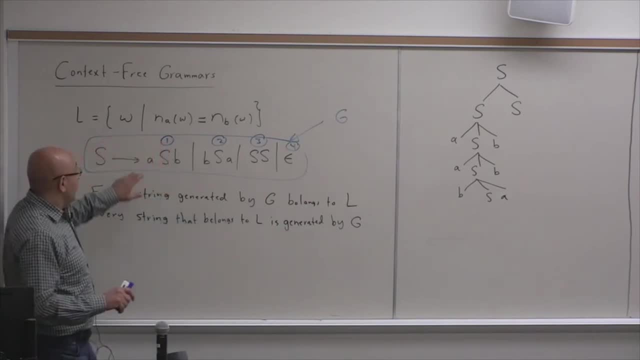 that belongs to L is generated by G, or that this grammar covers all the strings that have an equal number of A's and B's. So did anyone try to come up with a string that has an equal number of A's and B's but cannot be generated using this grammar? 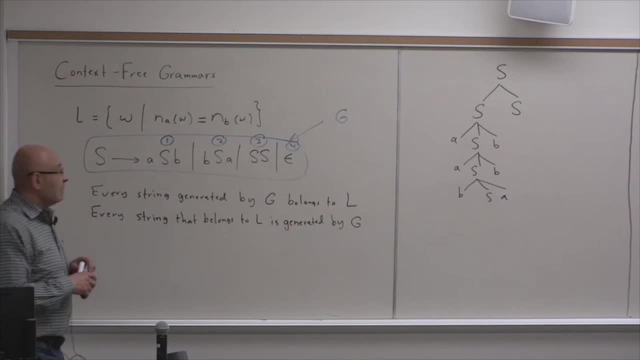 Yeah, In fact we will not give a formal proof for this. We'll just give a, you know, a logical argument, a convincing argument that there is no way or there is no string that belongs to the language that does not get generated. 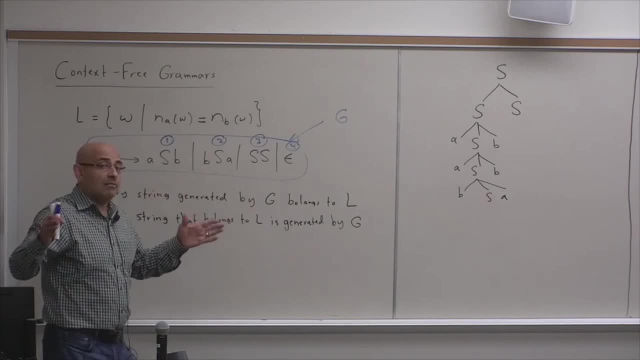 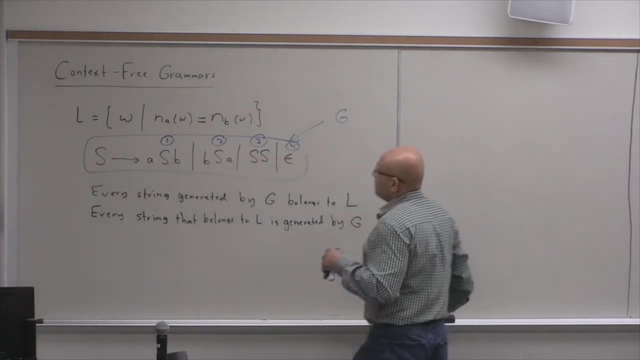 by this grammar, or that this grammar is general enough to cover all the strings that have an equal number of A's and B's. So let's consider the following. you know analysis of the strings that belong to the language. So a string that belongs to the language, you can think of them. 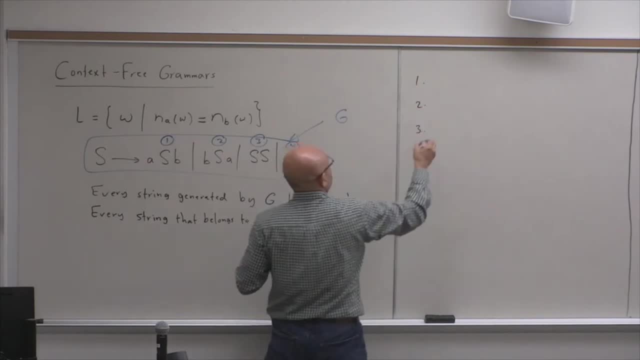 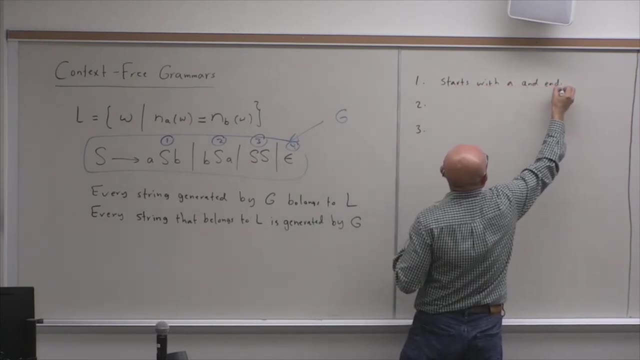 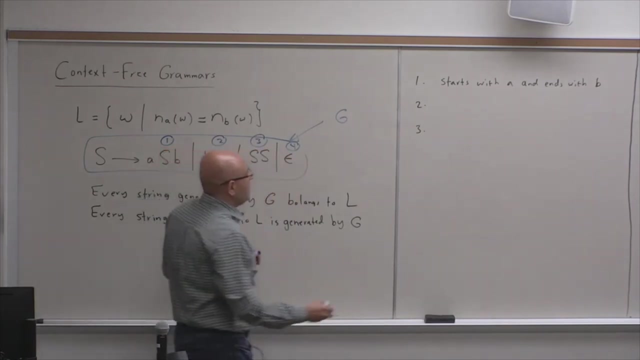 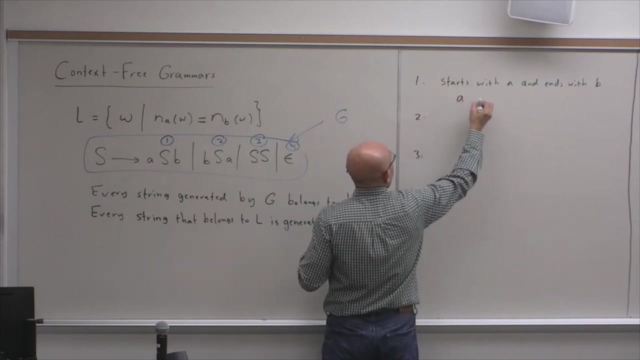 as three kinds of strings. Either starts with A and ends with B, B. So if it starts with A and ends with B, So if it starts with A and ends with B, it ends with B. So what should you have between A and B? 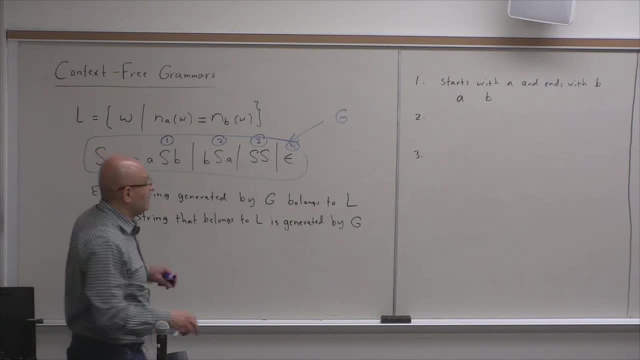 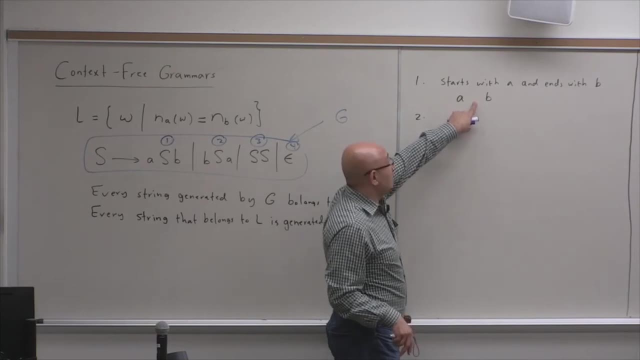 So the string. what can you say about the string or the substring between the A and the B? Epsilon star- Okay, What? what? no, no, you cannot put anything here. What can you say about the W that should be between? 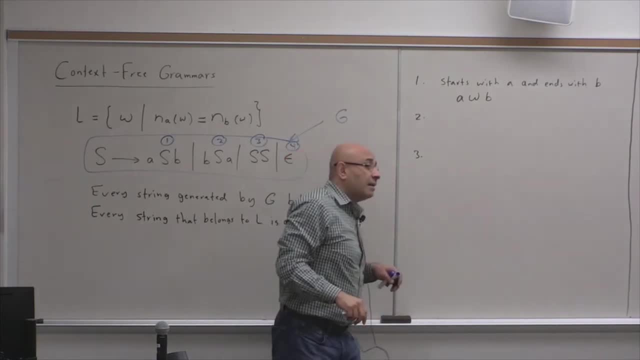 that can be between A and B in this case. Yeah, It also belongs to the language. Yeah, It also belongs to the language. So, in fact, this is- this is, in fact, you know, showing the recursion And this is, in fact, you know, a proof by induction: 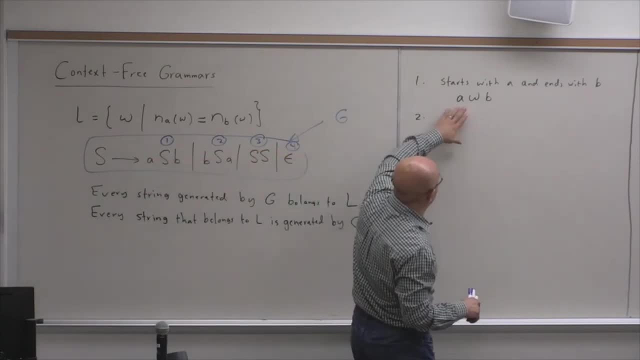 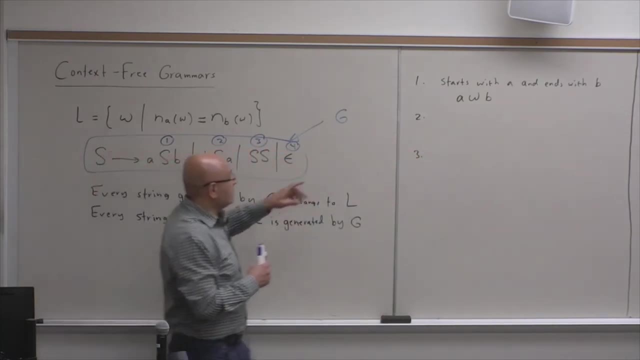 Or you can turn this into a proof by induction that the strings that this will generate, the strings that start with A and B, that start with A and end with B, So everything that starts with A and ends with B should have in the middle. 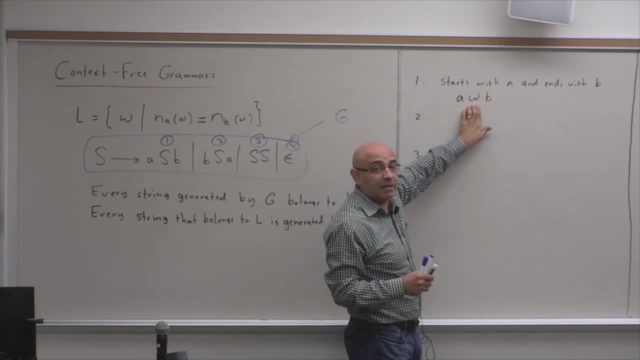 between the A and the B, something that has an equal number of A's and B's, Because here you have one A and one B. If you have something here that has more A's than B's or more B's than A's, the overall string is not belong. 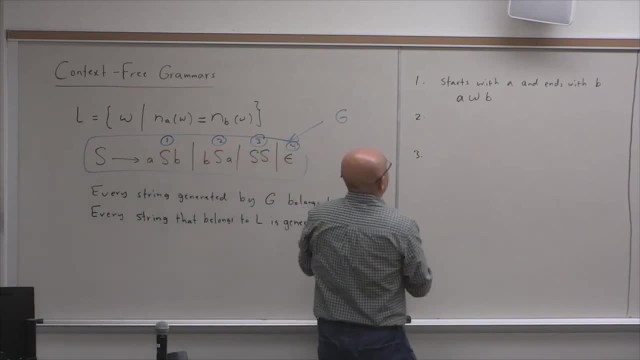 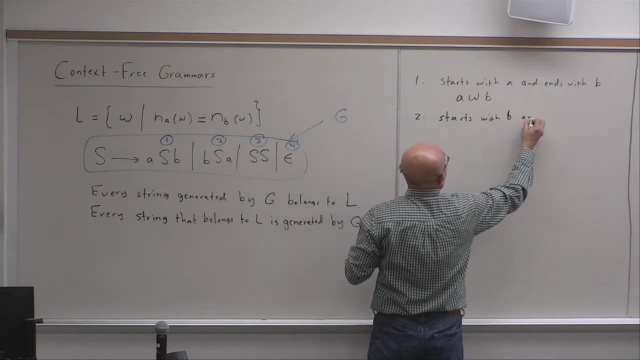 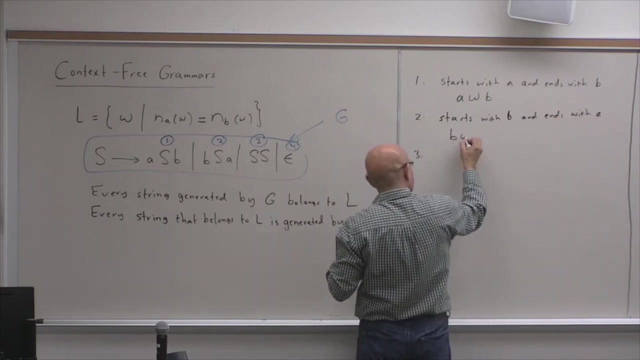 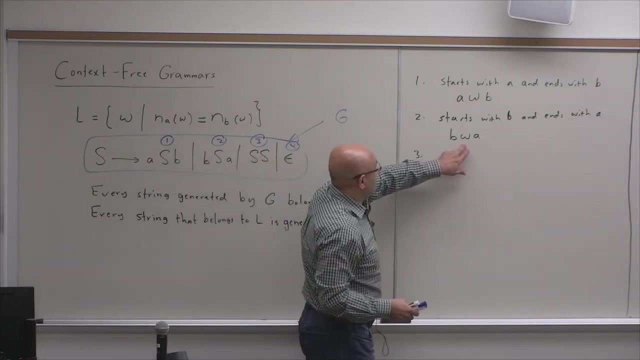 to the language. it's not going to belong to the language. Similarly, if you have a string that starts with B and ends with A, then same logic This should have Okay. Okay, Between the B and the A, it should have a string. 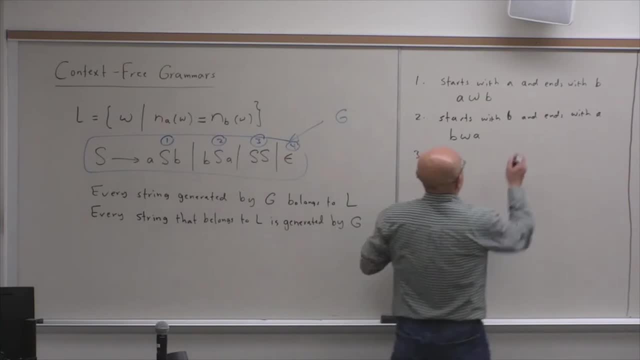 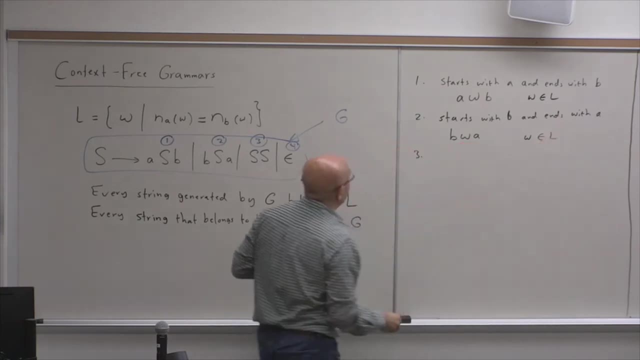 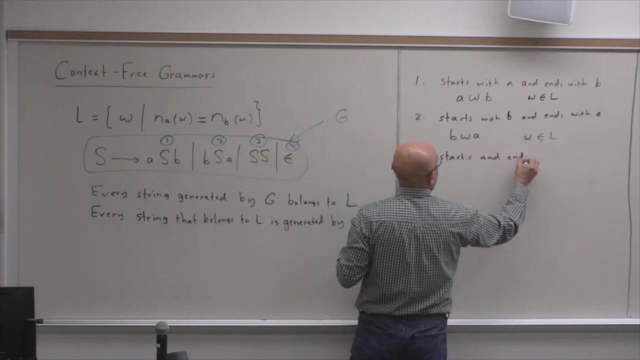 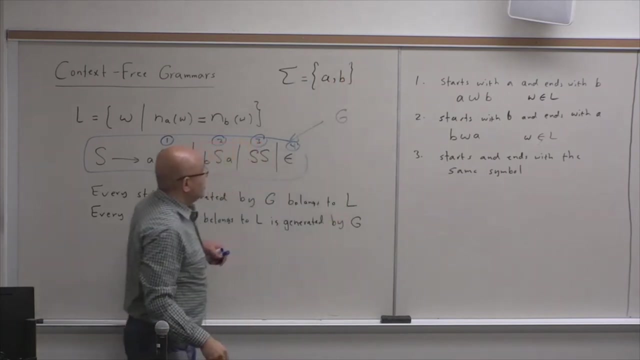 that belongs to the language. So AWB, such that W belongs to L, W belongs to L. Now, what about the string that starts and ends with the same symbol? Okay, Of course, our sigma here is AB, which is obvious. Now, if it starts and ends with the same symbol, 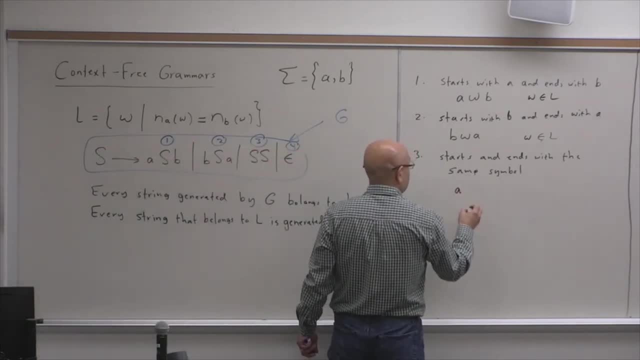 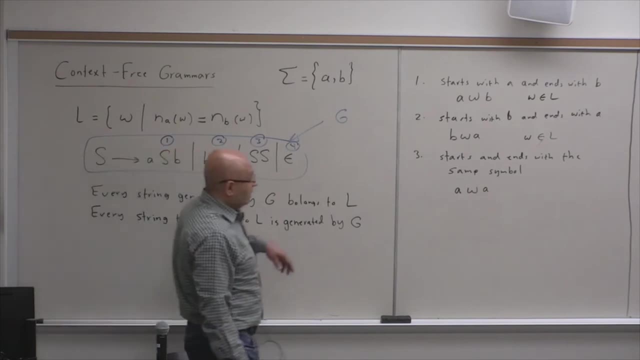 like something. A then WA. Now what can you say about the W between the A and the A? Can you say that this W will have an equal number of A's and B's? Of course not. In fact, this W should have. 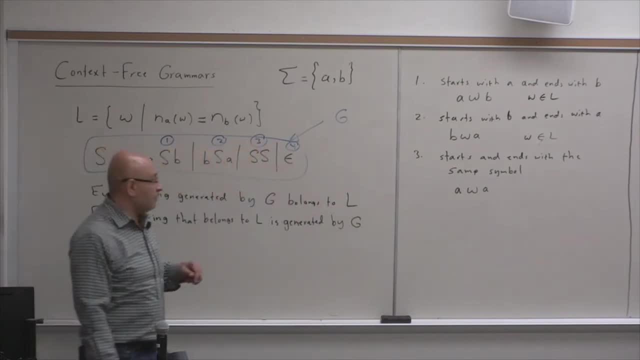 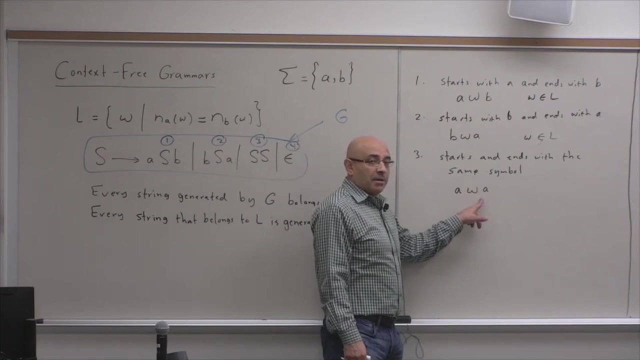 Two more B's, right, In order for this whole string to belong to the language, this W should have two more B's. But in fact, you know how do we justify using this rule. The idea is that any string of this form must be of the form: 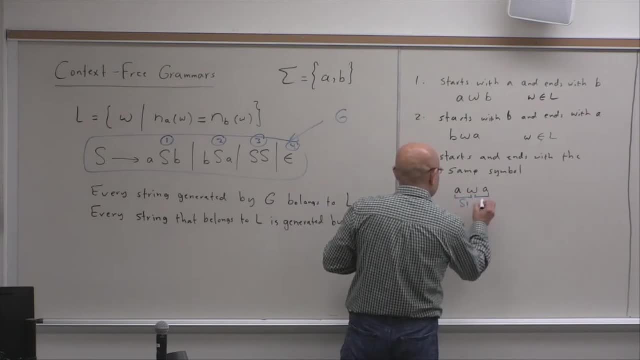 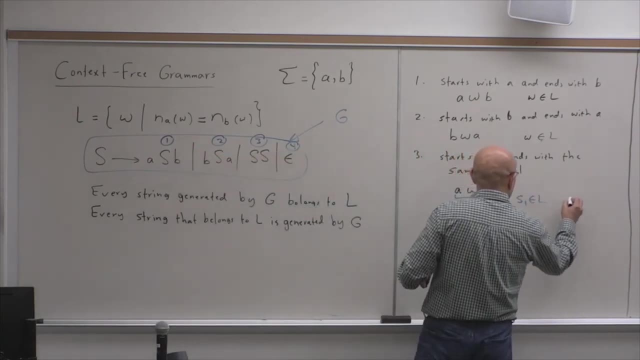 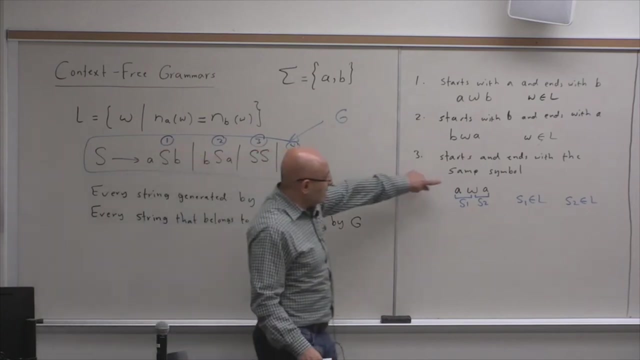 you know S1, S2, such that S1 and S2 belong to the language. S1 and S2 belong to the language. S1 belongs to L and S2 belongs to L. Why So? any string that starts with an A and ends with an A can be split. 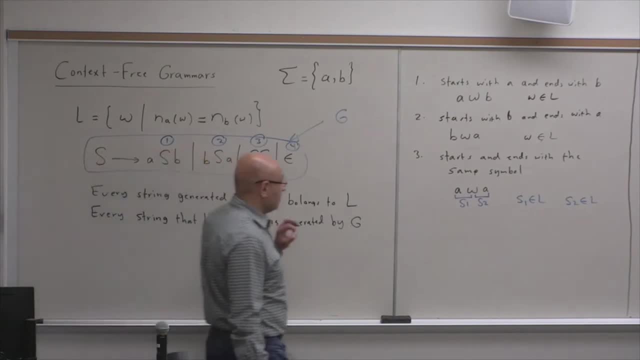 or can be divided, not split, can be divided into two strings, such that you know each one of them has an equal number of A's and B's. Why? Because think about it this way: If let's look at a string, 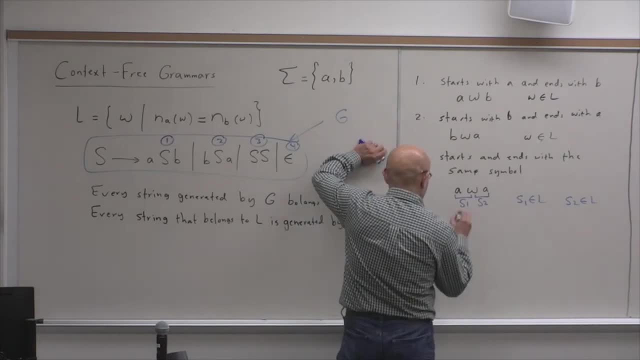 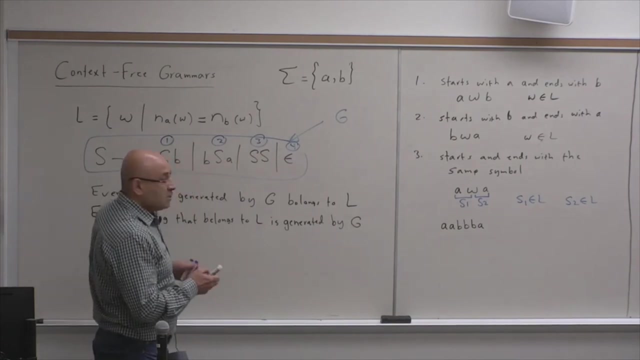 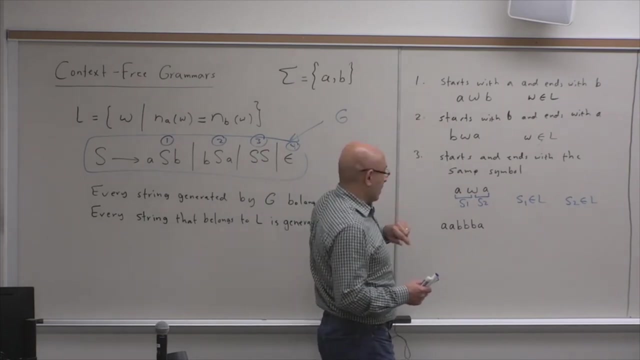 Like you know, a string that starts with an A and ends with an A, So like AABB, AABB, then BA. So this is a string that belongs to the language, but it cannot be generated using this rule or this rule, right. 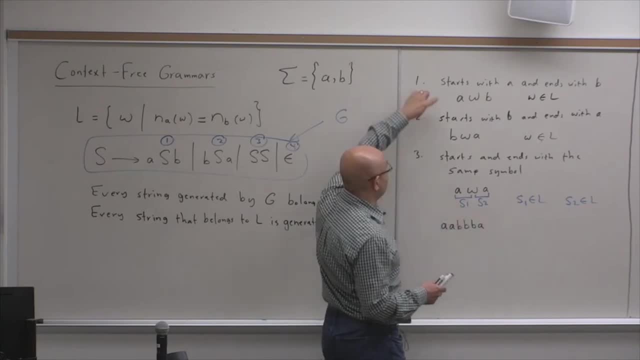 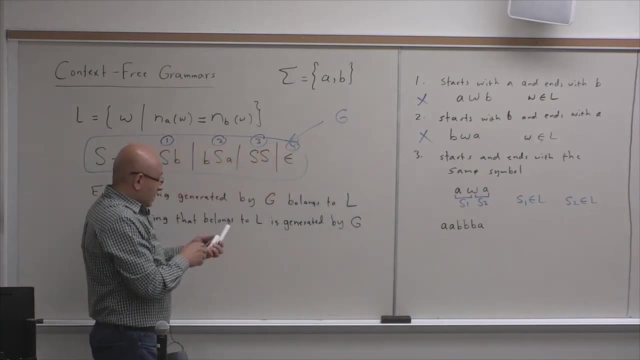 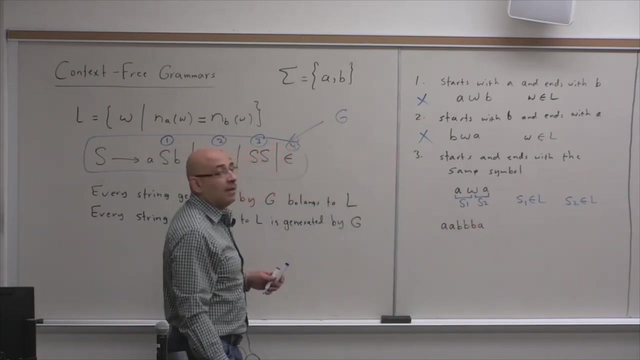 Because it starts with an A and ends with an A. So we cannot generate it using rule one, We cannot generate it using rule two. But if we think of, if we keep the count of A's and the count of B's, or the count of A's, let's say the count. 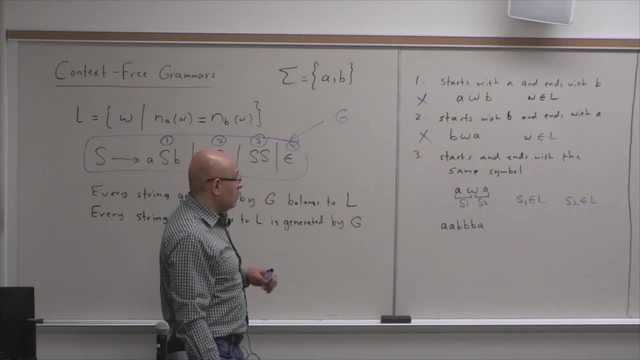 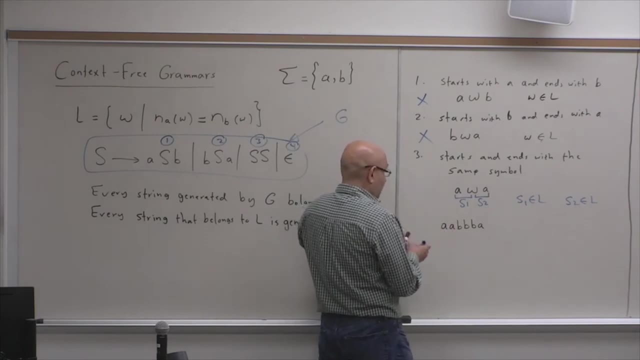 of excessive A's. how many more A's than B's do we have? If we keep counting, we'll say: okay, here I have. this counter is going to say: I have one more A, Now I have two more A's. 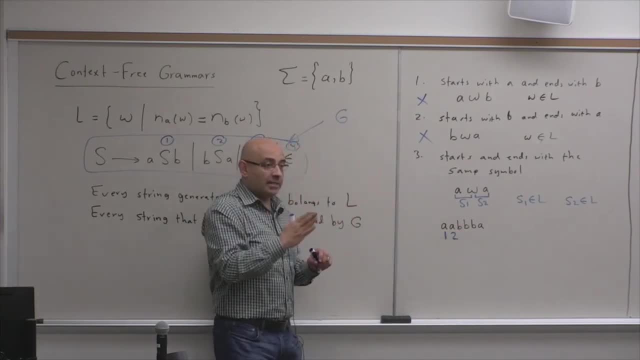 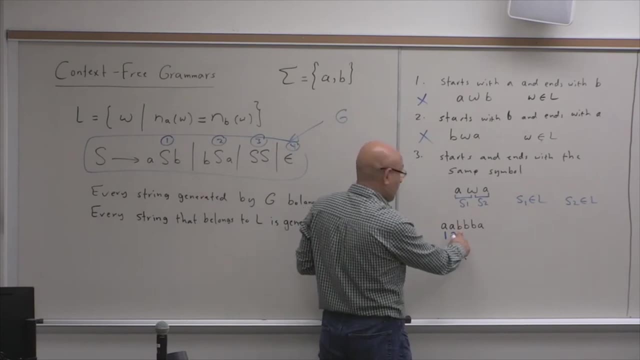 So so far the count is I have two A's but zero B's. So I have two more A's than B's. But now, when I get to this B, what should the counter be? One, Then here, zero. 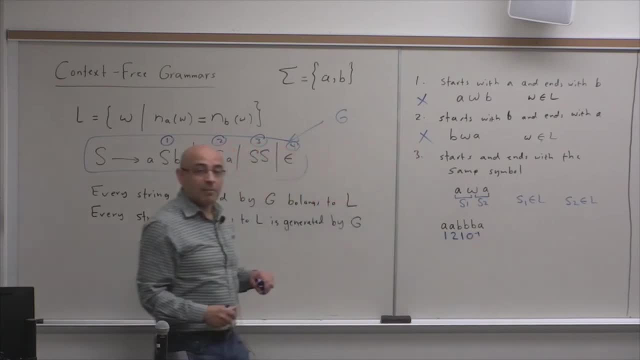 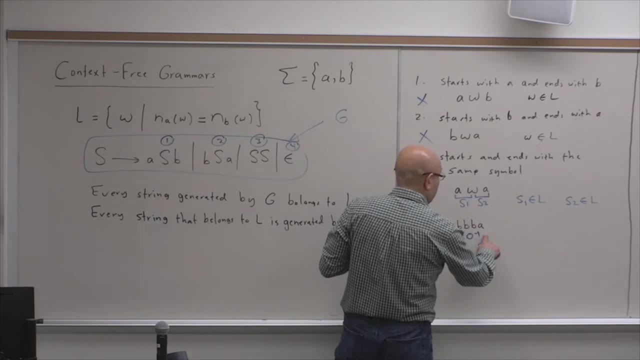 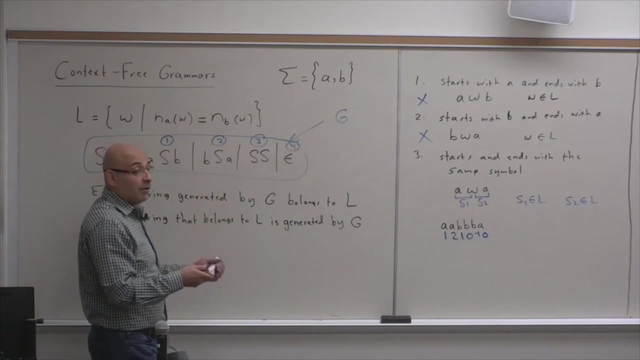 Here it will go to minus one, Because I have now three more, one more B's than A's, And This will bring it to zero. So now, this is for this example. Now, for what does this mean? What does it prove? 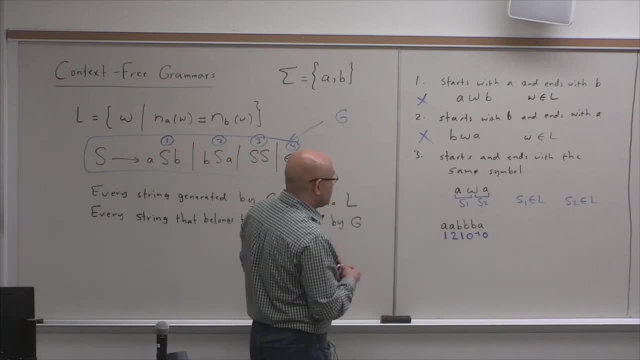 It proves that every string that starts with an A and ends with an A and belongs to the language, can be divided into two strings, that such that each one of them belongs to the language. So Why? Because if you, if you look at a general string, 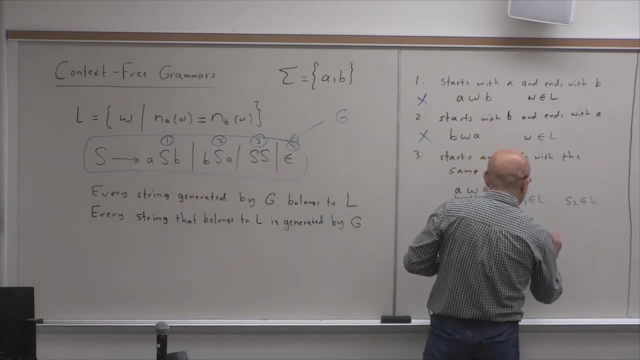 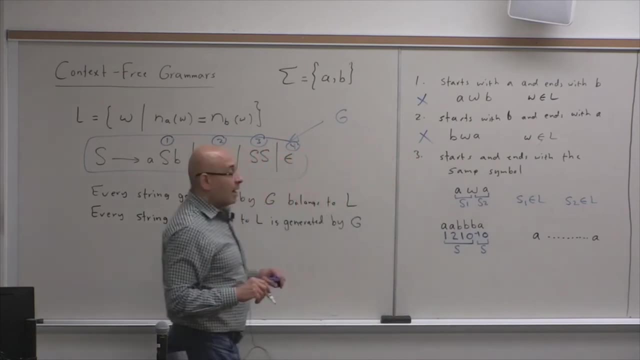 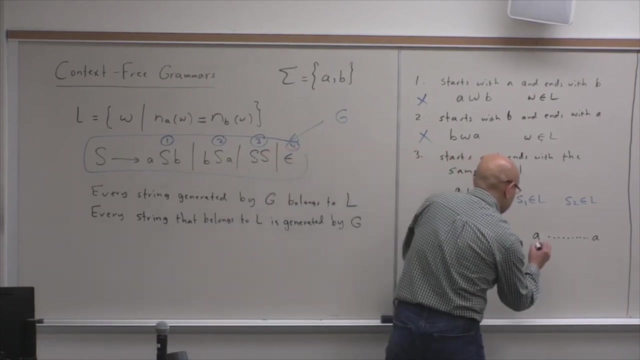 so here I have an A and then I have something and another A. Now I know that you know thinking in those counts. I know that here the count is going to be one, And what must the count be here in order for the string. 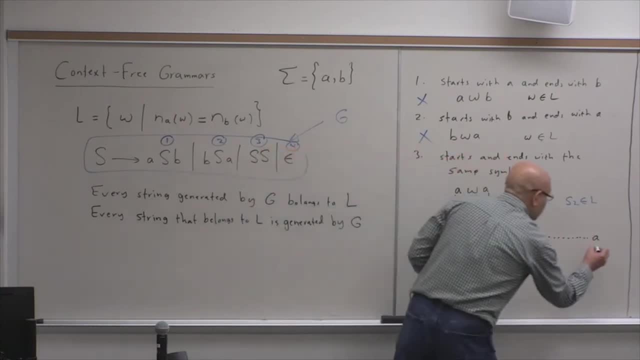 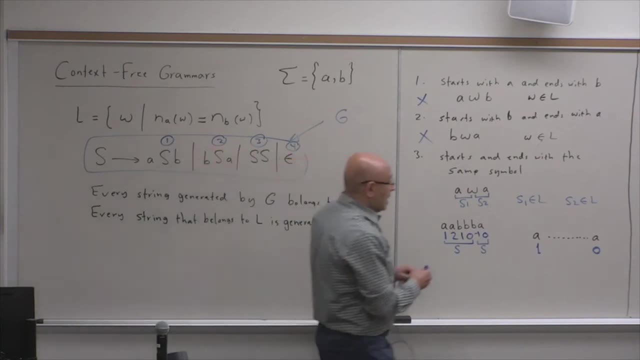 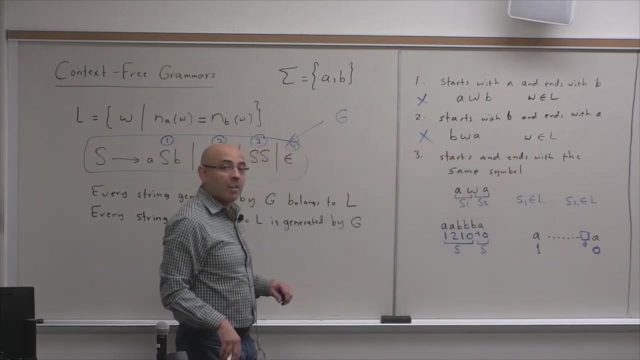 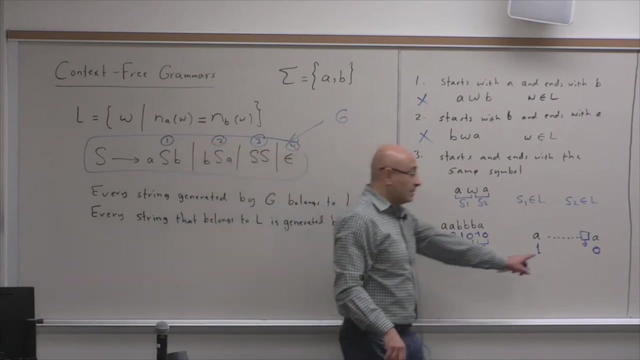 to belong to the language Zero. I know that the count here is zero. Okay, So now this here, in this location. what was the count here? What was the count? It must be. No, there's a unique number. 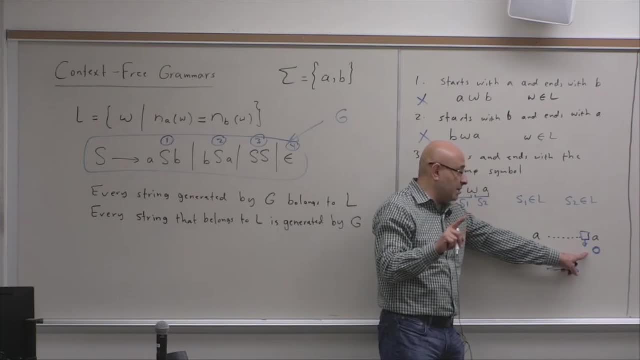 It must be a specific number. What should the count here be before the A? Negative, Negative, Negative: 1.. Why negative 1? Because something, this A added a 1.. So it's like X plus 1 equals 0.. 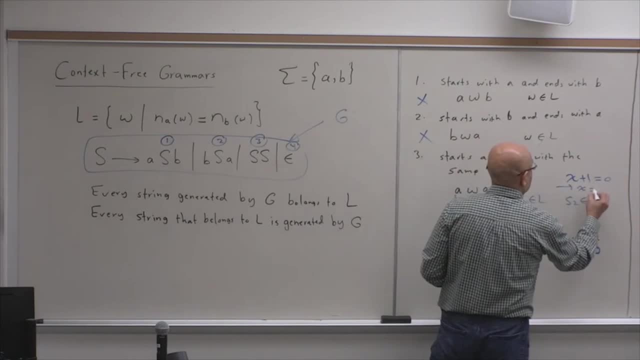 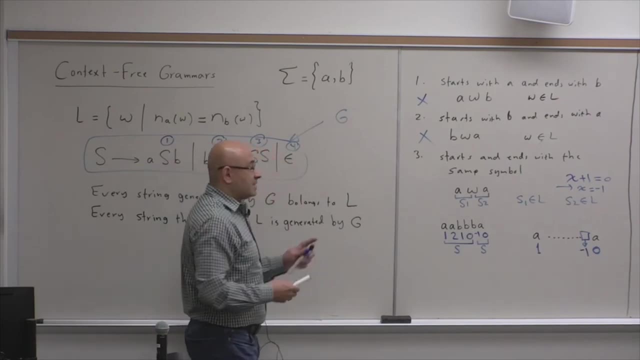 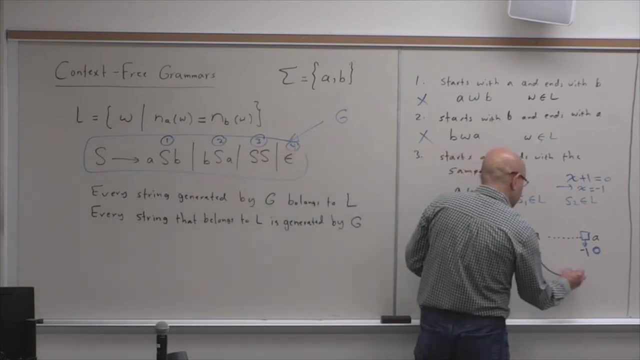 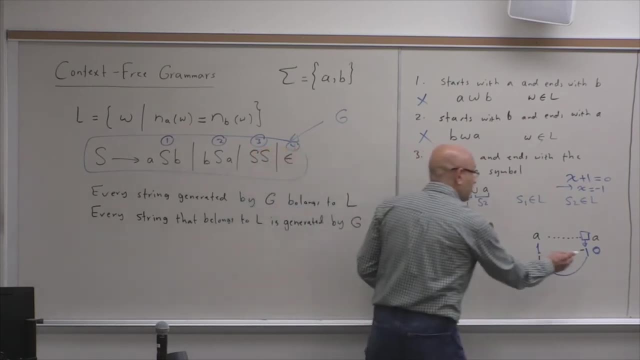 You have this function that goes from 1 and ends at minus 1.. What can you say about this? If it goes from 1 and it ends at minus 1, what can you say will happen somewhere in that, somewhere in the middle? 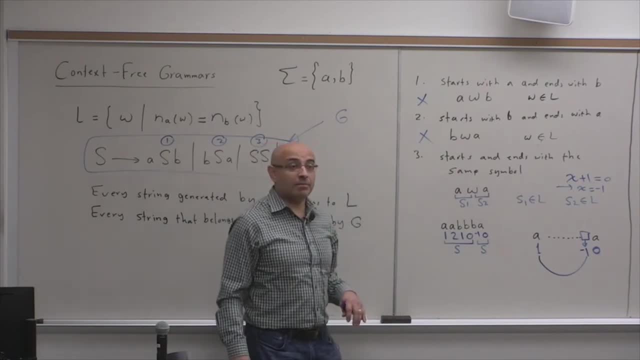 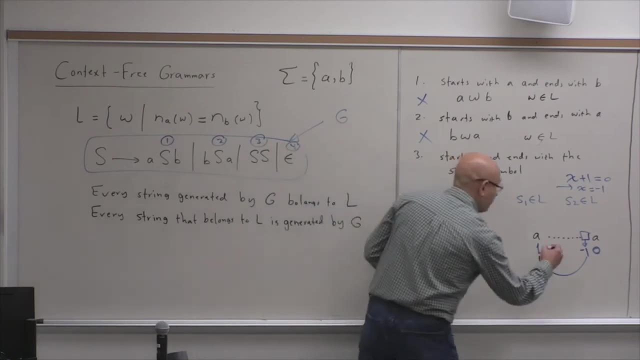 It will reach 0 somewhere It must. there is no way to go from 1 to minus 1 without going through a 0. So there has to be a 0 somewhere, We don't know where. It doesn't have to be in the middle. 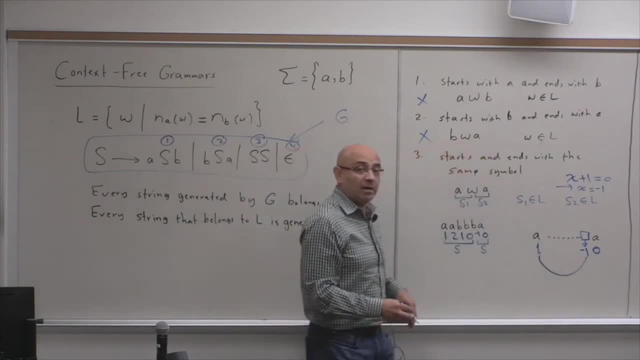 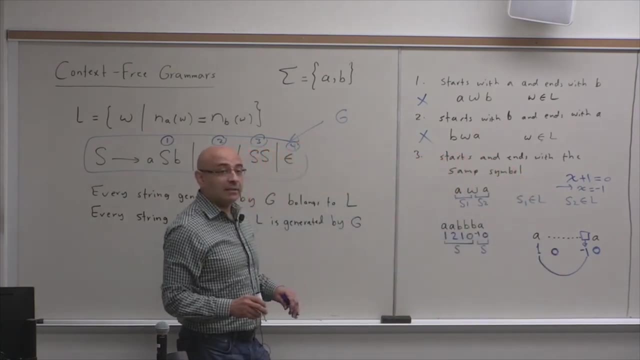 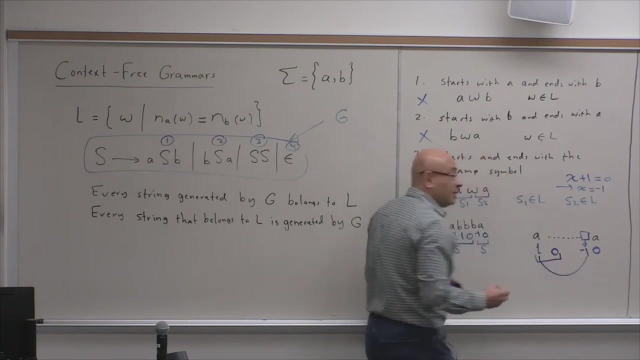 It could be closer to the minus 1.. It could be closer to the 1.. But there has to be a 0 somewhere. And what does this 0 tell us? It tells us that this string must consist of two strings. So whenever we get a 0, we have a string. 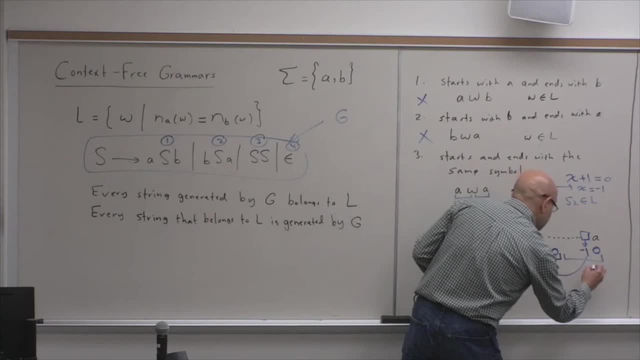 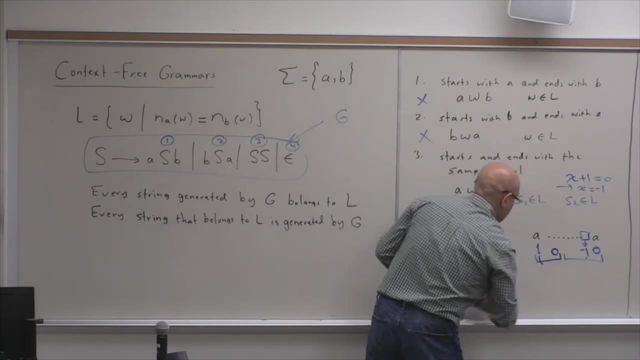 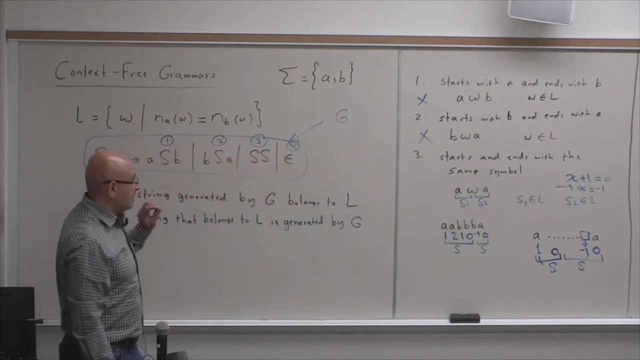 that belongs to the language. So the other 0 will give us another string that belongs to the language. So, Okay, So this argument just shows that you know the logic behind this rule SS, so that to cover all the strings. 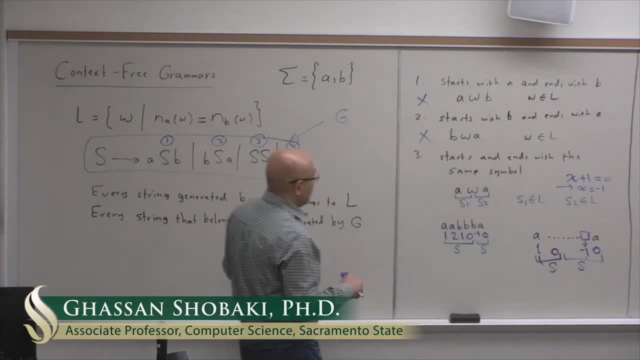 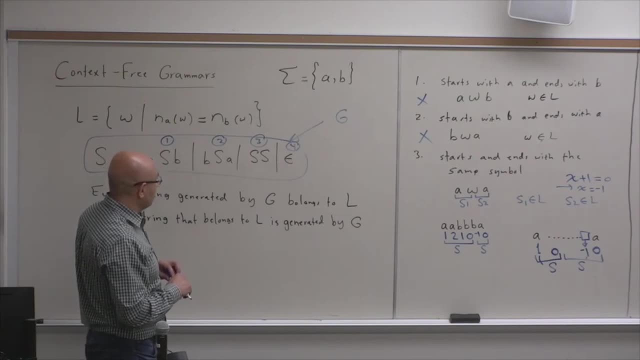 that start and end with the same symbol And in fact it doesn't only cover all the strings that you know start and end with the same symbol. It just it allows you to concatenate strings that that come from the same string. 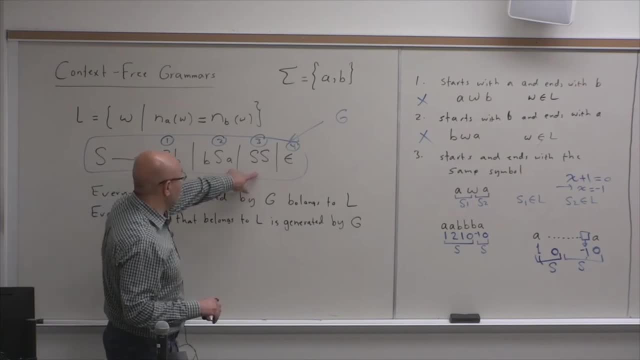 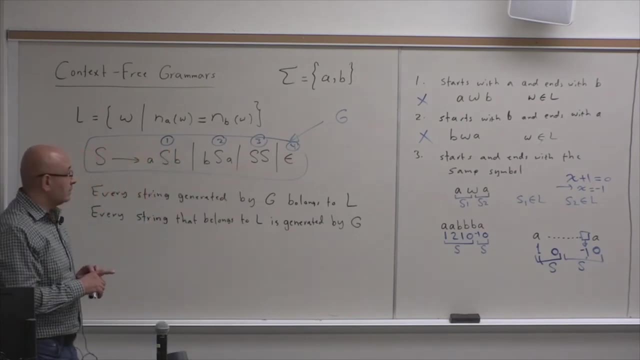 Okay, Okay, Okay, So you can concatenate strings that come from this rule or this rule, Or, in fact, you can. it can concatenate strings that that come from this rule as well. Okay, So this is not a formal proof. 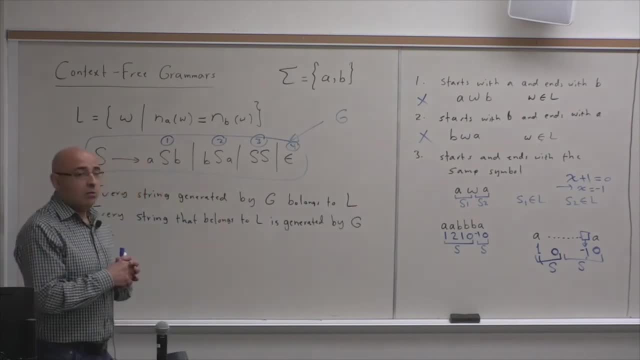 But it should be. it should convince you that we are covering all the strings that belong to the language And try to come up with a string that we cannot derive. Yes, So if you have epsilon, would you have to number epsilon 2? 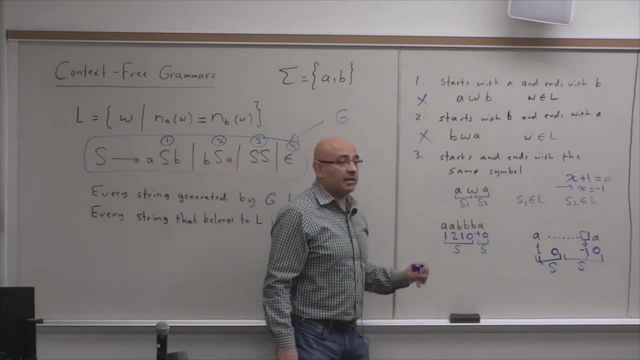 or Yeah, There would be no epsilon in an actual string, right? An actual string will not have an epsilon in it. Epsilon by itself is a string that does not have any symbols in it. So basically, with an epsilon, we start with 0 and end with 0. 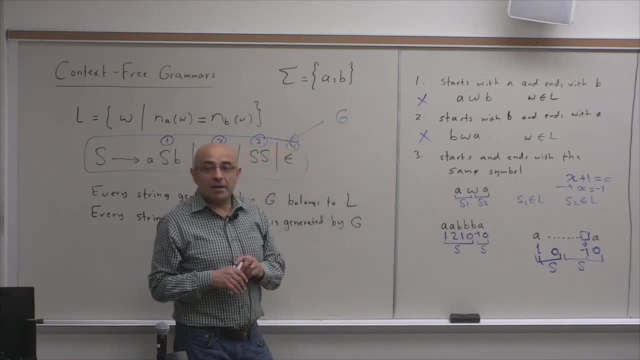 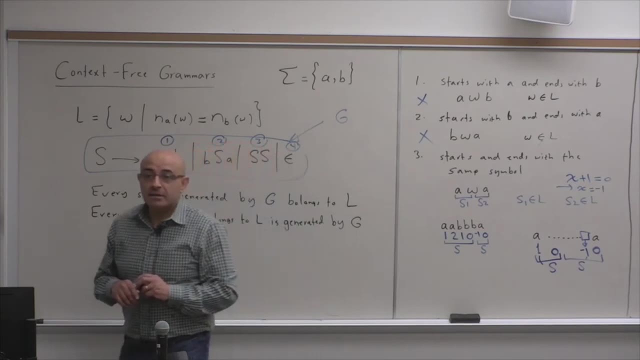 And it will never go to 1 or minus 1.. So the epsilon. so it cannot have. the epsilon is not a symbol that can appear within a string. The epsilon is a symbol that represents the empty string, So it doesn't have any symbols. 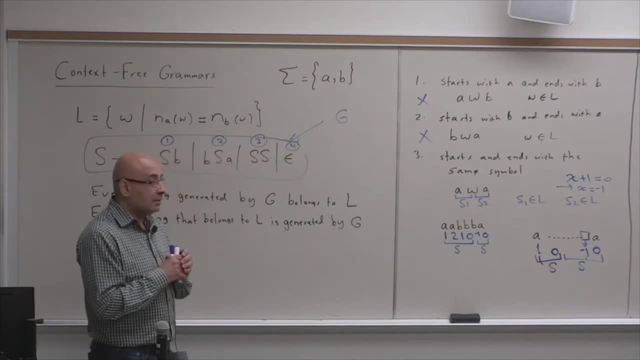 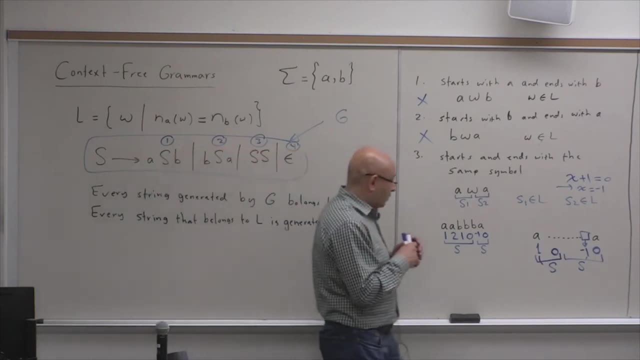 Yes, Is there more like the thing 0's in between Right? Yes, so this that's a good point. So what we have argued shows that there should be at least one 0, but there can be multiple 0's. 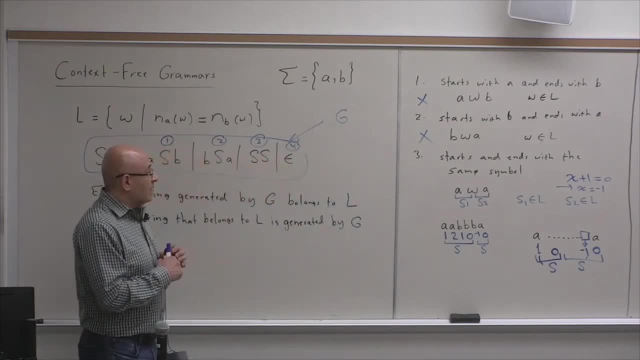 Yeah, So that's a good point. Okay, So you know this string here. There is more that we would like to say about this grammar. So there are. well, first of all, with this grammar, there can be multiple ways of deriving the same string. 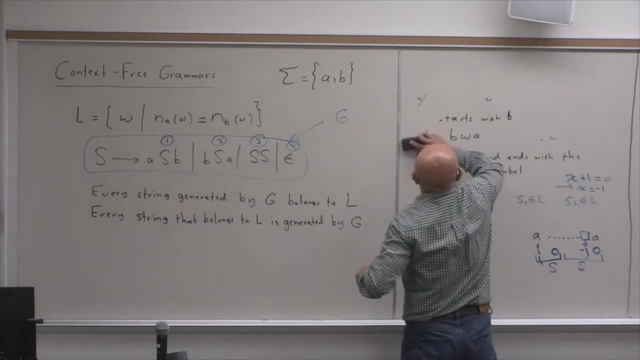 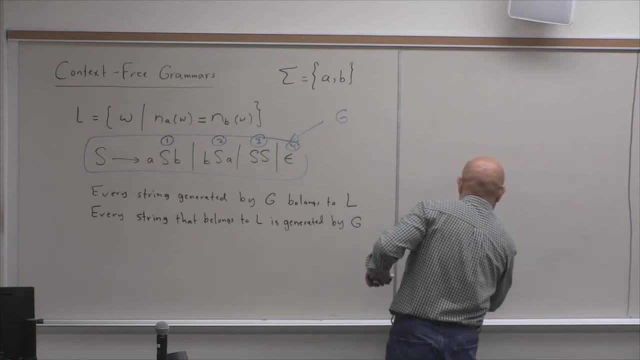 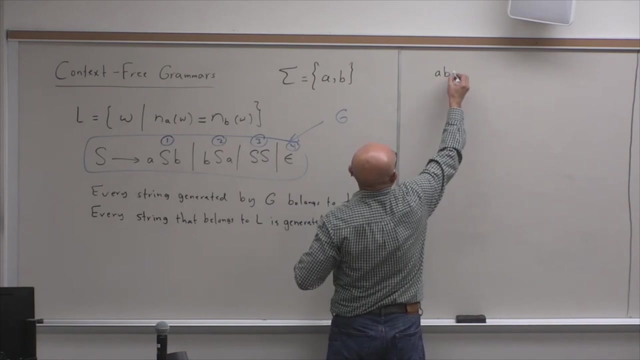 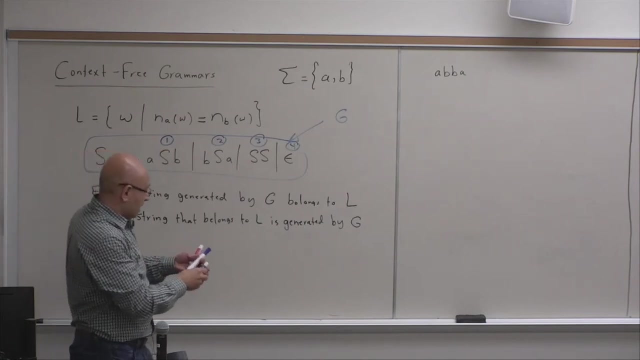 So, like you know, the string say a, b, b, a. So you can derive this in two different ways. I can show you two different derivations of this. One derivation is that it's an s and a. 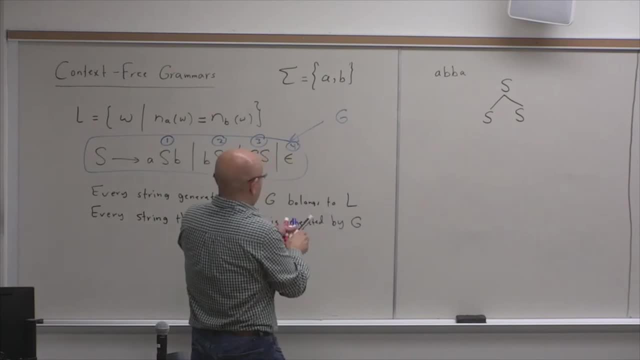 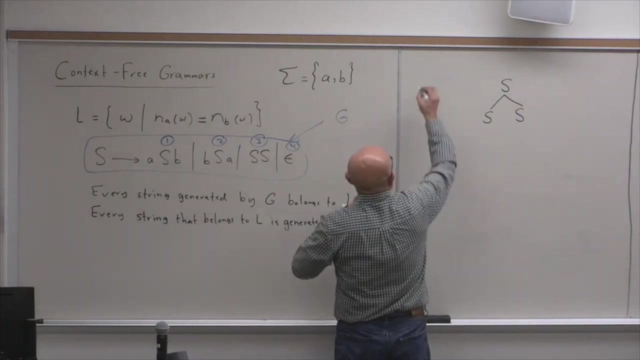 And an s, where you know, this is the first s and this is the other s. Or let's make it more interesting. A more interesting example, The one that I just had: a, b, b, sorry, a, a, b, b, b, a, b a. 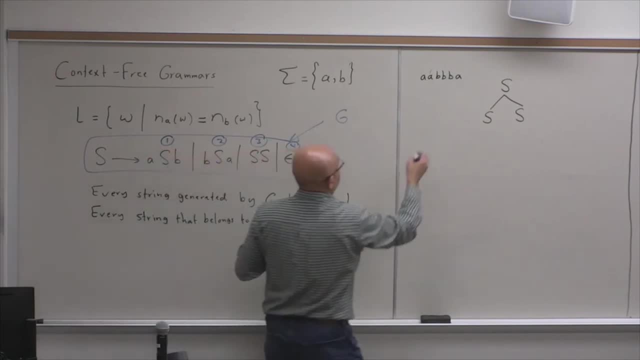 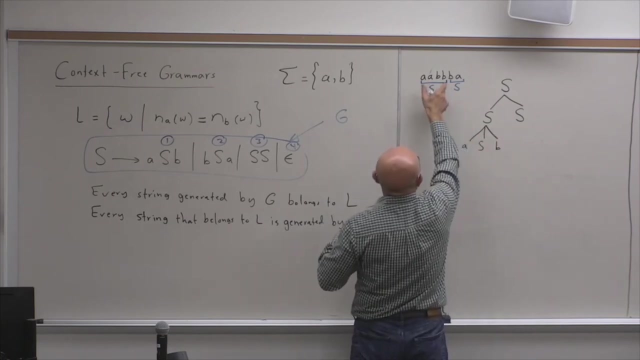 This one, So this one will. I don't know, I don't know, I don't know, But you can view it as this is an s and this is another s And you can derive it. So this is going to be a s b And then, yeah, a s b. 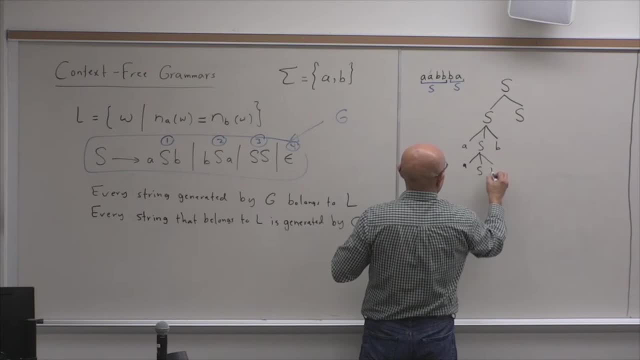 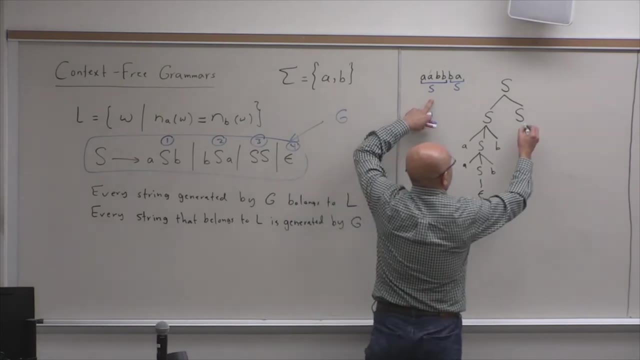 And then another a, s, b, And then I put an epsilon. So this way I derive this left-hand side s And for this the other s I do b, B, S, A, and then I put an epsilon. 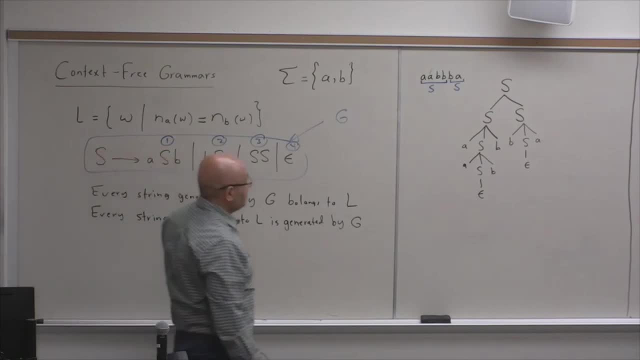 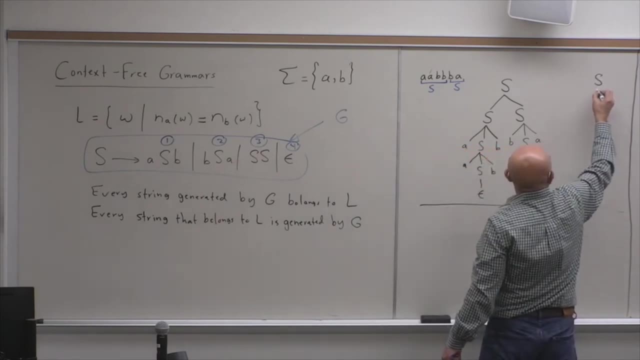 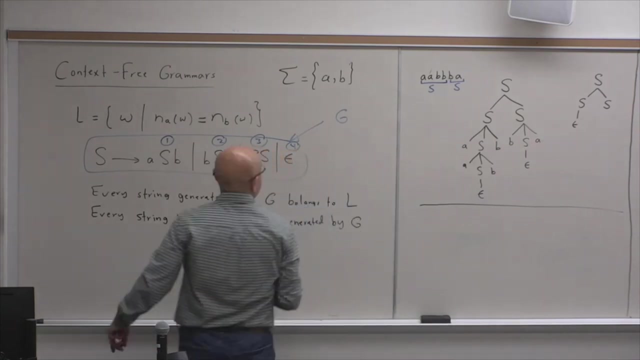 So this is one derivation, but I can derive it this way. instead. I can say: okay, S is SS, but I can set this S to epsilon. I can substitute epsilon for this, And then this S will have the actual string. 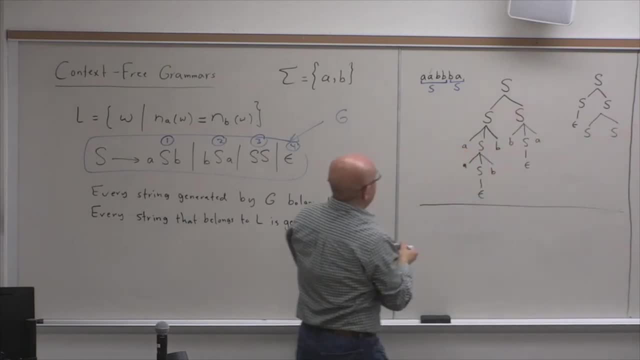 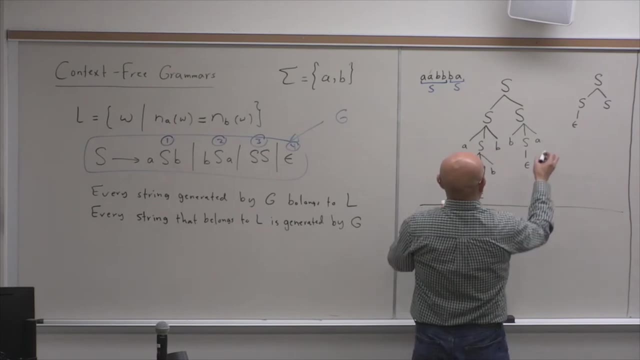 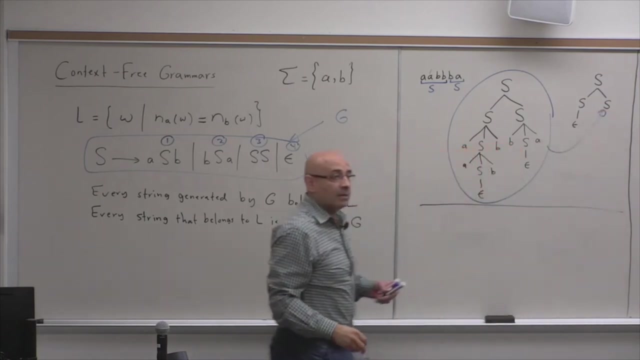 So this will be an SS And this will be just. you know this, I'm not going to repeat it. So this S is going to be this whole thing, Right? So you can say: this is I can set, this is just another alternative. 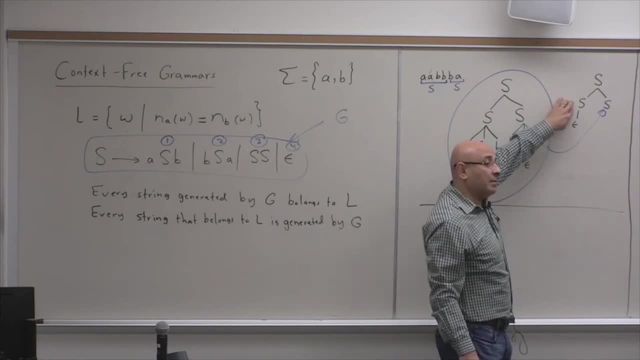 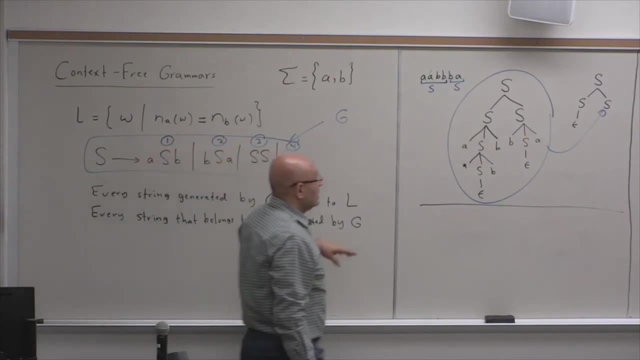 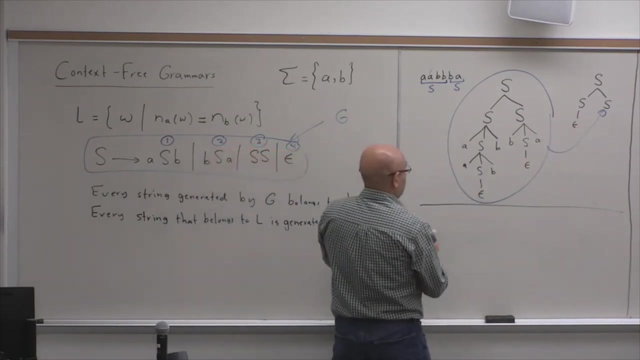 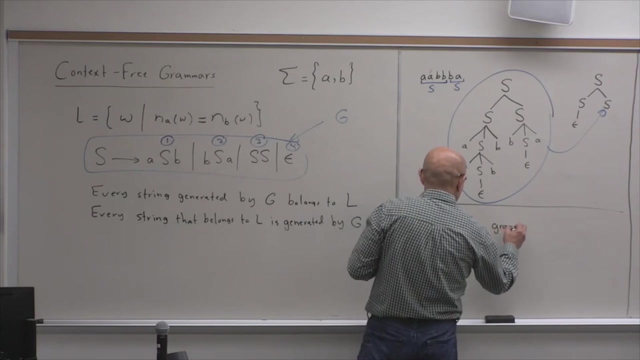 So what am I trying to show here? That there can be multiple derivations for the same string, And when there are multiple derivations for the same string, we call this grammar an ambiguous grammar. So this is an ambiguous grammar, Okay, So an ambiguous grammar. 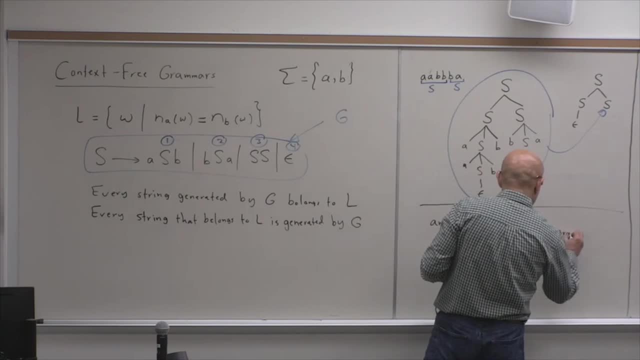 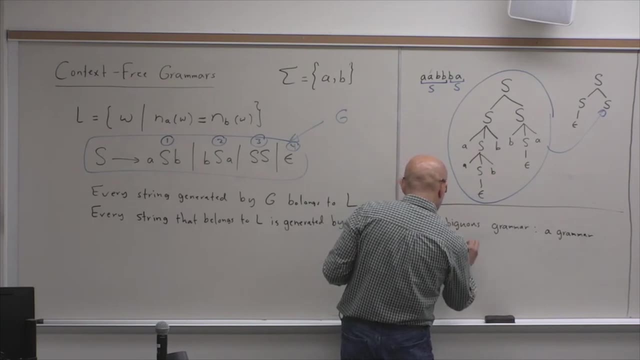 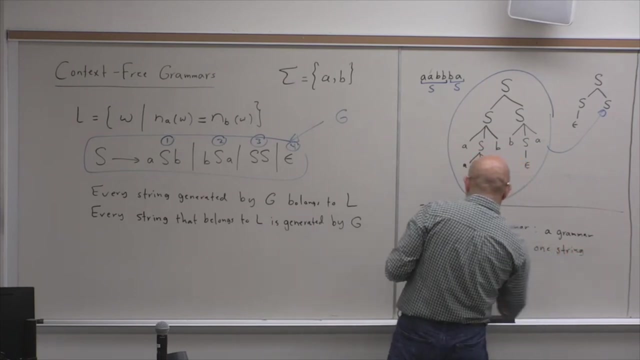 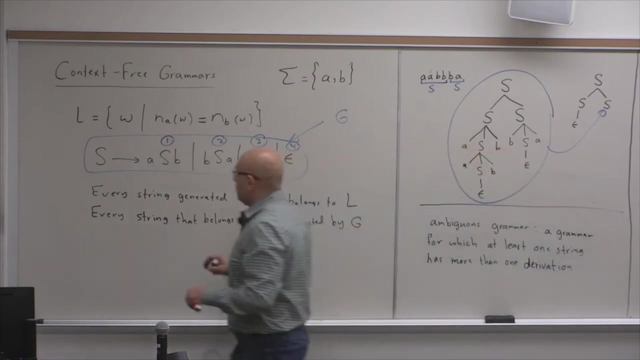 A grammar For which at least one string has more than one derivation. And speaking of derivations, there's a very interesting thing. There's a very interesting thing. There's a very interesting thing We have: we should be aware of the notion of leftmost derivation. 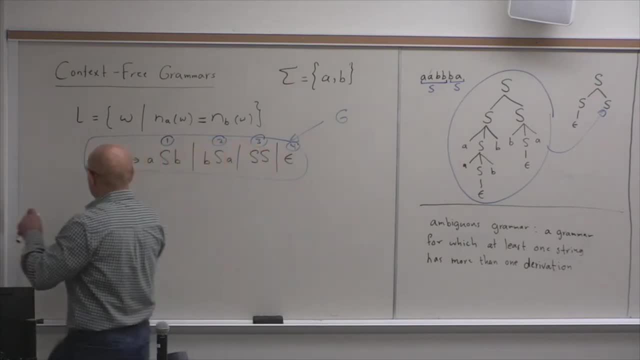 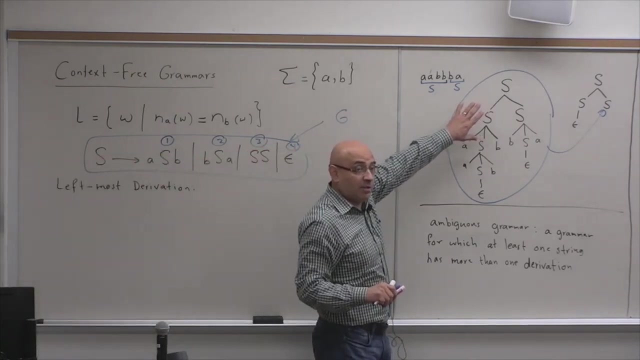 and rightmost derivation, Leftmost Now leftmost derivations and rightmost derivations. Okay, So for any derivation that you can do with a tree, with a derivation, you can do it with a tree, With a derivation tree, you can do it in a leftmost manner. 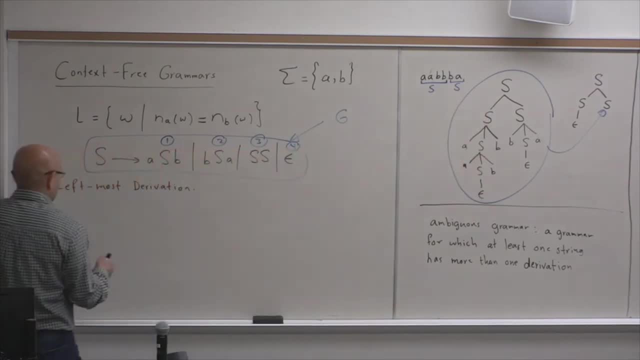 or a rightmost manner using the textual derivation. So I will show you the leftmost derivation for this string. So I will start with S, Then I will substitute by rule by, I will substitute by rule 3 and I get an SS. 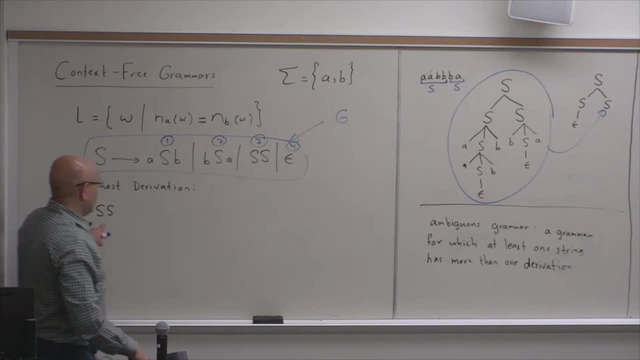 So this is rule 3, gives me SS. Now in a leftmost derivation you always substitute for the leftmost symbol first. So here you substitute for this S, ASB by rule, by rule 1.. I do ASB, then S, Then I substitute. 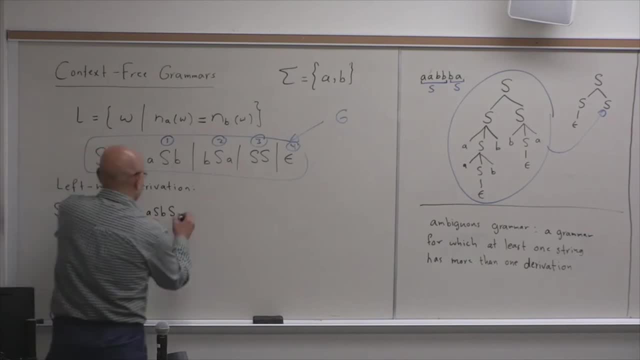 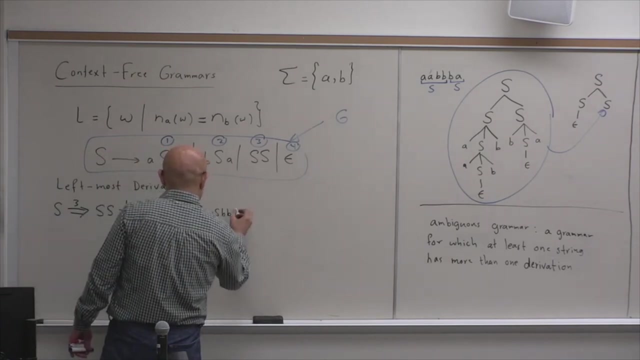 for the leftmost symbol, again by rule 1.. I do ASB A, A, S, B, B, And then I still have the S. Then, with the leftmost logic, what should I substitute Epsilon for the S. So, using rule number 4, I substitute epsilon for the S. 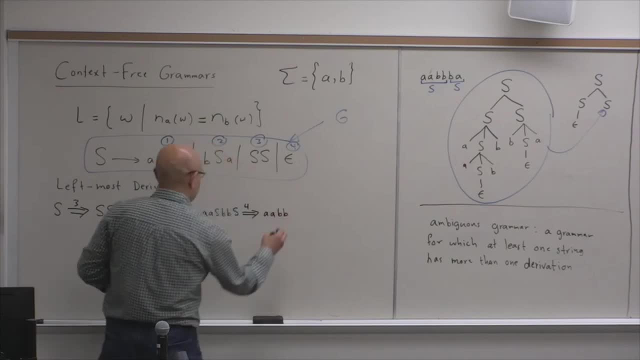 So I will get A, A, B, B, S, Then by rule I substitute for the S, Then I substitute for the S. So now I'm done with the leftmost, with the left-hand branch. So leftmost derivation is going to do the left first. 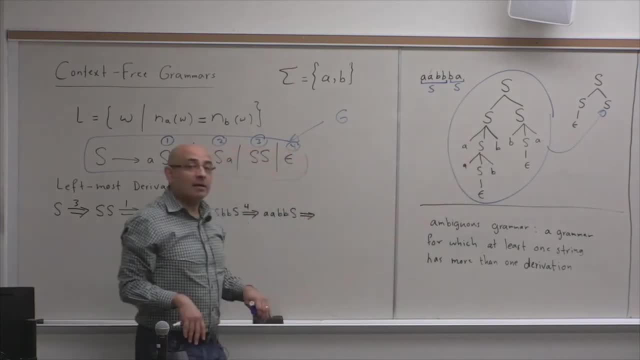 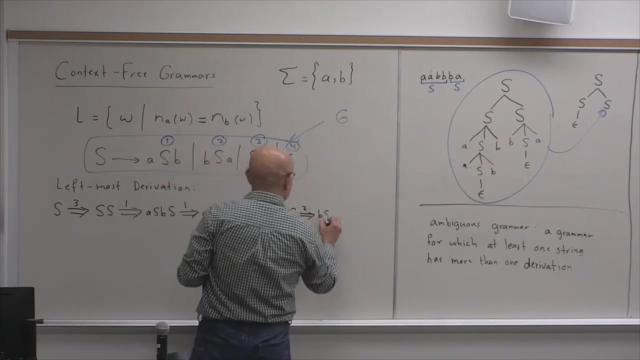 then the right in a depth-first manner, Then I will do this. So this S is this S, This S here is this S. So I'm going to do by rule number 2, I'm going to do B, S, A And then my final substitution: oh sorry, 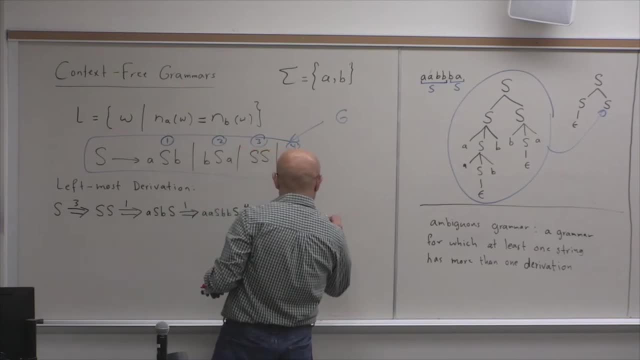 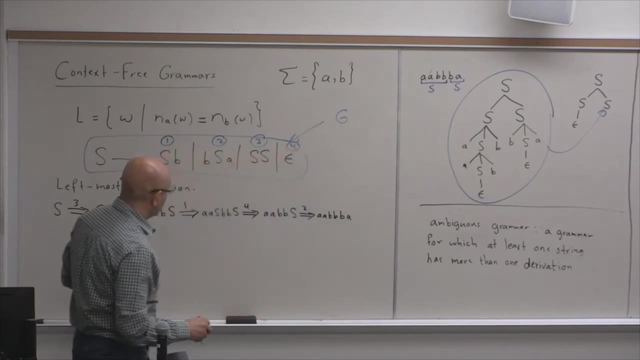 I forgot the rest of the string, So it's: I keep this A A, B, B, And then I substitute for this: S B A B. sorry, B S A. You shouldn't skip any steps. 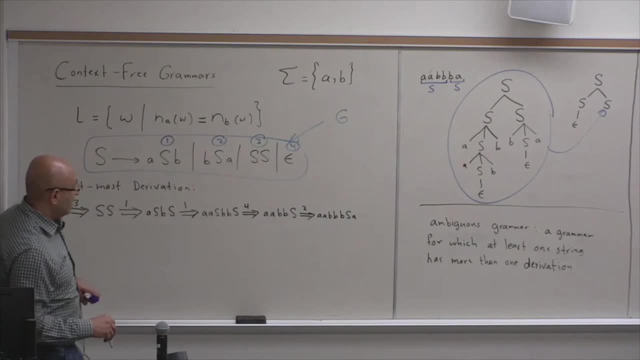 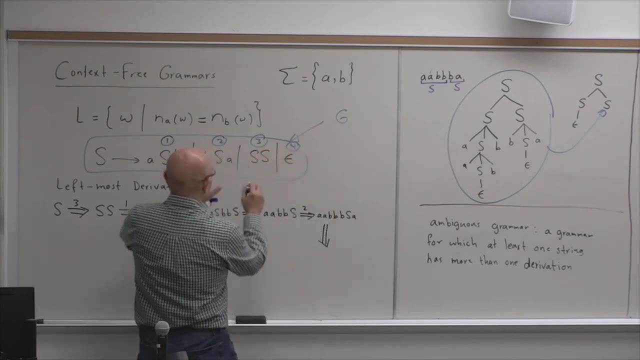 B, S A. We should not skip any step. So this gives us this. And finally, by rule 4.. Yes, Yes, So I do A, A, B, B, B, A. Okay, So, step by step. 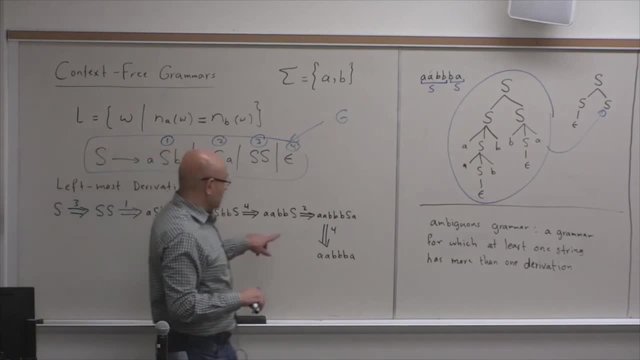 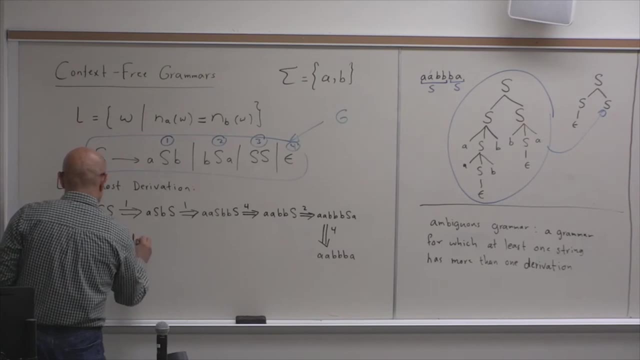 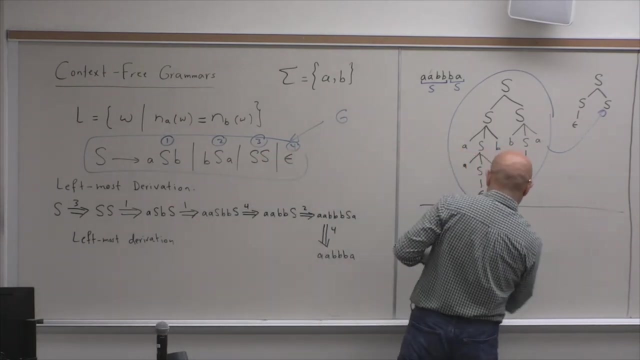 We shouldn't skip any step. So this is the leftmost derivation. Now let me do a rightmost derivation for the same string. Let's see what the rightmost derivation. So we're going to do a rightmost derivation for the same tree. 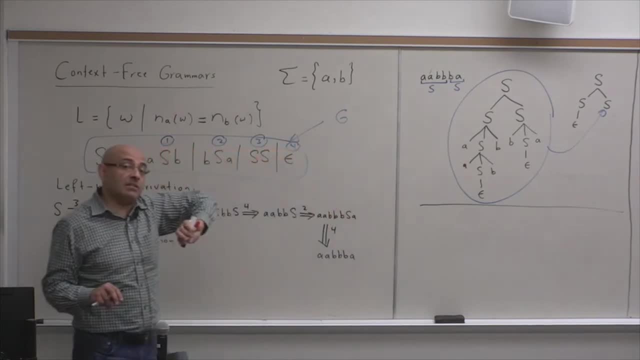 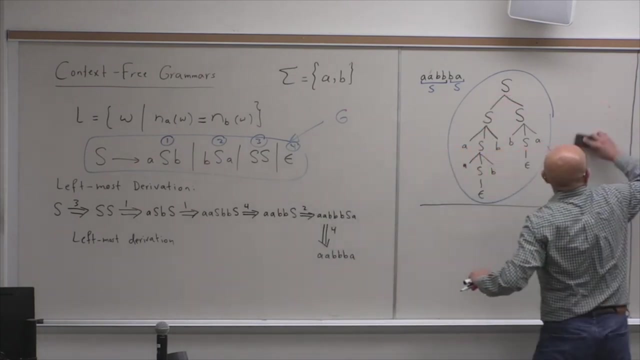 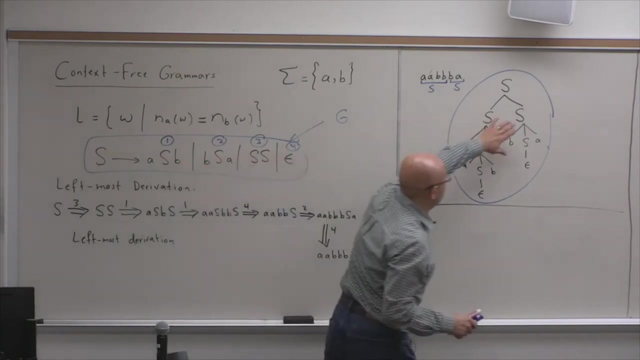 So the rightmost derivation is not a unique derivation, It's not distinct from the leftmost, So the same derivation. you can do it left to right or right to left, So forget about this other derivation. So this can do. you can do it right to left as well. 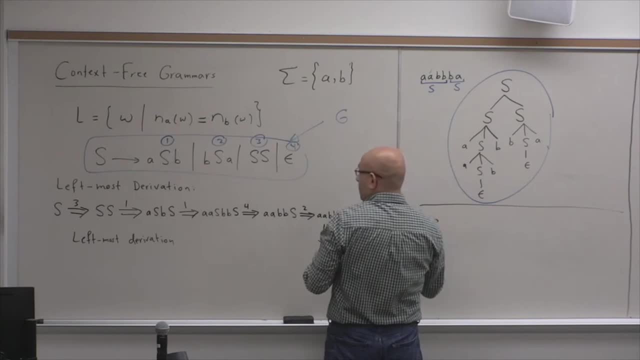 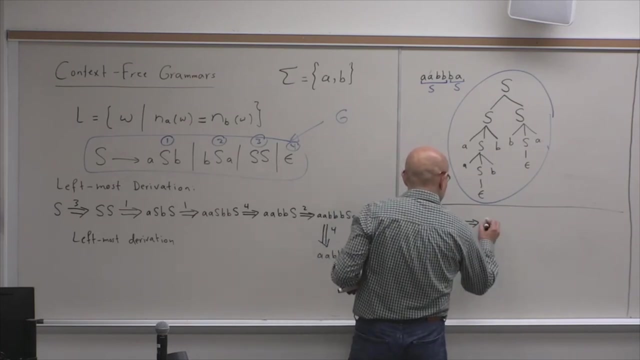 So you can do S by rule 3, you get S S Now. you substitute for the right first. So what do I substitute for? the right B S? sorry, first the left, then I substitute for the right B S A. 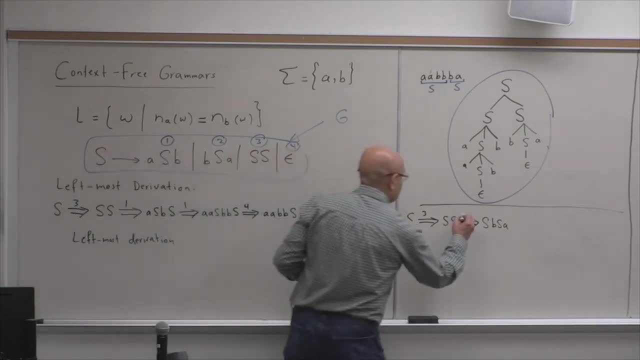 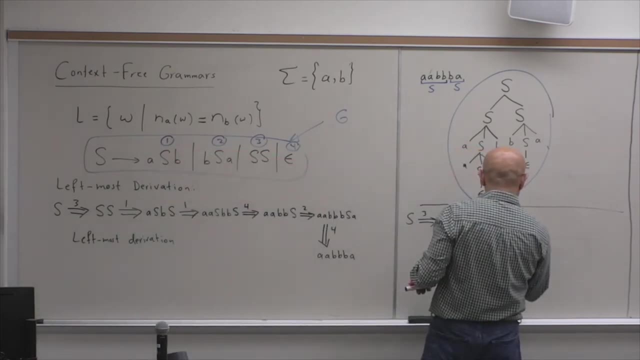 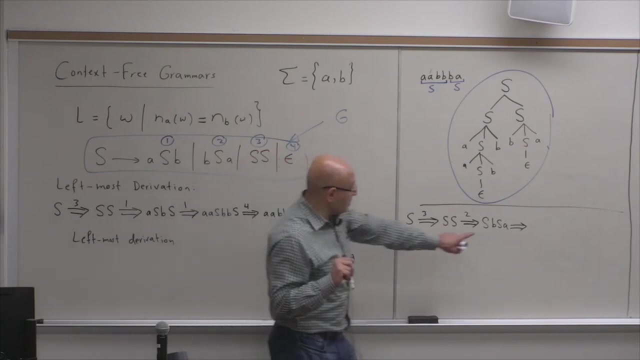 Which rule did I use? Rule number 2.. So here I started with rule 1.. Here I started with rule 2.. Then I substitute: what? For which S should I substitute next? The rightmost S? The rightmost S is this: 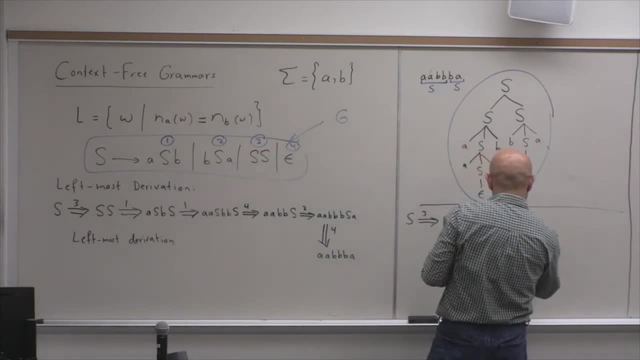 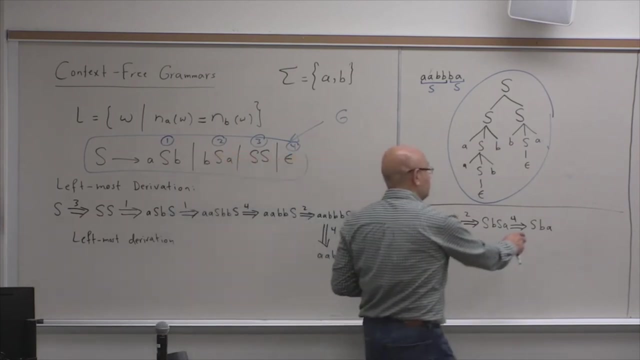 So I substitute an epsilon. So it's going to be S B A By rule 4.. S yeah, S B A by rule 4.. Then I expand this: S B A by rule 4.. 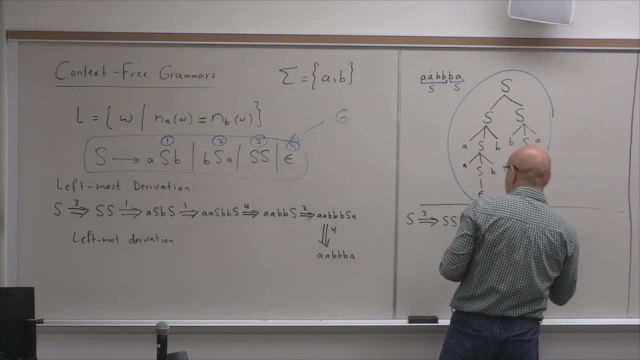 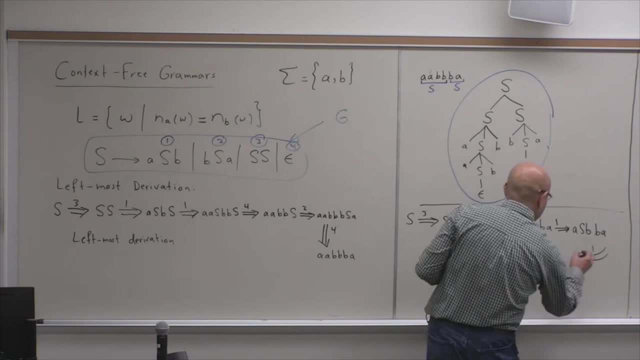 A. Let me make it clearer. This is A A, S, B, B, B A. This is A A, S, B, B, B A A by rule number 1, then which rule do I use? 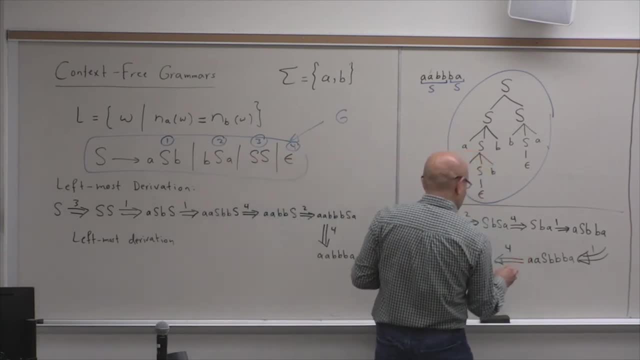 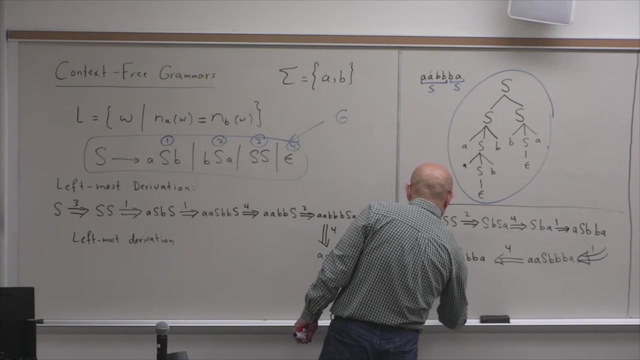 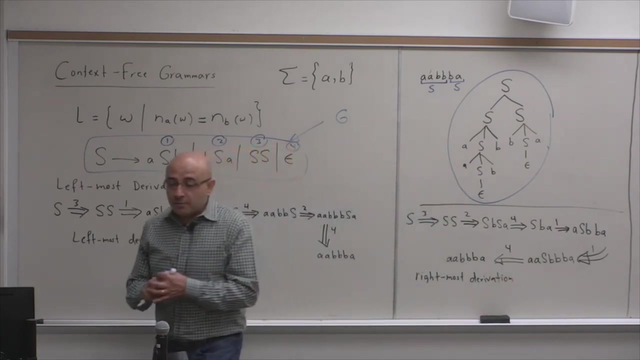 Yeah, the rule for the epsilon, which is rule number 4.. I do AA, B, B, B, A. OK, so this is the rightmost derivation. So the leftmost and the rightmost derivation, they are just two different ways. 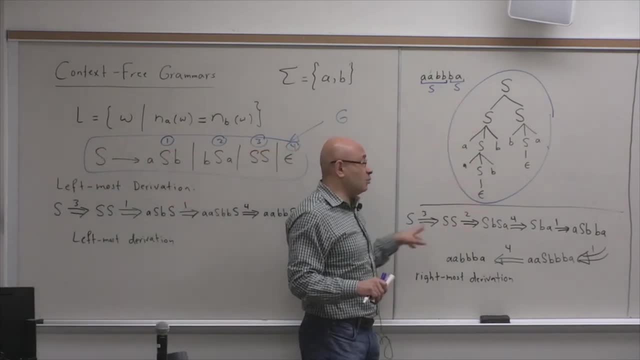 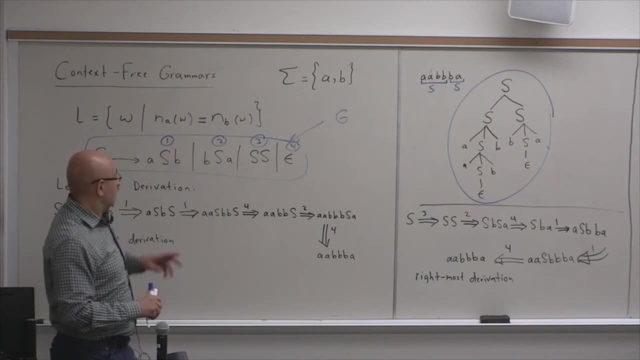 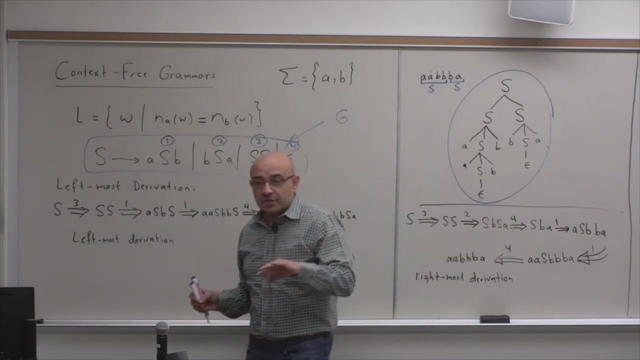 of doing the same derivation. So they don't count as two derivations, They count as one derivation. So in fact, in every language that has multiple symbol on the right-hand side, you will always have a leftmost derivation and a rightmost derivation. 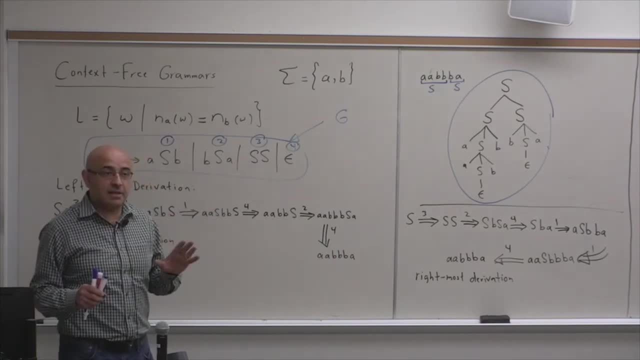 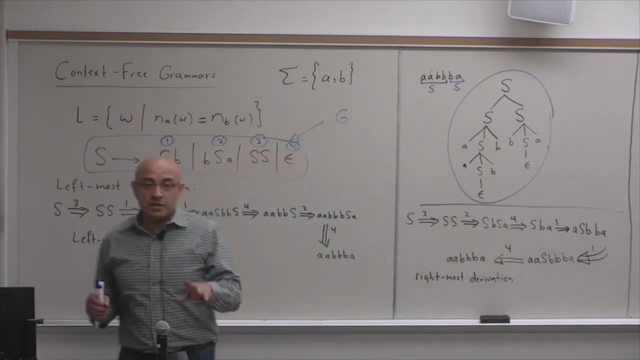 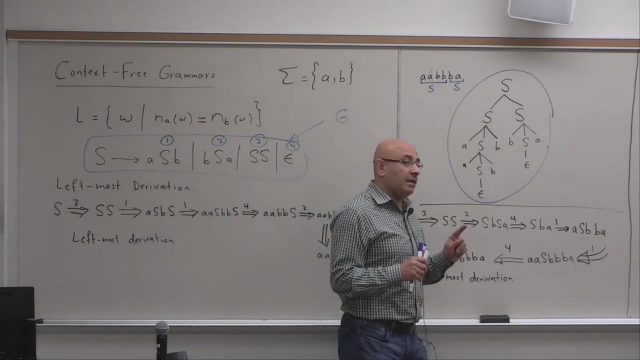 And having a leftmost derivation and a rightmost derivation doesn't mean that the language or the grammar is ambiguous. OK, So having a leftmost and a rightmost doesn't mean that the grammar is ambiguous. The grammar will be ambiguous if you can come. 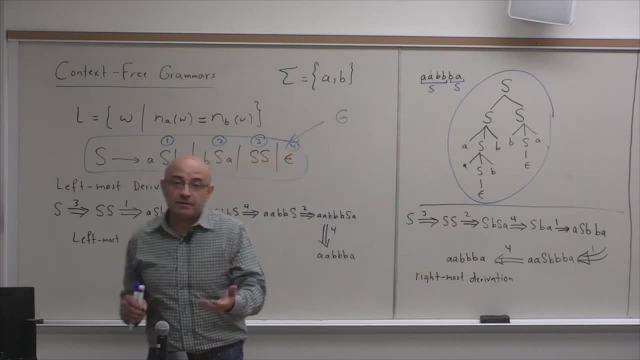 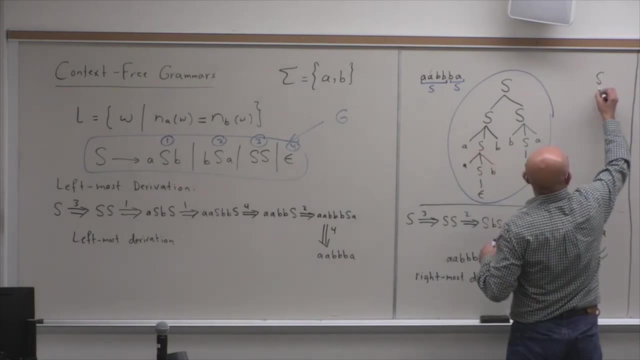 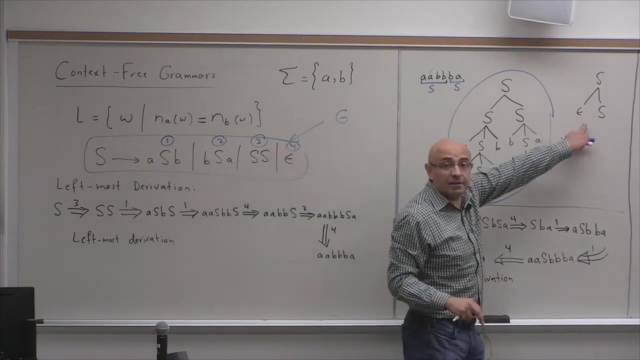 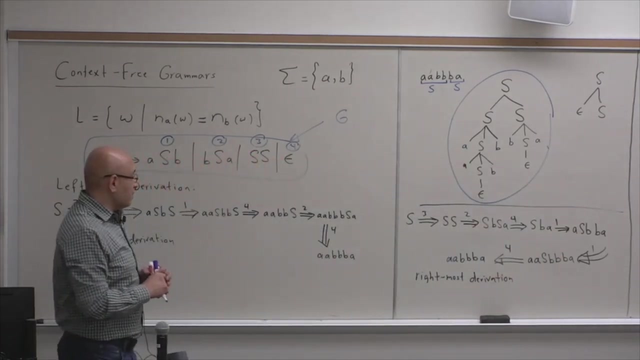 up with two actually different derivations, like two different derivation trees, Like this grammar. you know, we came up with this derivation with a different derivation tree, which is this: So this is fundamentally different. So this makes it ambiguous. OK, So are we clear on the concept of leftmost. 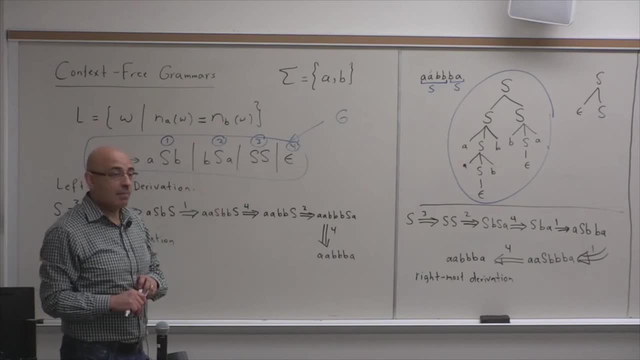 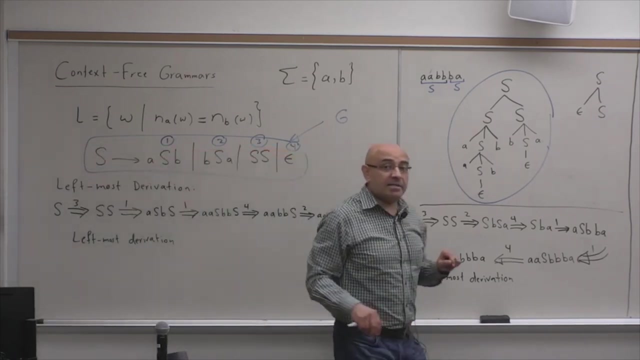 rightmost and ambiguous. One more thing that we need to know about this grammar is that this grammar is not a linear grammar. This grammar is not linear because we have multiple. we have multiple S's on the right-hand side. So a linear grammar is a grammar in which there can be 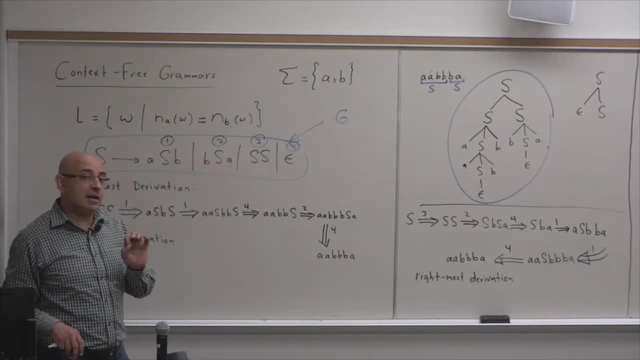 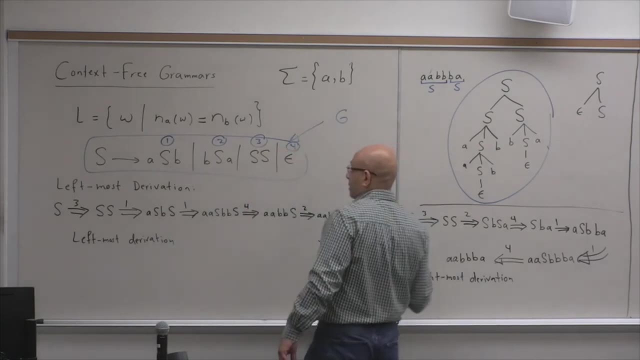 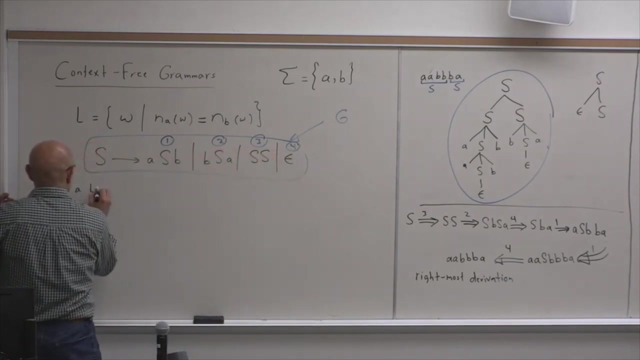 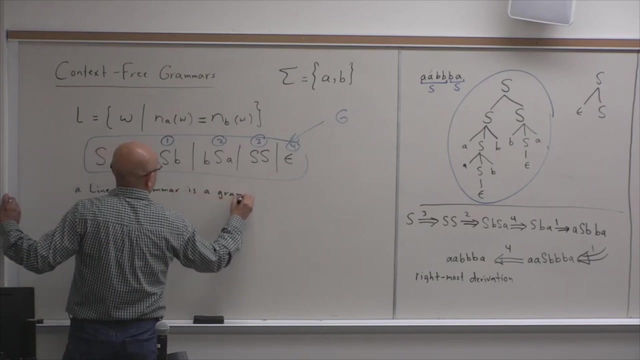 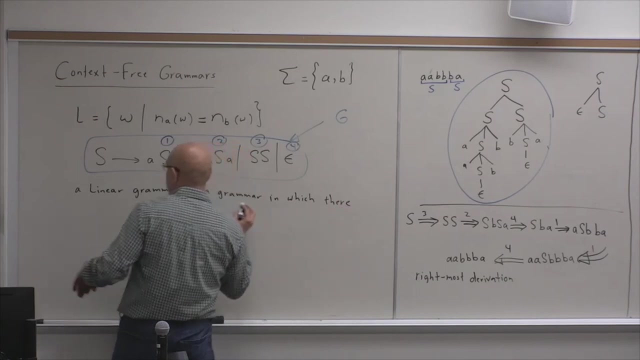 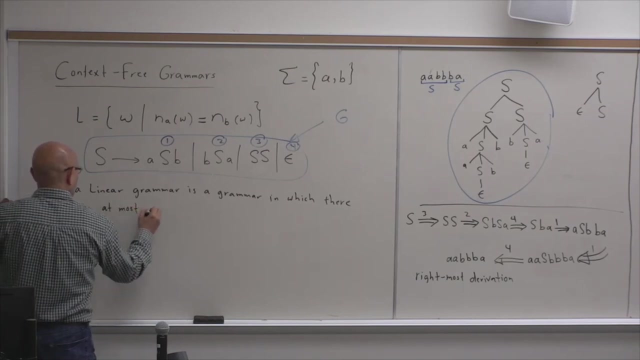 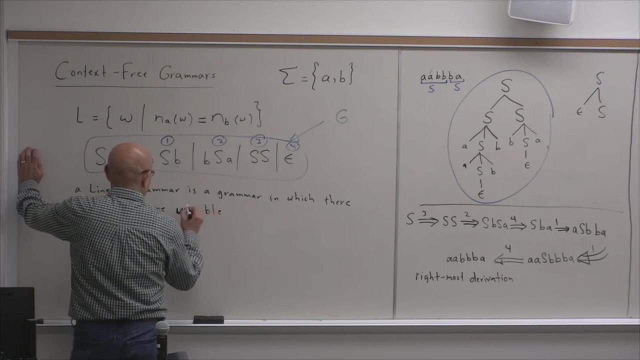 at most one symbol on the right-hand side of every rule. OK, So let me define a linear grammar, A linear grammar. A linear grammar is a grammar in which there is at most one variable. one variable- oh, did I say symbol? 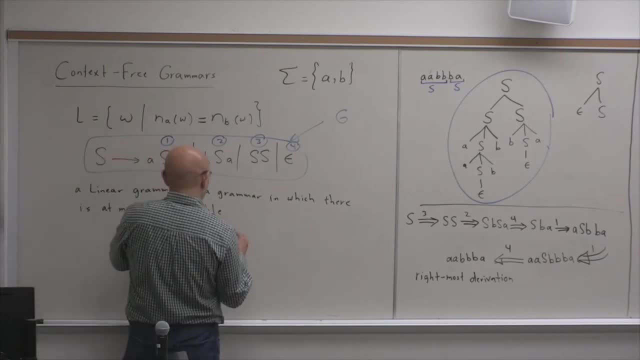 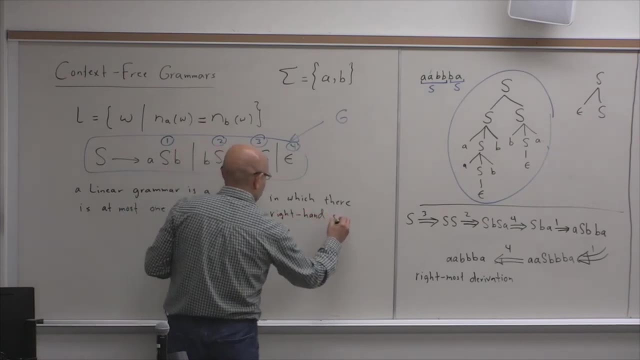 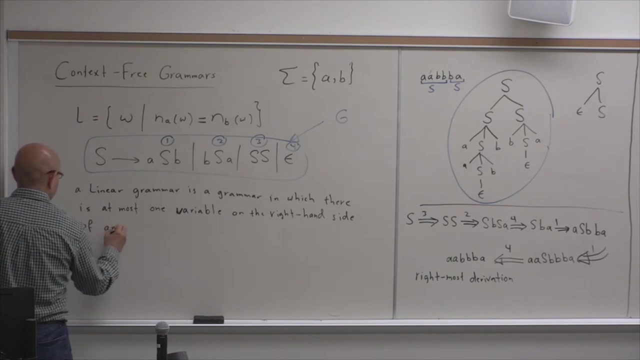 I meant variable, At least one, at most one variable On the right-hand side. there is at most one variable on the right-hand side of any production. In other words, if you have a production in which there are multiple variables on the right-hand side, 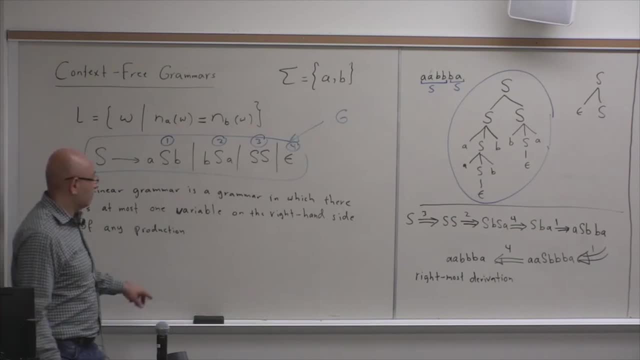 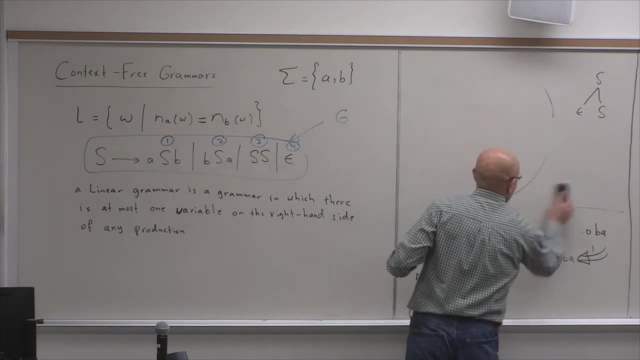 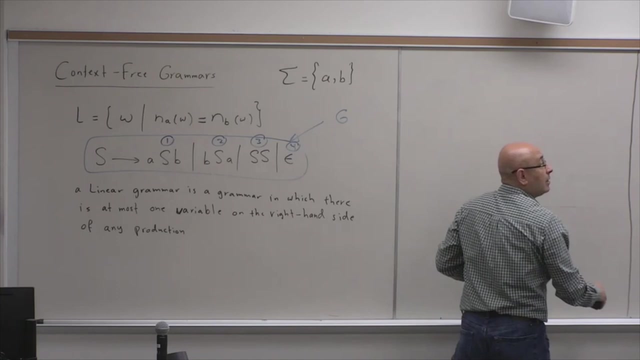 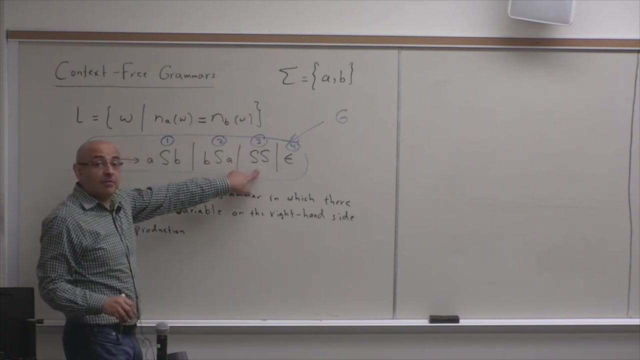 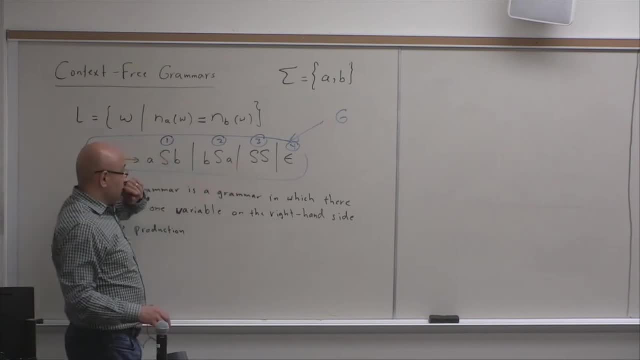 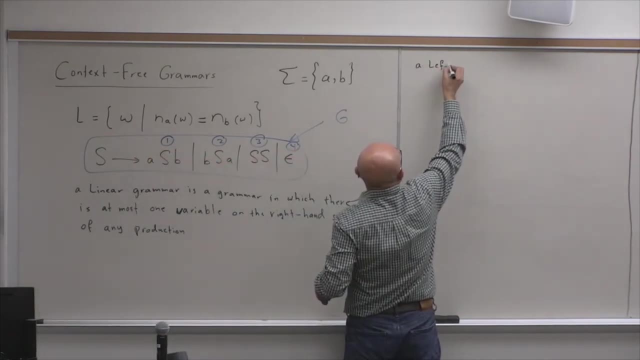 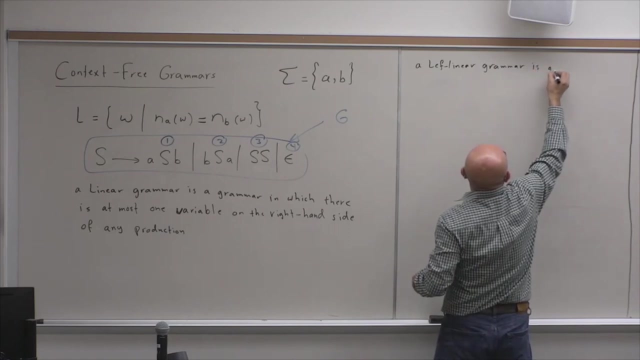 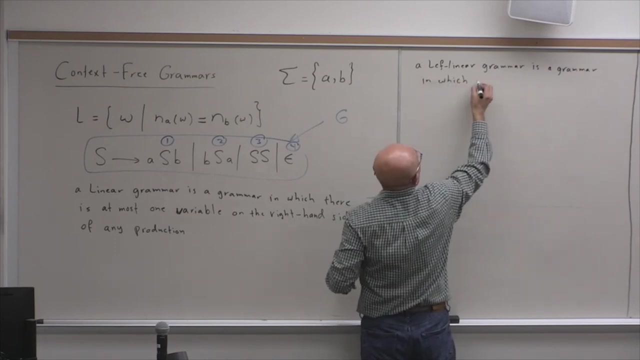 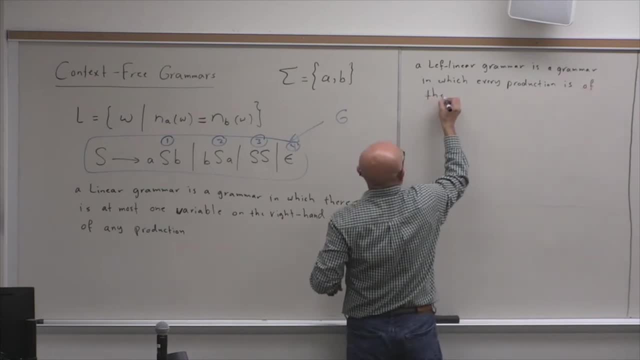 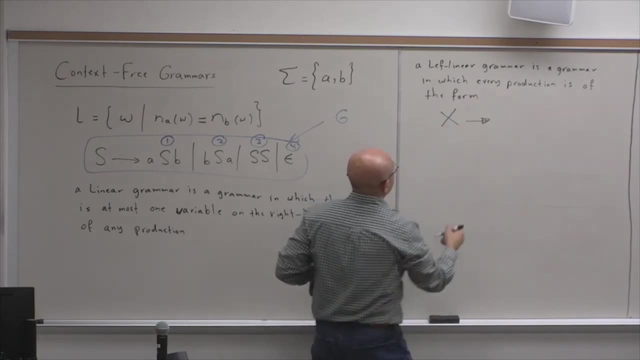 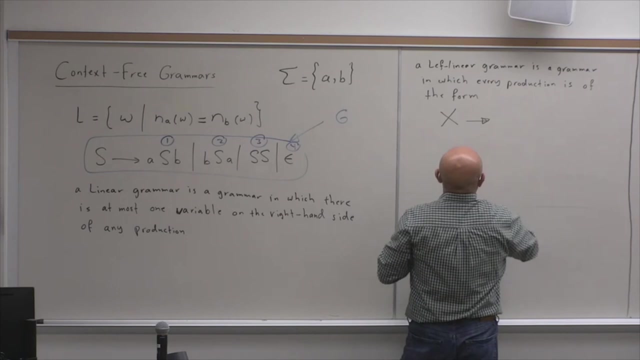 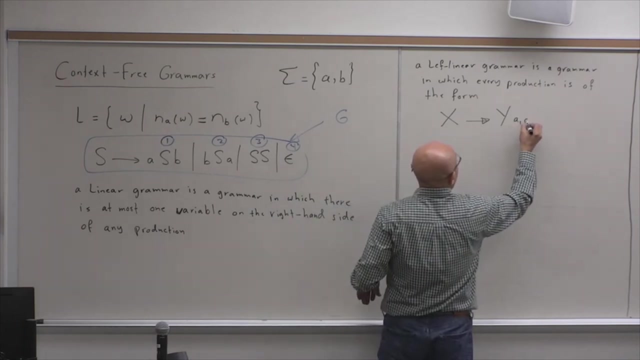 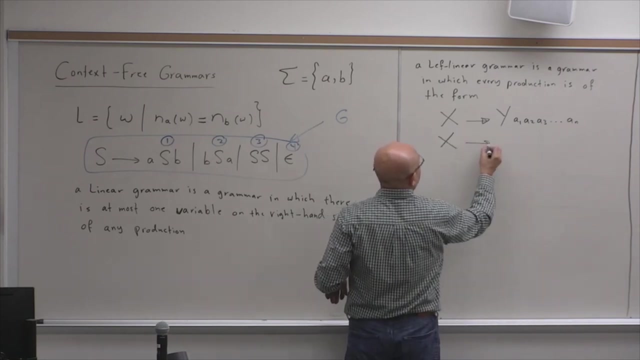 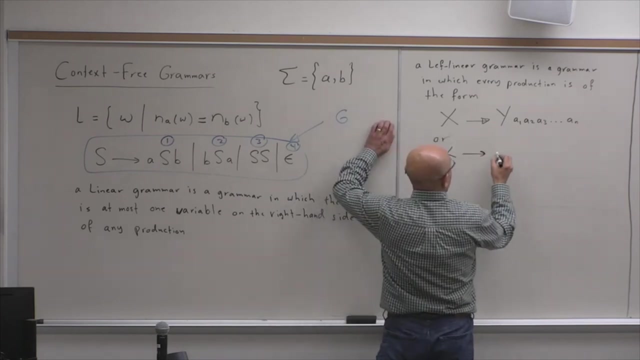 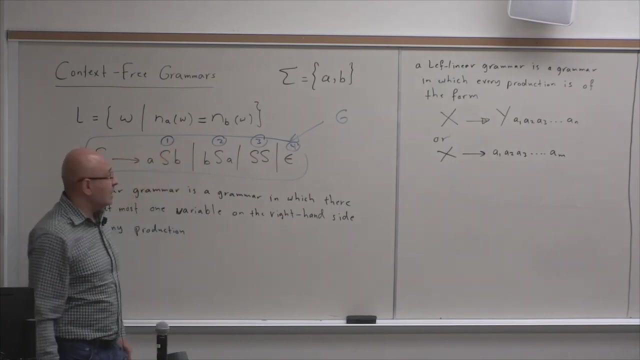 is of the form x, a1, sorry, this is x, y, a1,, a2, a3, through an or x, or the form or x is a1,, a2, a3, am. So if in your grammar every production either has: 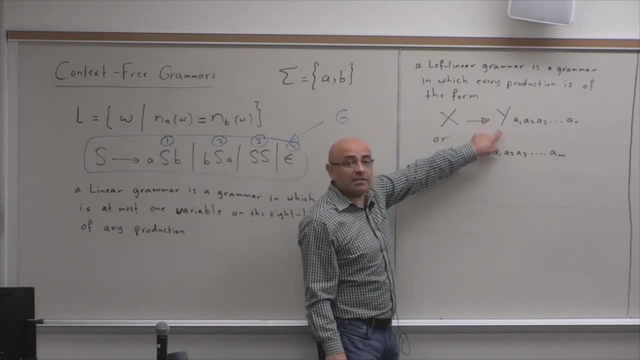 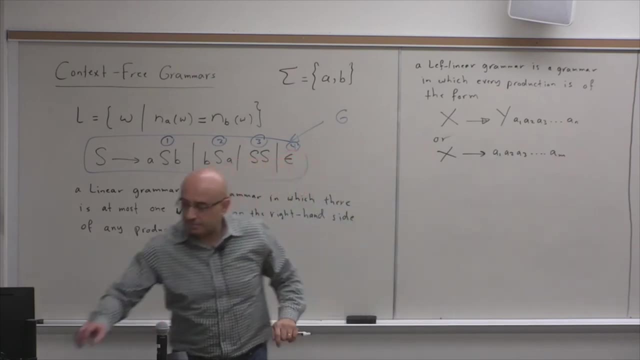 or doesn't have a function. So if in your grammar every production either has one variable that appears on the left-hand side, the left-most variable, the left-most symbol, is a variable followed by terminals. So these are terminals a1.. 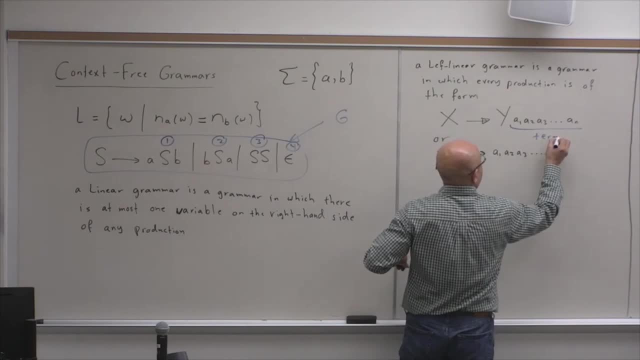 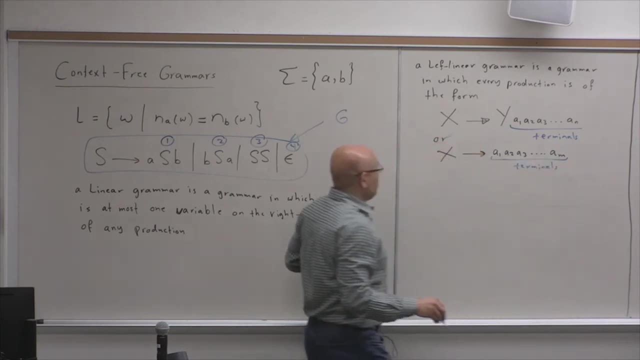 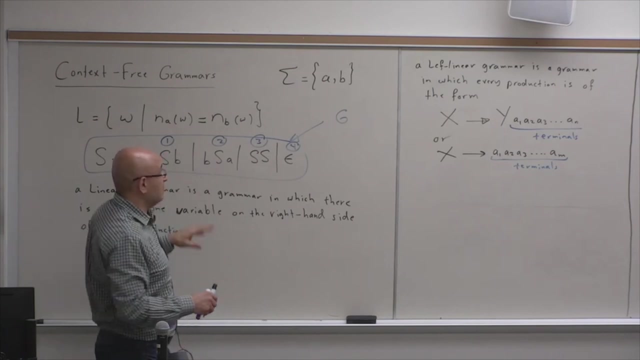 So these are terminals And these are terminals. So every production either doesn't have any variables on the right-hand side, So it's either completely terminals, or it has a, a variable that appears on the left-hand side. So this is, if a grammar is like this, 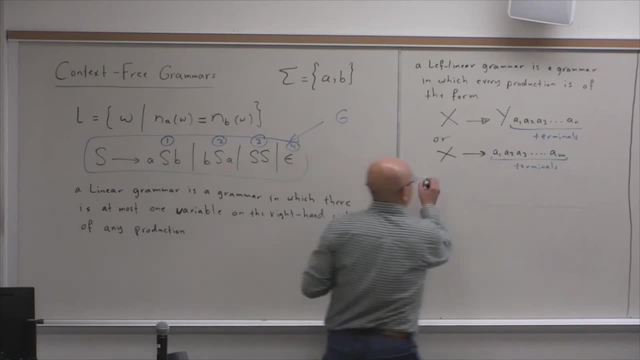 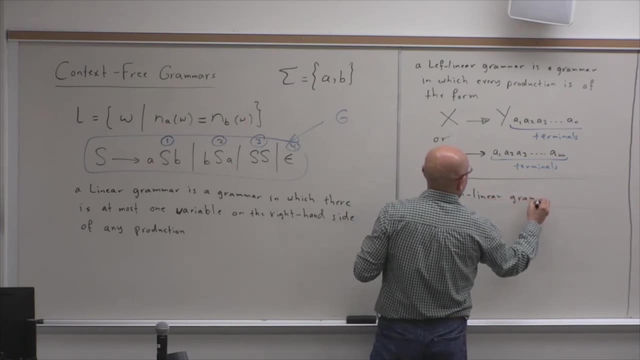 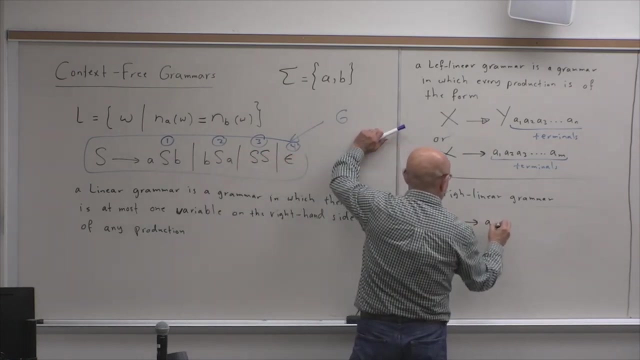 then it's a right left linear grammar. Of course, a right linear grammar is a grammar in which every production is of the form x a1, a2, through an y, or x a1, a2, through am. 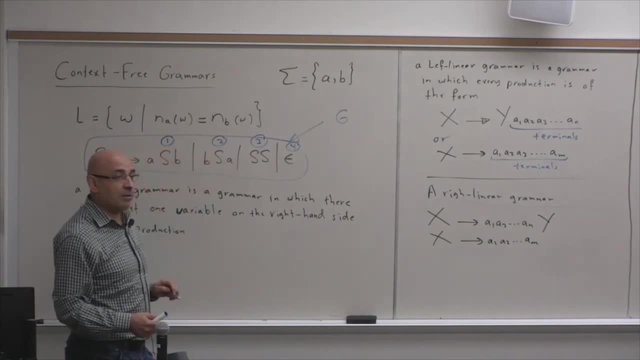 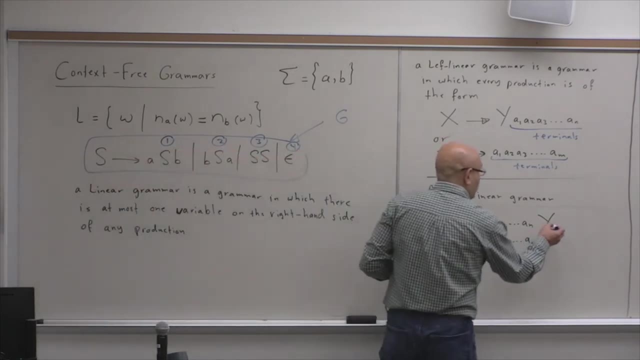 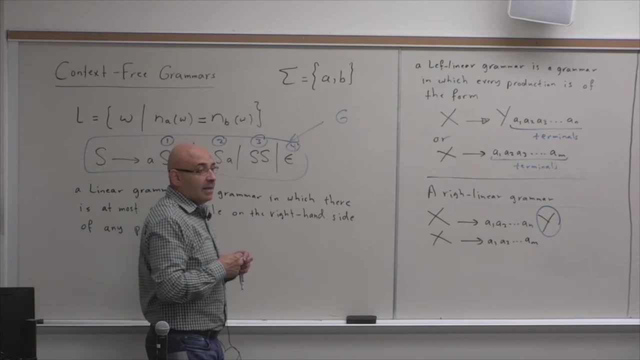 So a right linear grammar is a grammar in which there is only one variable on the right-hand side And this variable appears consistently in the right-most position or as the right-most symbol in every production. Now why are these left linear and right linear variables? 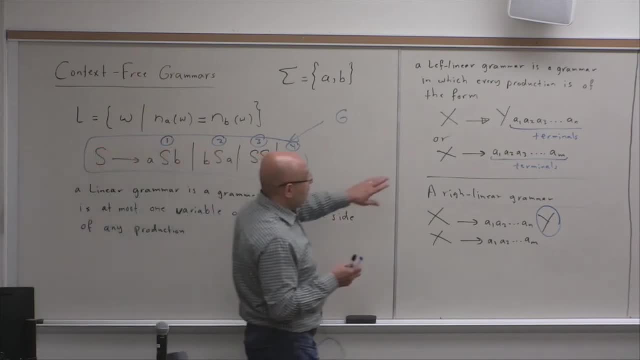 Why are these left linear and right linear grammars interesting? They are interesting because if a grammar is right linear or left linear, it's a regular grammar And calling it a regular grammar is not a coincidence. In fact, we call it a regular grammar because it will be. 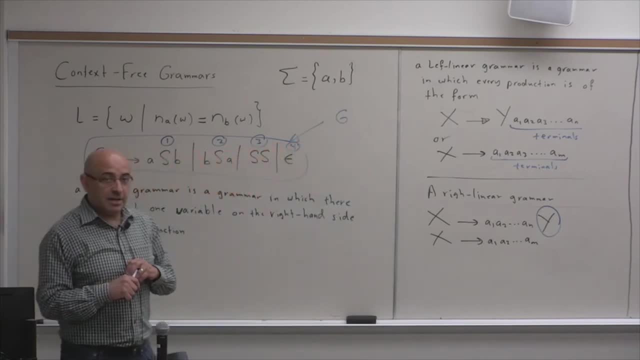 equivalent to an NFA or a DFA or a regular expression. And we will, you know, in the. in fact, in the next lecture we'll see a systematic procedure. for, you know, in the next lecture we'll see a systematic procedure. 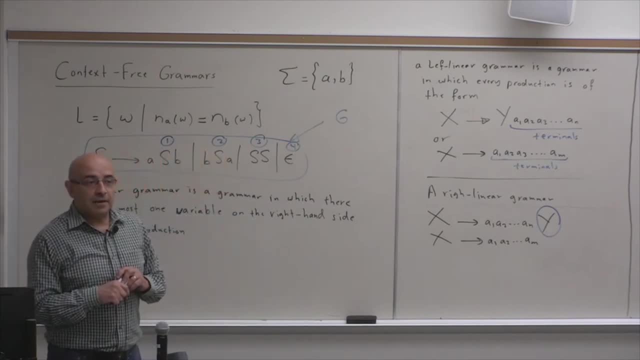 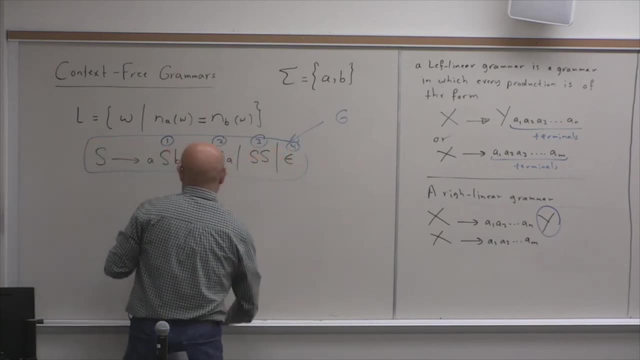 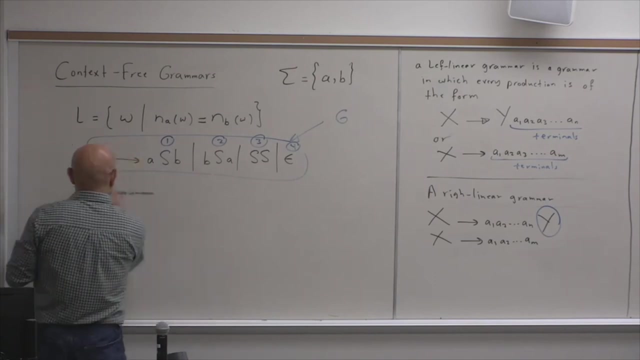 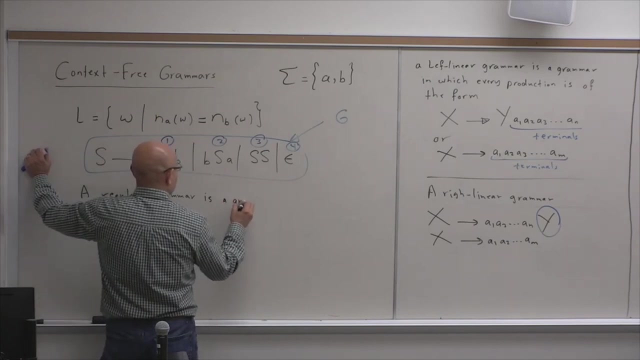 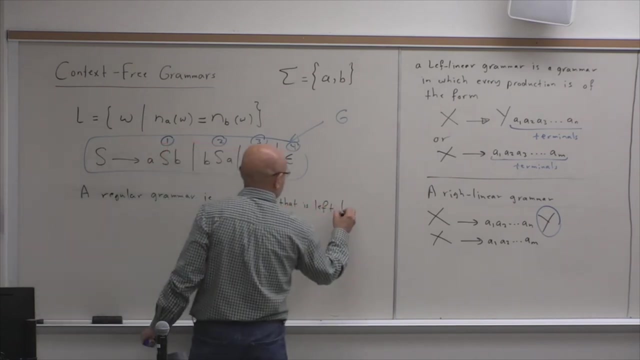 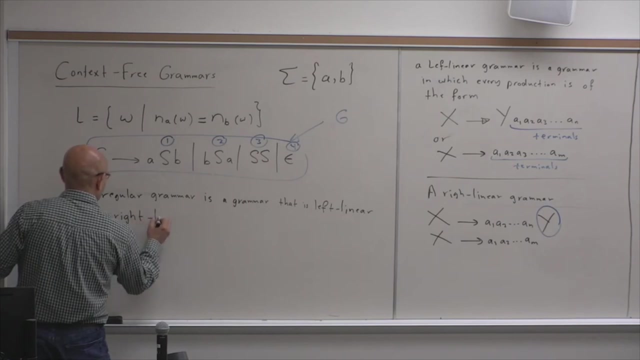 for converting a regular grammar into a finite automaton. So if a grammar- or well, we can define it- A regular grammar, a regular grammar is a function of a grammar that is left linear or right linear. Well, so we need an example. 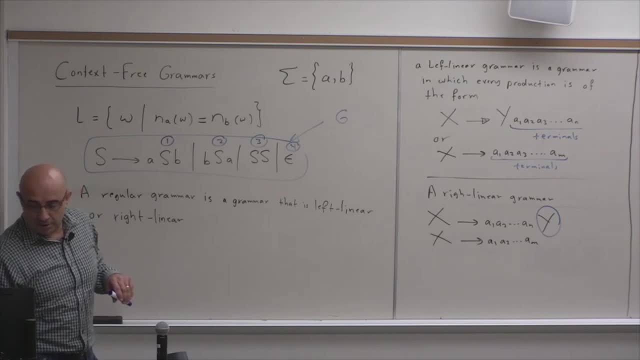 You know, today we will not go, we'll not get the chance to go through the systematic procedure for converting a regular grammar into an NFA or a DFA, but we will go through an example. Okay, So we need an example that will show us. you know, 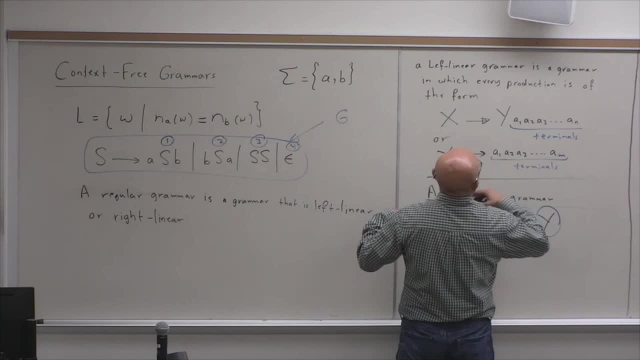 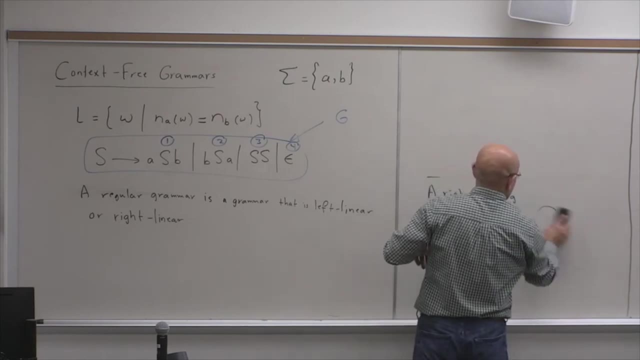 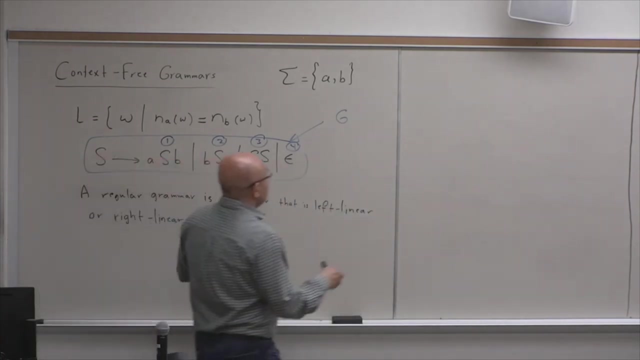 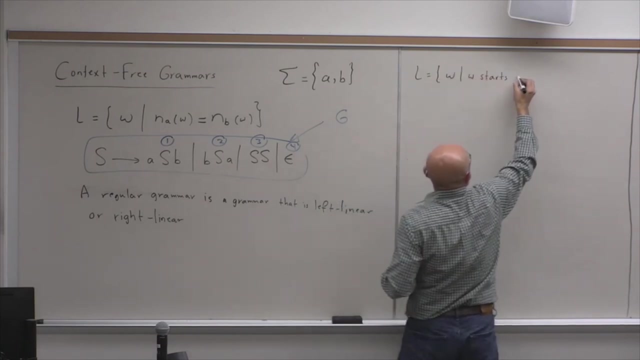 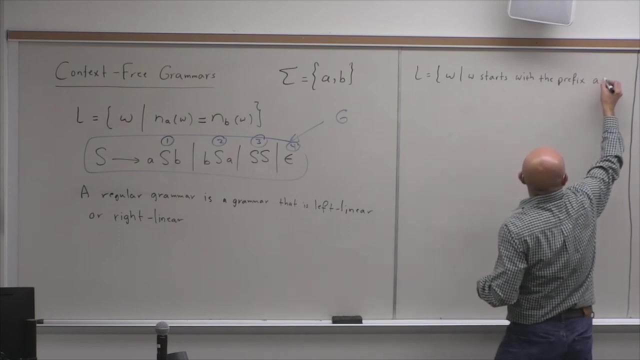 the relations or that we can, you know, always come up with a regular grammar for a regular language. So let's, let's look at this language W, such that W starts with a prefix A, B. Now is this linear. 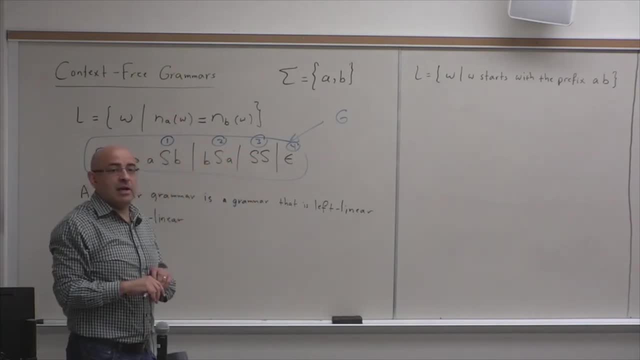 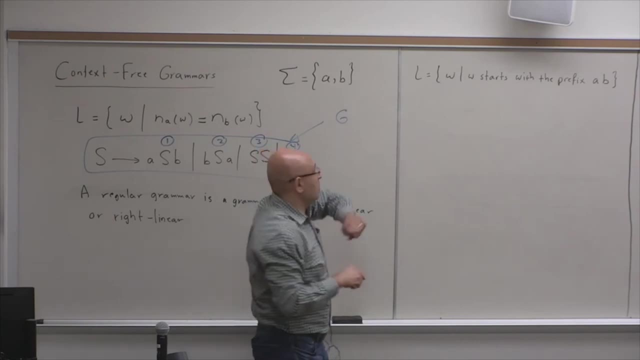 Sorry, is this a regular language? Of course it's a regular language. We, you know, we know how to construct an NFA or a DFA or a regular expression for this. So a regular expression for this is what? Just A, B, what? 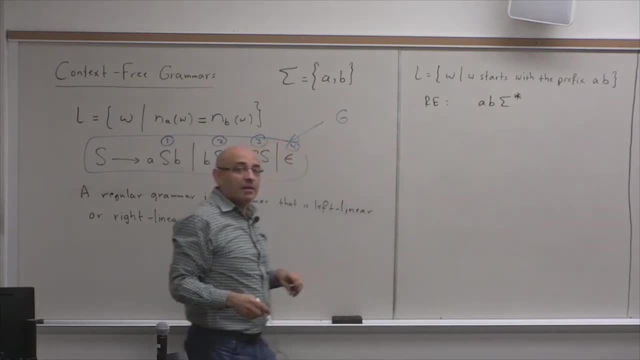 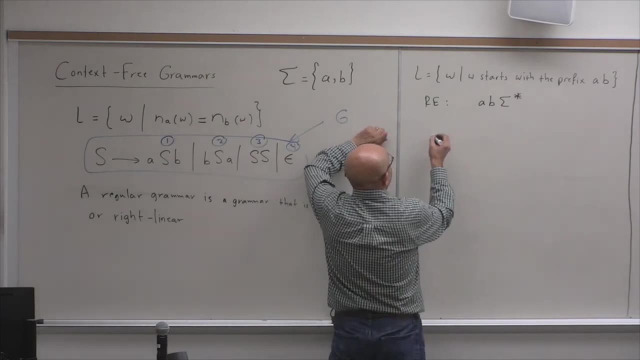 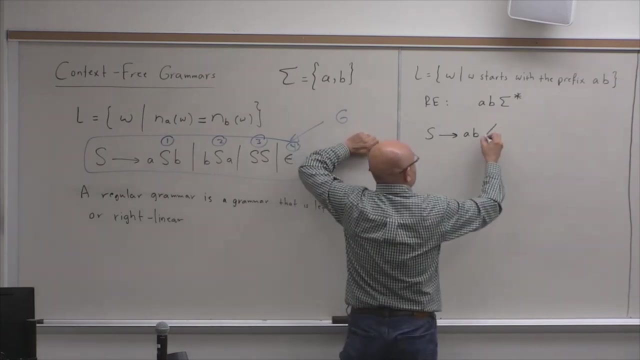 Sigma star. So this is very easy. We know that it's regular. How do we construct a grammar for this language? Well, we can do this. We can say: S is A, B, X. Now what should the X now generate? 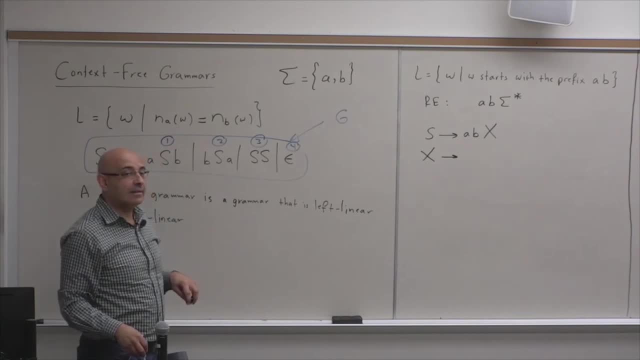 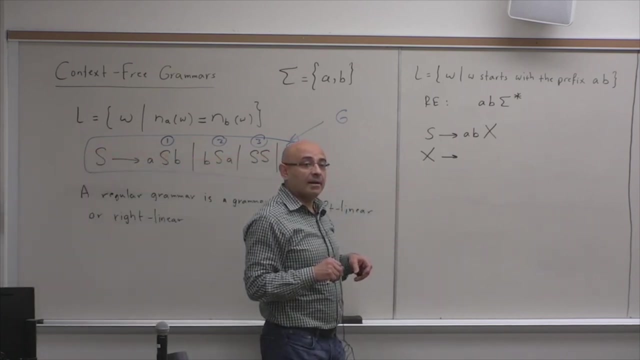 What should it generate? It should generate sigma star. It should generate, It should generate any string. And how do we write a grammar for sigma star? How do we write a grammar that will generate any string: AX or X. Okay, AX or. 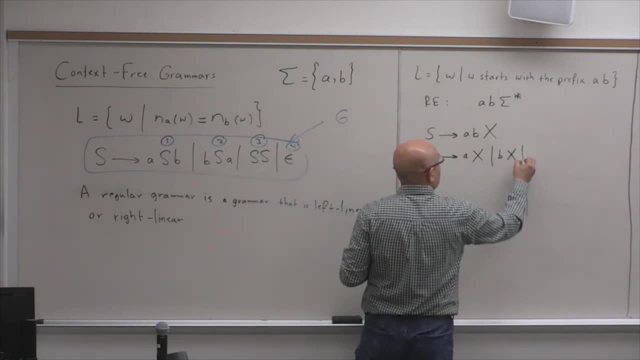 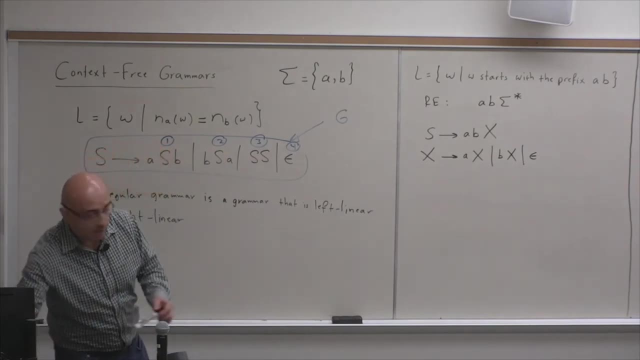 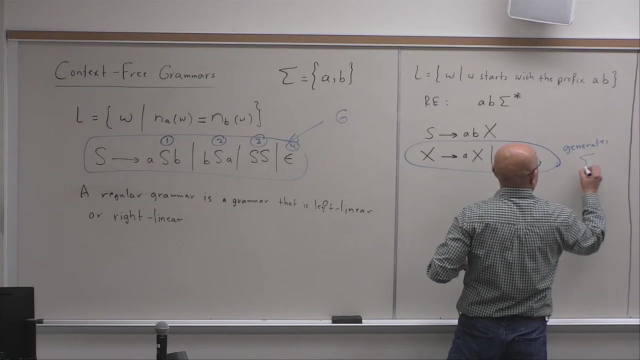 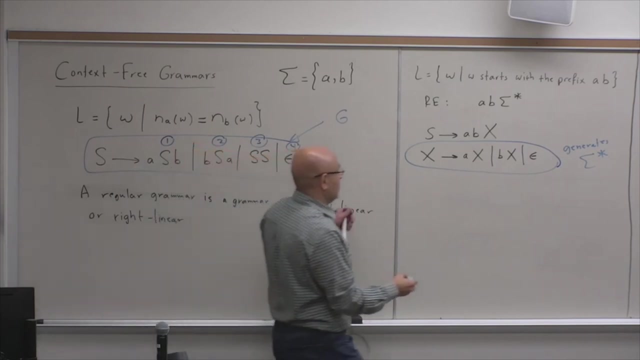 BX, Or BX or epsilon, This can generate anything, right? This can generate sigma star. So this, This generates sigma star, Right? So let's convince ourselves that it generates sigma star. Here's an X. I put you know AX. 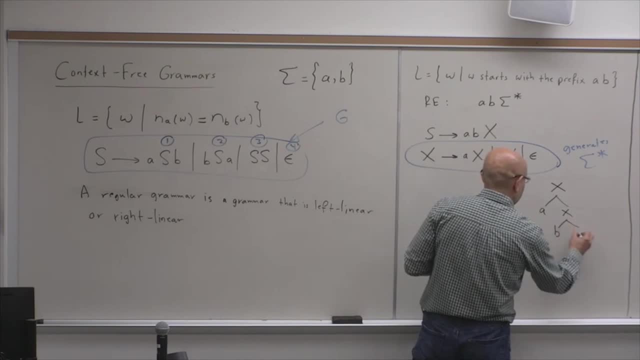 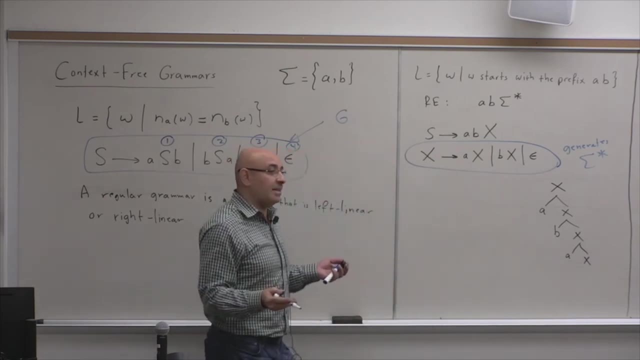 If I want a B, I just do a BX. If I want an A, I do an AX. If I want a B, I do a BX. So you can do. you can generate any string, So this can generate. 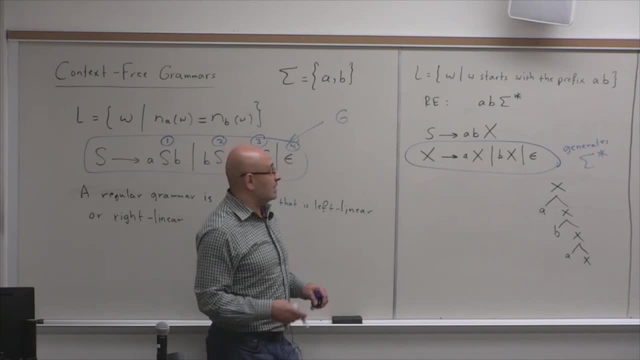 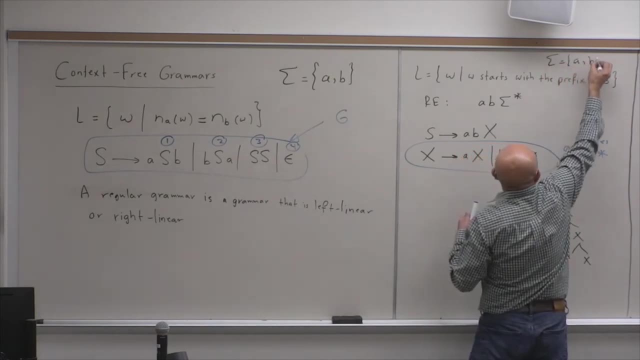 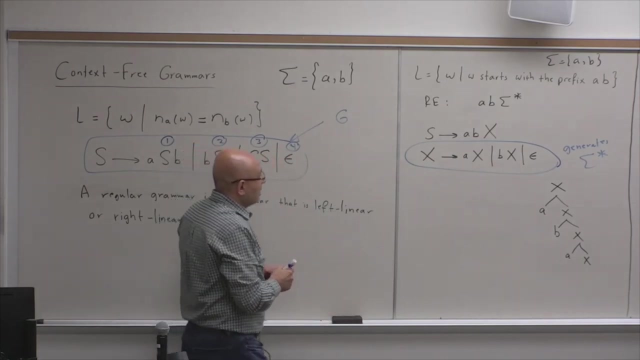 Okay, any string that belongs to the sigma star of this alphabet, Of course. here our alphabet is implicitly, or I didn't mention that- it's A, B, Okay, so is this grammar linear? Yeah, it's linear and it's more than linear. 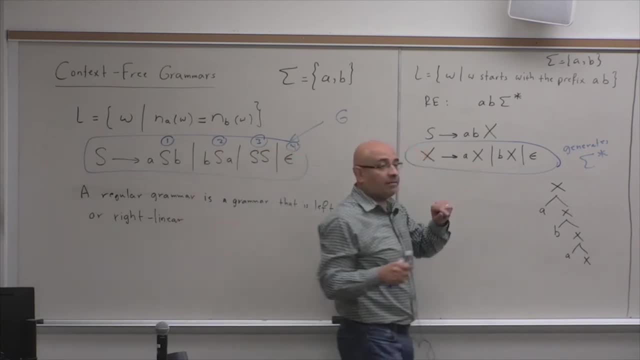 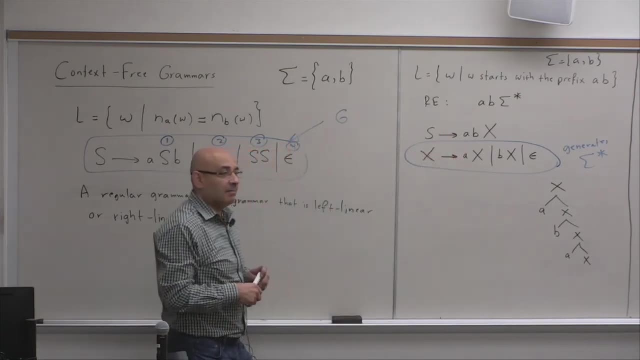 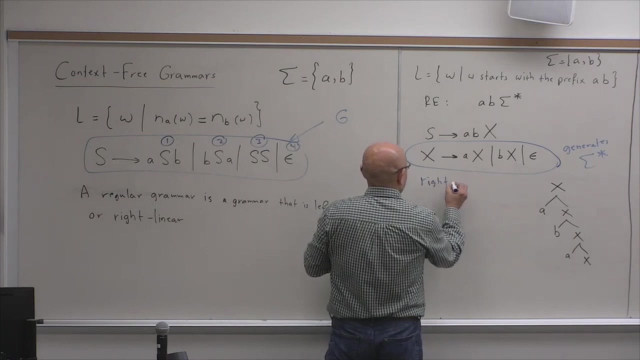 It's. is it right linear or left linear, Right linear. So if a grammar is strictly right linear, it's a regular grammar. But in fact I can make it. so this is right linear and regular. So right linear by definition. 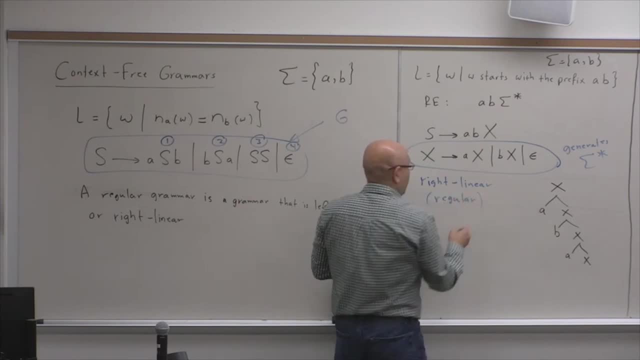 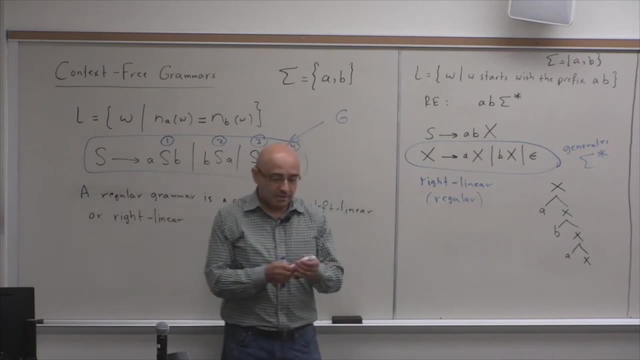 if it's right linear, then it's regular And, as we will see next time, we can take any regular grammar and convert it into a finite automaton. There is a simple, systematic procedure. There is a procedure for converting any regular grammar into a finite automaton. 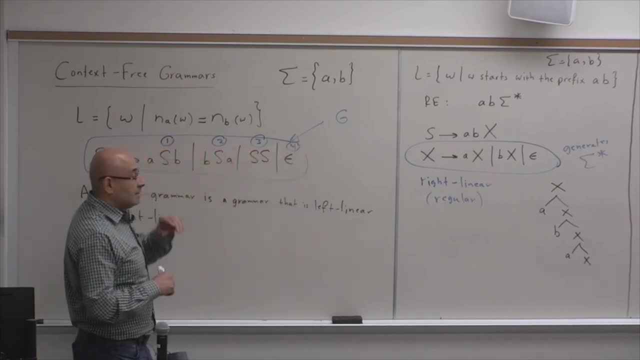 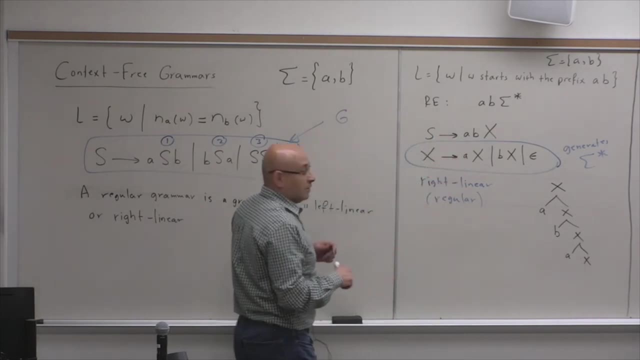 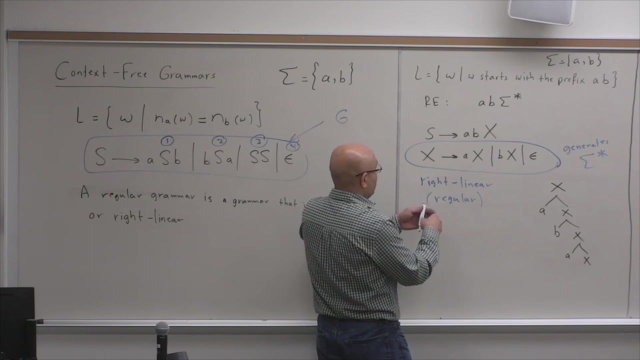 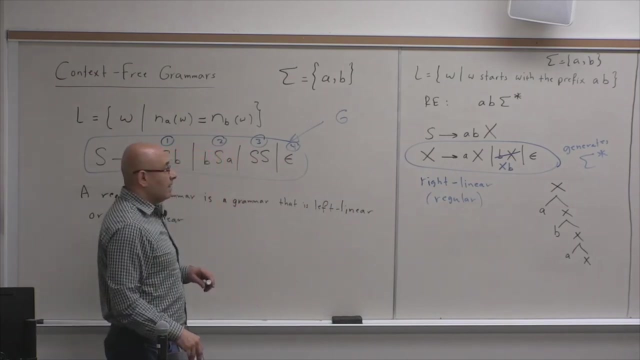 But the point here, the subtlety here, is that I can turn this grammar into a grammar that is not regular. So if I just do this, if I, if I change this to XB, then it will still generate sigma star, right. 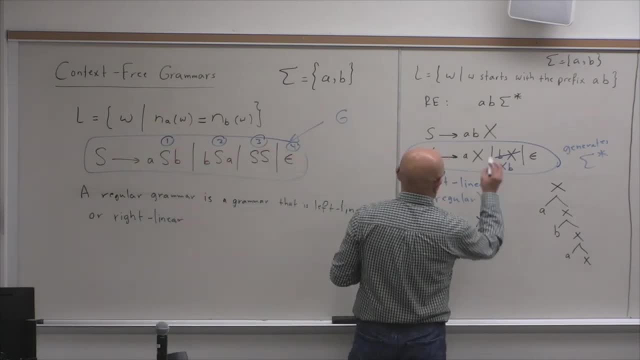 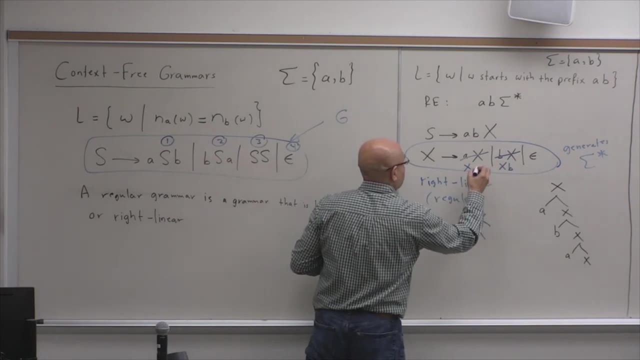 So X or I can generate, I can change both of them: XB. So to make it XA. sorry, to make it simpler, If I change it to from AX to XA, to XB now is this: 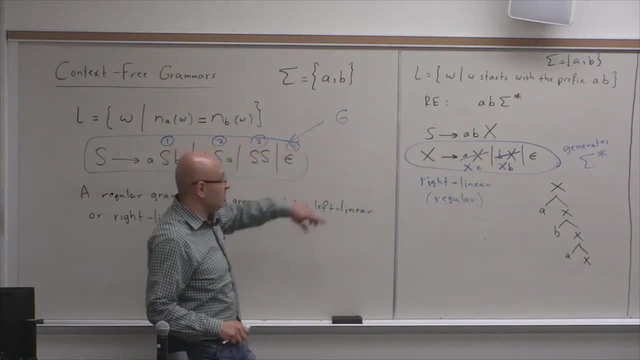 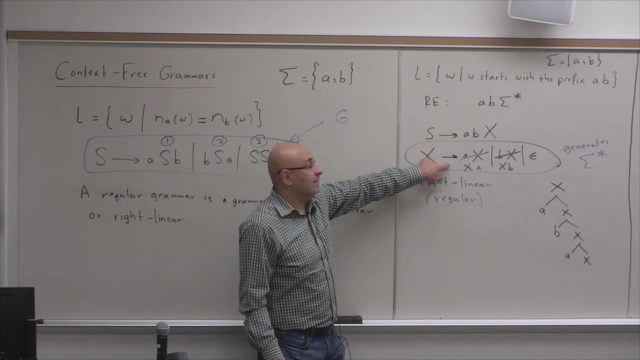 first of all, is this grammar? does this satisfy the definition of a regular grammar? No, it doesn't. Is this right linear or left linear? It's mixed. it's not right linear or left linear, So it's a mixed linear. 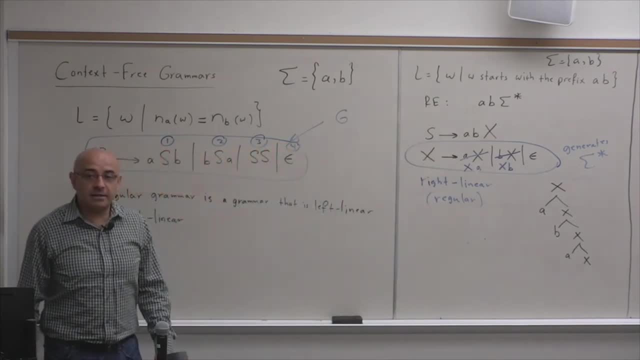 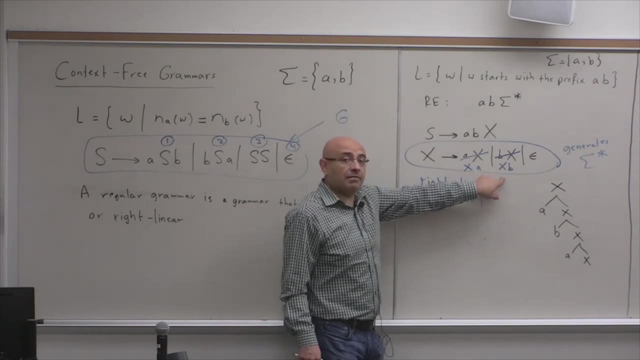 It's not right. it's not strictly right linear, it's not strictly left linear, Because this production is has the variable on the right. These productions have the variable on the left, So it's not right linear or left linear. 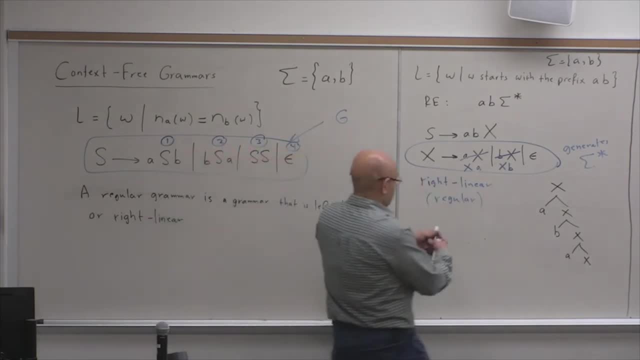 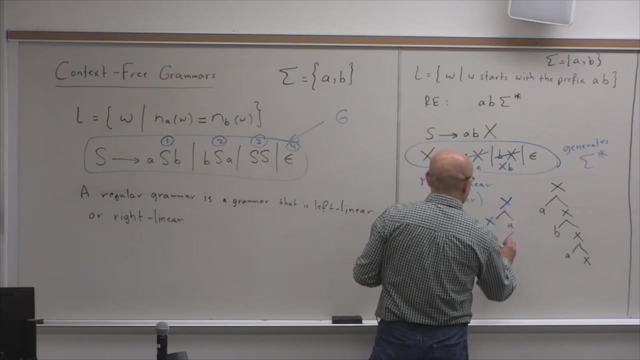 But it can still generate the same thing, Because here you know X, you can do, you know XA, you can do- sorry, XA, and you can do so. it will grow in the other direction. Yeah, then you can do XB or XA, whatever. 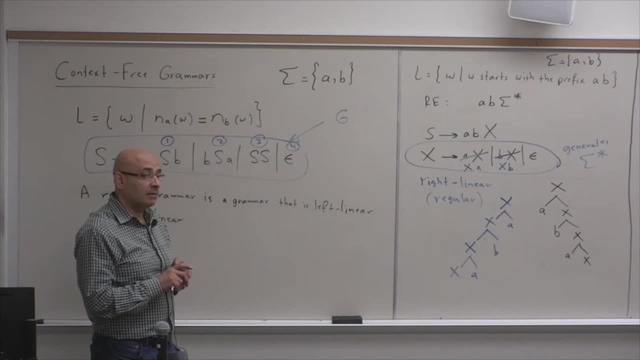 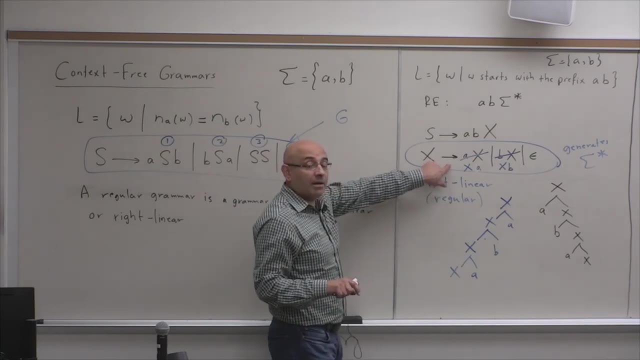 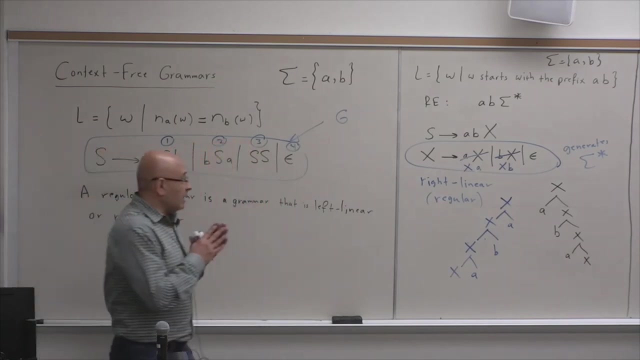 So you can generate sigma star. yes, So there's mixed linear and non-regular, Yeah, but the subtlety is, this is a non-regular grammar, But it doesn't make the language non-regular, So a regular language, okay. so now let me ask you this: 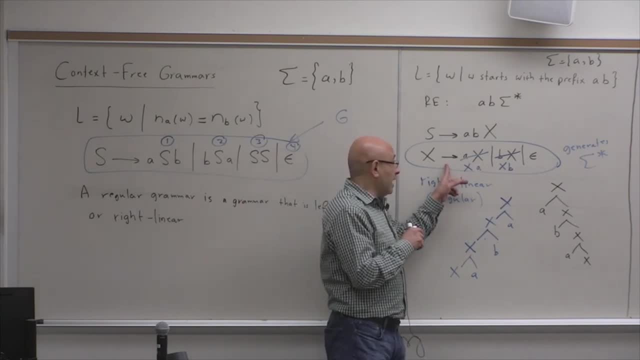 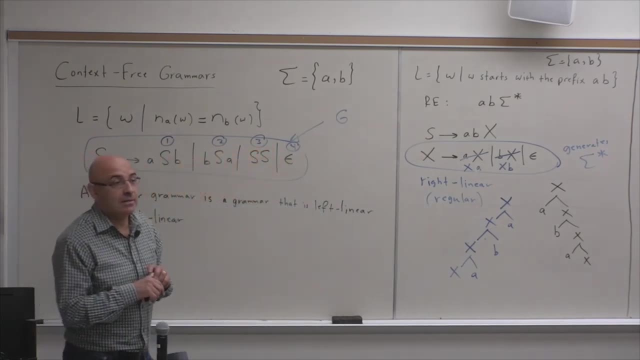 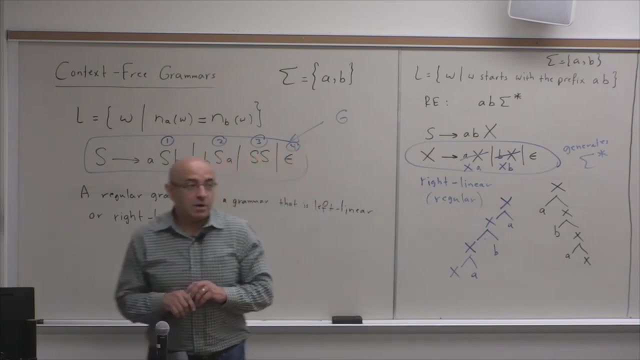 This is a non-regular, a non-regular grammar that generates a regular language. So now, how would you define a regular language in terms of grammars? What's the precise definition of a regular language in terms of grammars? What, so? how would you define it? 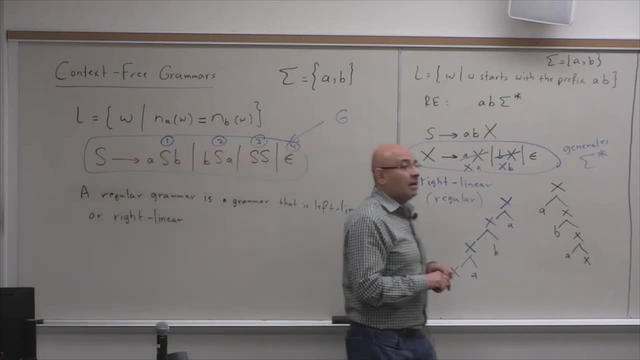 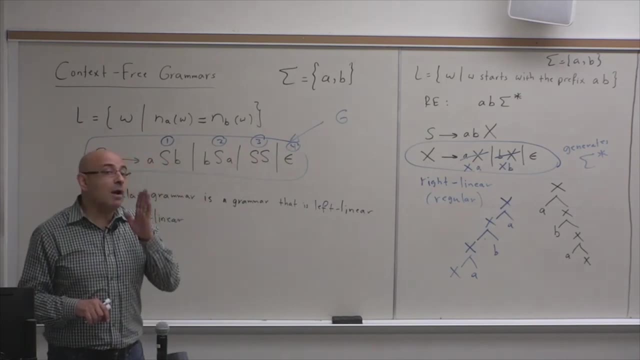 So you cannot say that it's a language that's generated only by regular grammars, right? You can say that a language is regular if there exists at least one regular grammar that generates it. okay, So if you can find one regular grammar, 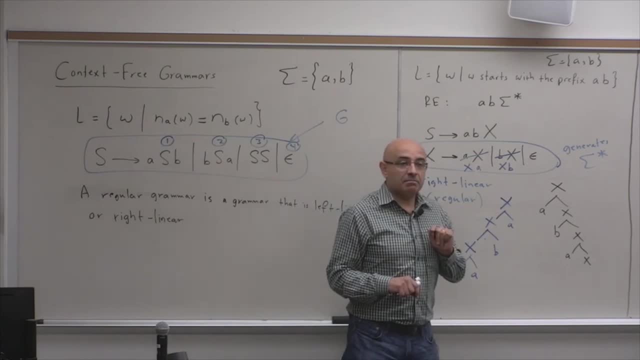 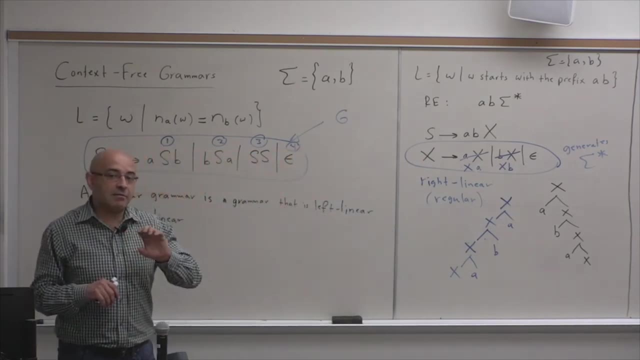 that generates a language, then it's a regular language, even if it has many non-regular grammars that generate it. So in order for the language to be regular, it doesn't have to be not all the grammars that generated. 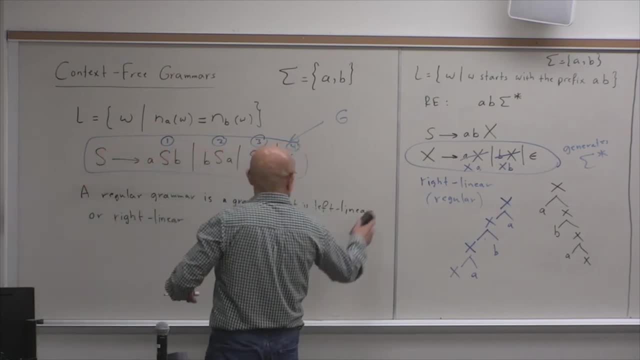 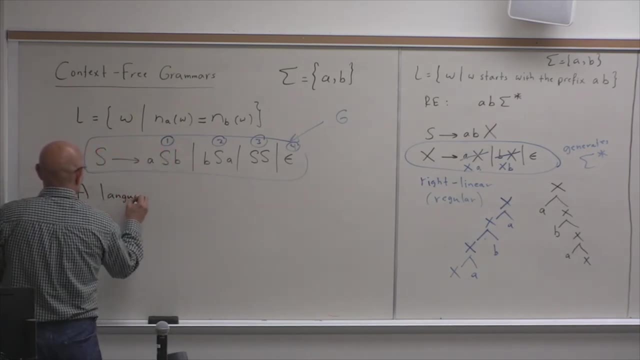 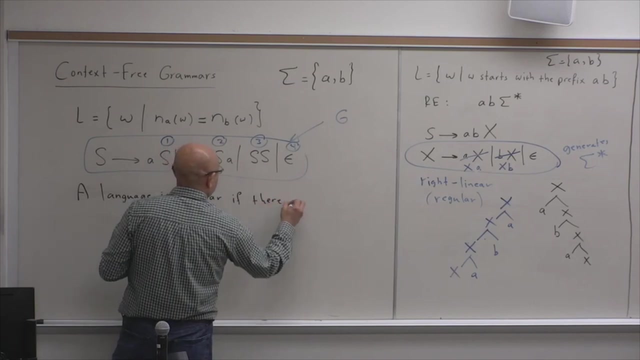 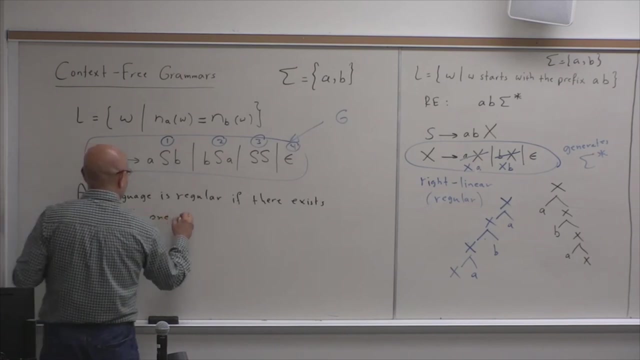 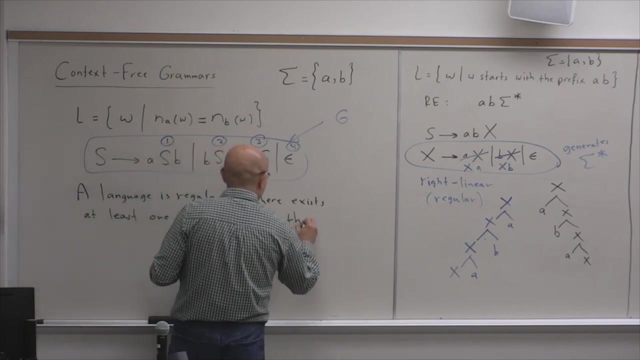 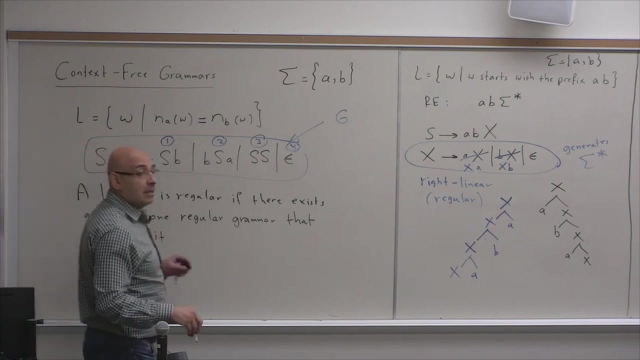 generate it have to be linear, regular. So a language is regular if there exists at least one regular grammar that generates it. In fact, I can make these, I can come up with an equivalent grammar here that is not even linear. 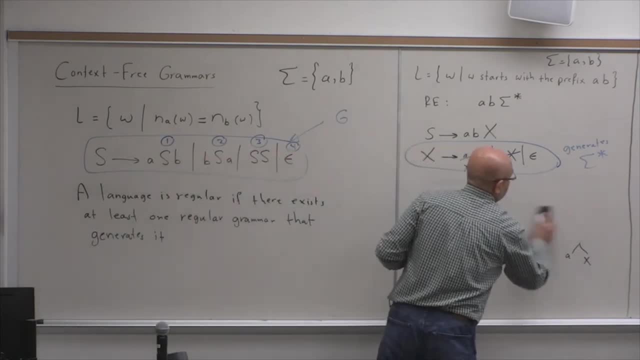 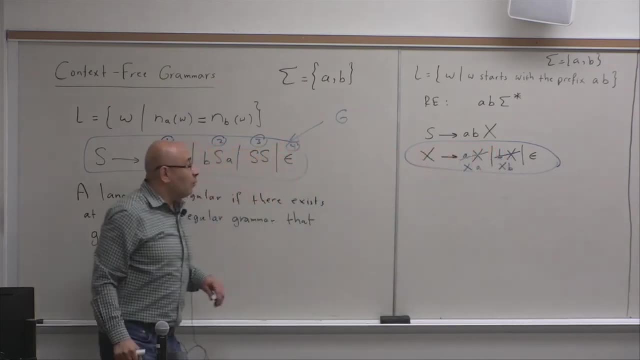 Can you, can you turn this grammar? you know, can you easily come up with a, with a non-linear grammar that is equivalent to this linear grammar? Yes, what's that? I would be able to take that x rule and I would take the ax. 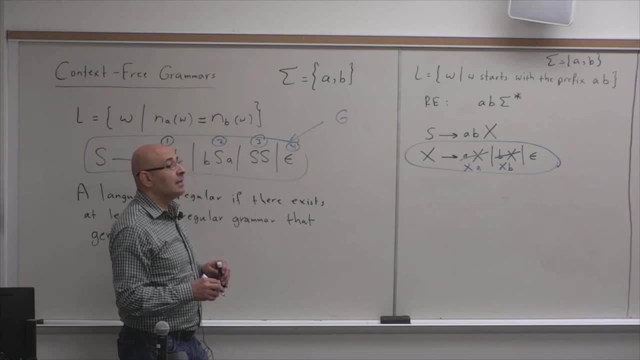 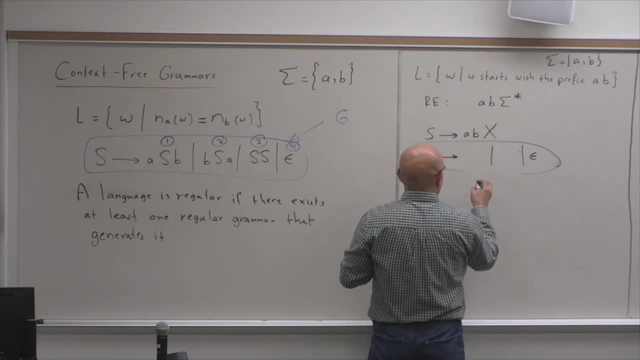 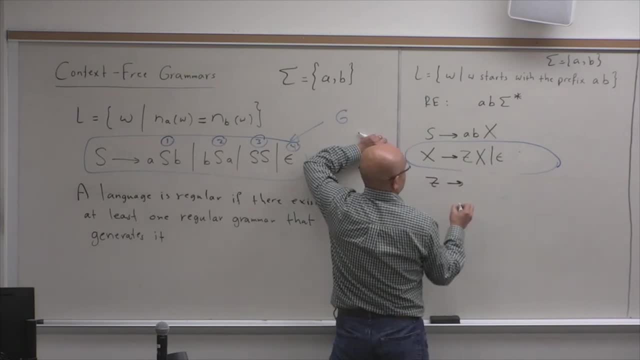 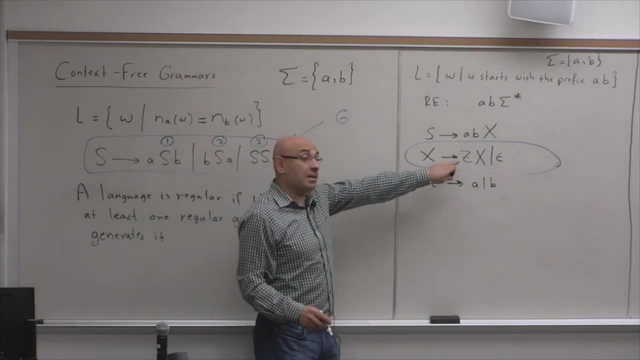 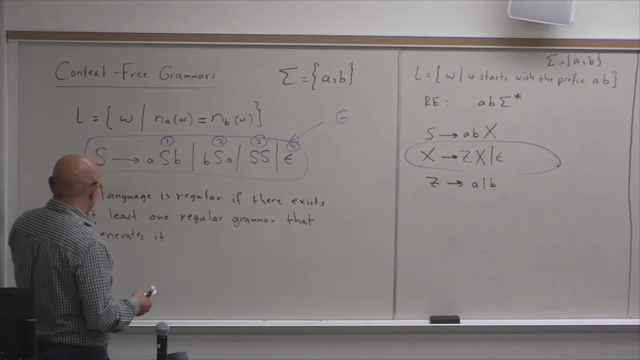 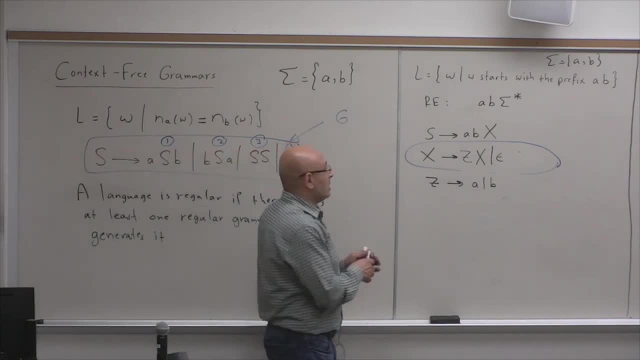 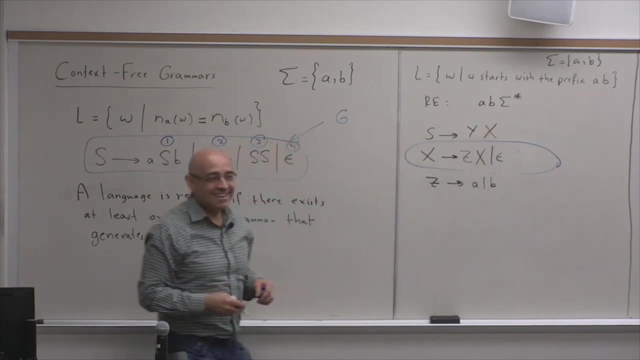 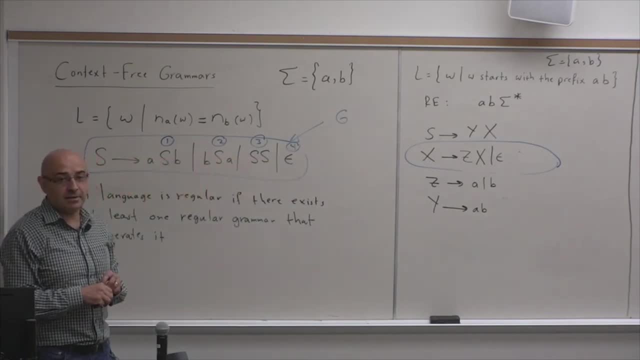 OK, Thank you, OK, Thank you, Thank you. Yeah, Thank you, Thank you, Thank you if you can find at least one regular grammar that generates it. Okay, Finally, any questions? So this relation between you know grammars? 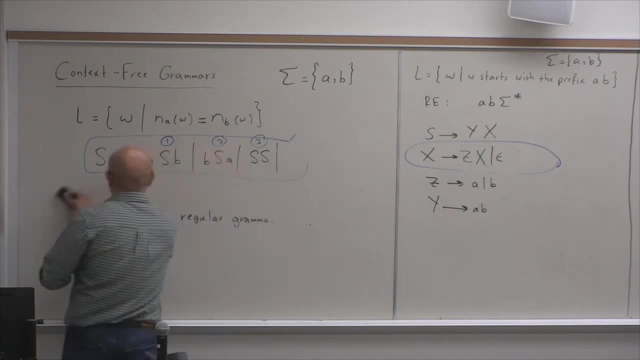 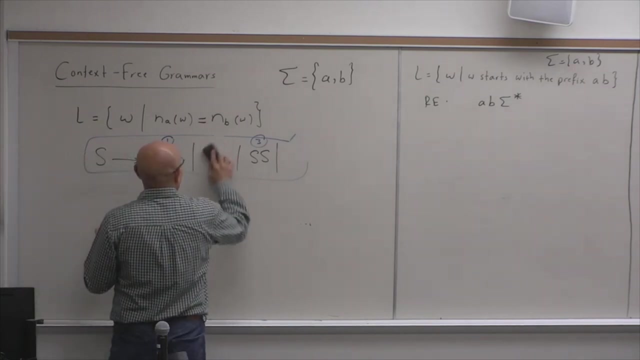 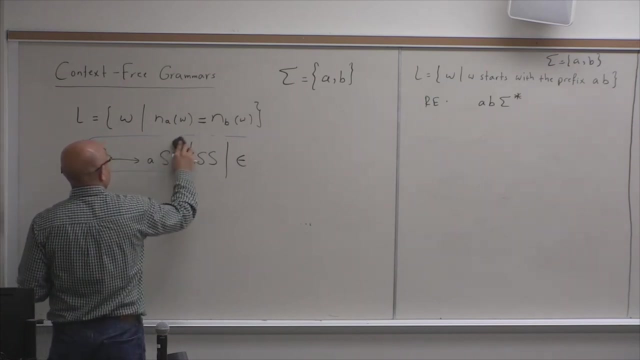 and finite automata, I think is interesting. In fact, I don't need to erase this because I will not have the time to use this. So what about this grammar? So what does this generate? So what can you say about the strings that are generated? 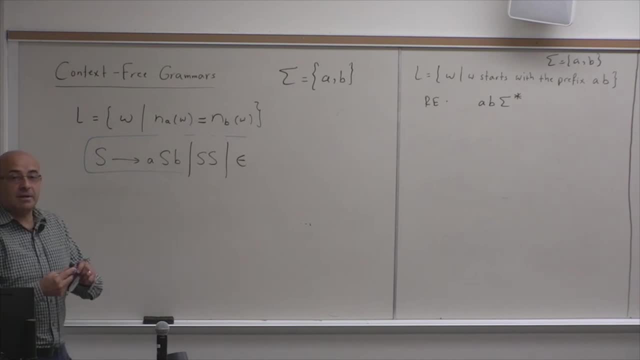 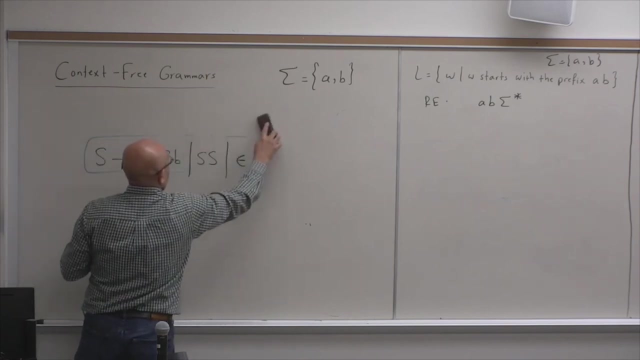 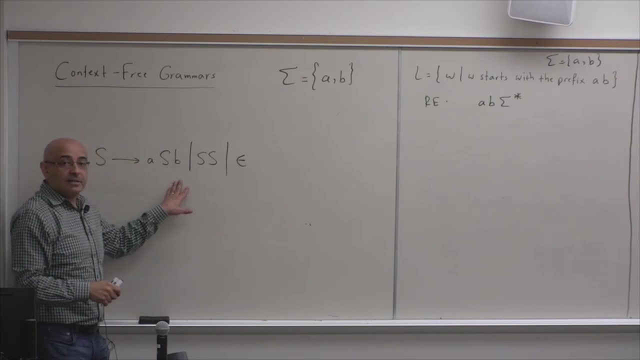 Of course, the strings that are generated by this grammar. this language is going to be a sub-language of the language of strings that have an equal number of A's and B's. So this language here. so this is no longer this. So this language, you know, the set of strings generated here is a subset. 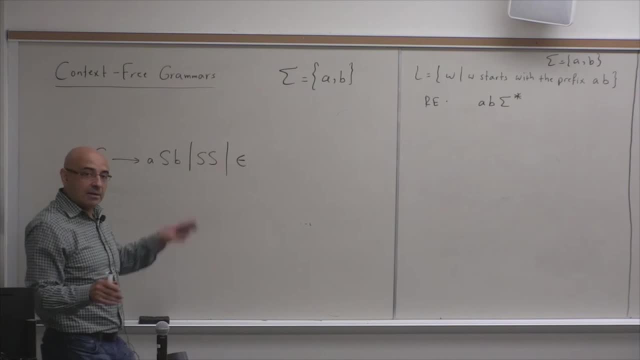 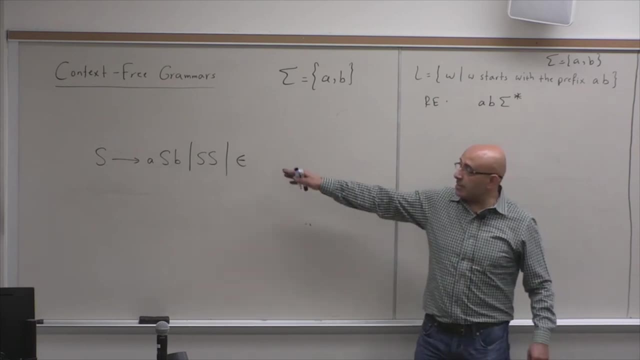 of the set of strings that are generated by the previous grammar that we had before with the other production. you know the language of equal A's and B's, So this is a subset of it. So, in addition to having an equal number of A's and B's, 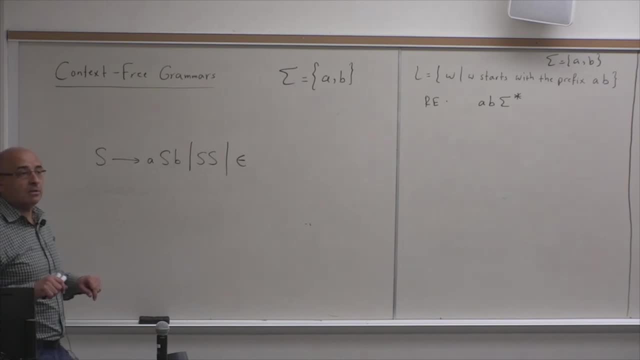 what can you say about the string that gets generated by this language? Okay, it starts with an A and ends with a B, And it's more than that. In fact, if you replace A and B, if you replace sigma with this, 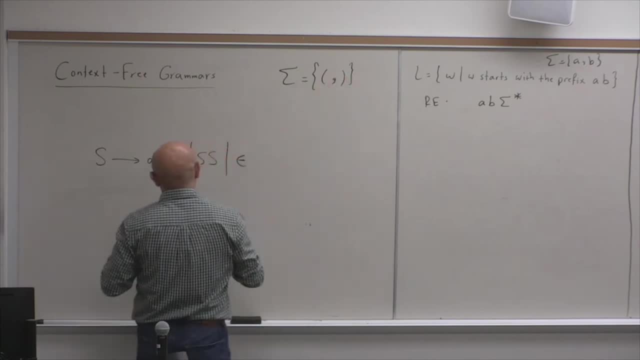 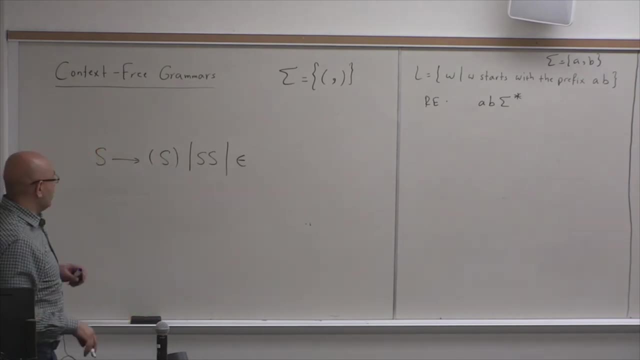 with these two symbols. okay, so what will this generate? Balance, Hmm, Balance. Yeah, exactly, Balance parentheses. It will generate the set of all balanced sequences of parentheses. So L is going to be W, such that W is a balanced or a sequence. 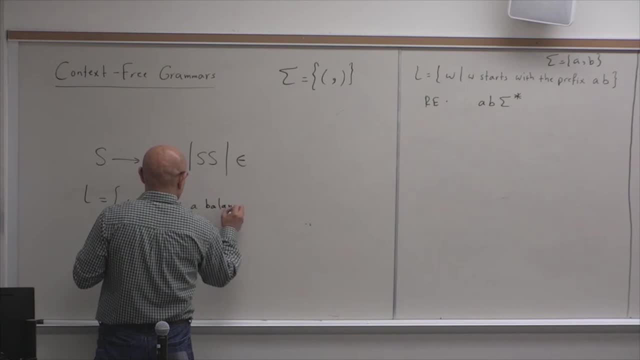 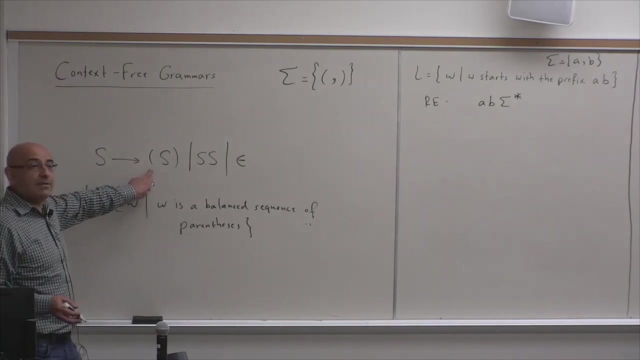 oh, in fact, a balanced sequence of parentheses, So it's going to be W. So here you know. basically it's saying that you cannot have. you cannot open, have open parentheses without having closed. So everything that you open, you must close it. 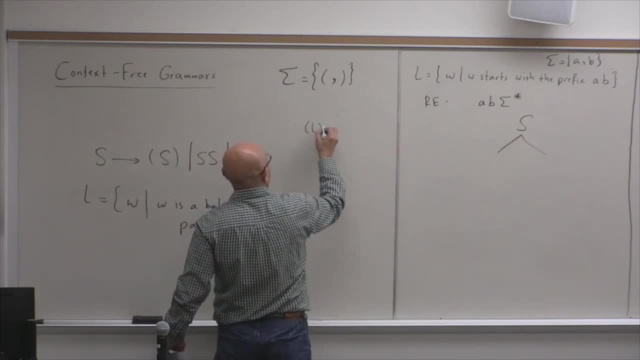 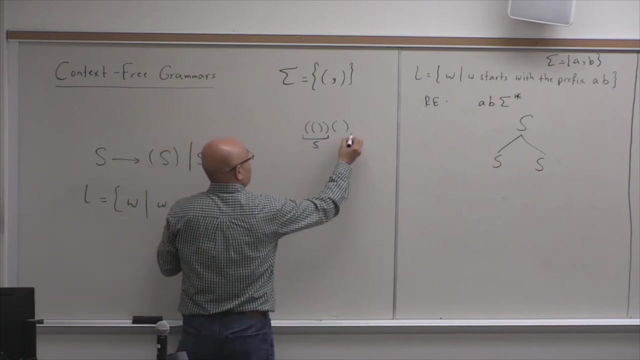 So here you know I can derive, so let's try to derive this. Trying to derive this, Okay, Okay, Okay, So I can derive this. I have an S and an S, And what's the first S? This is the first S, And this is the second S, And the first S is going.